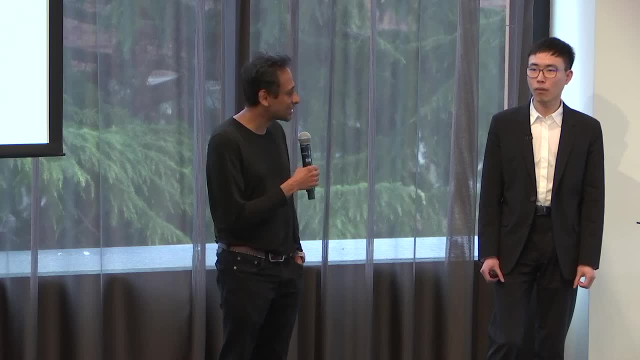 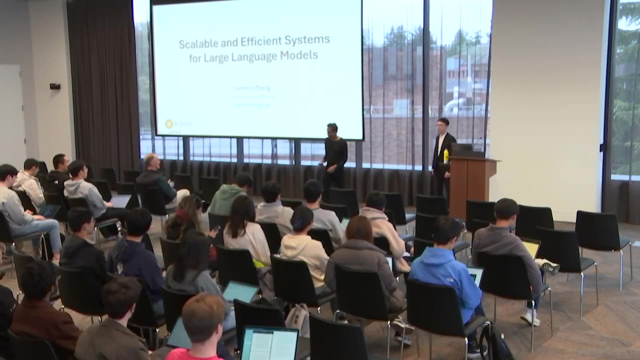 out of Leonman and his colleagues, And he's here to tell us more about those pieces of work, So take it away, Okay. Yeah, Thanks, Alvar, for Thank you for the introduction and thank you so much for having me here. I'm very excited. 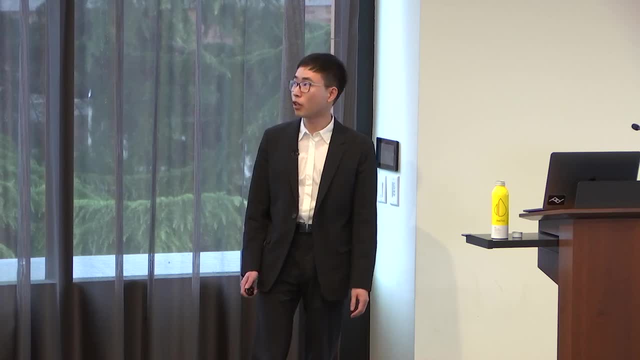 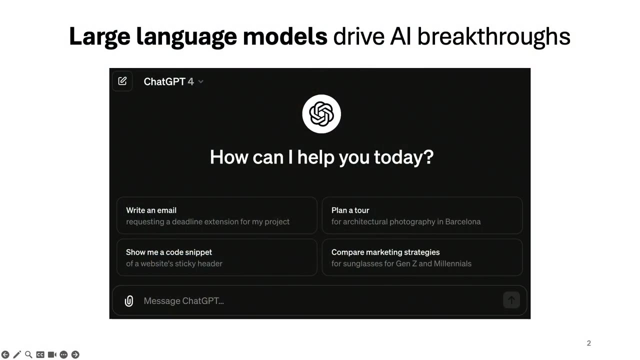 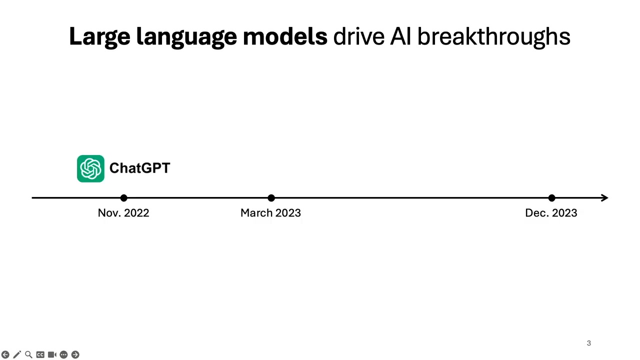 to introduce my work on scalable and efficient systems for large-language models. So large-language models have been driving the recent breakthroughs in AI. Most likely many of us have interacted with these models through OpenAI's CharterGPT, a very smart charter system. So CharterGPT. 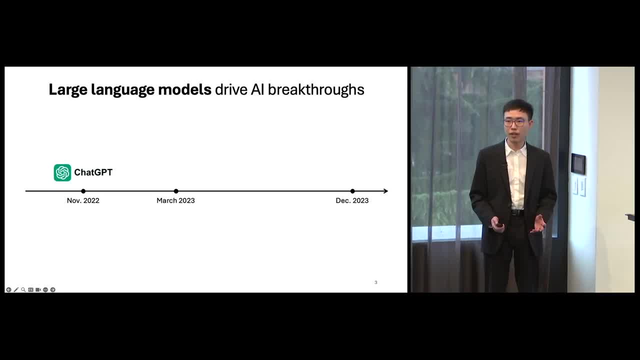 was released about one year ago. In just one year, we have witnessed not only the emergence of CharterGPT, but also the emergence of OpenAI, Thank you. And now there's also a surge of many other powerful models, like Anthropia Cloud. 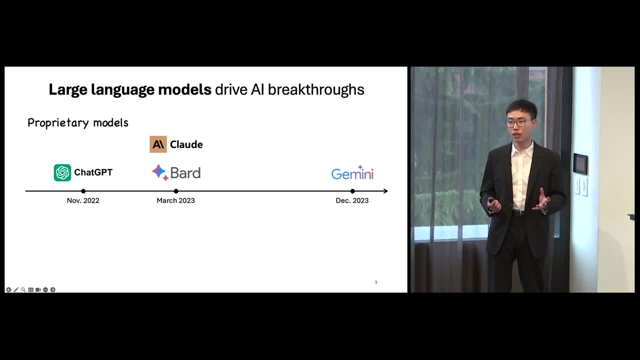 Google, Spark and Gemini. However, this model remains closed-thrust. This means you cannot see their model ways or model architectures, So it limits our ability to fully understand and build upon them. On the other hand, the open-source landscape has also seen significant 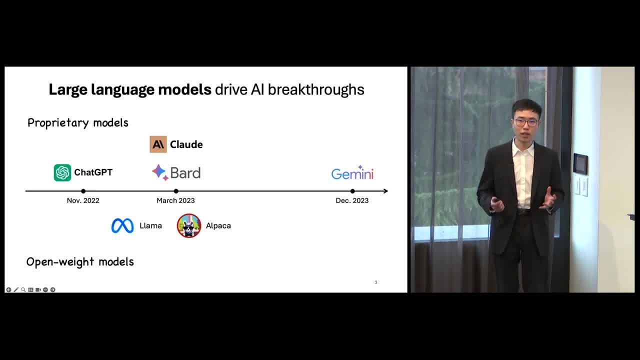 progress, starting with Meta-Lava. now we have the Al-Paqa and the Multi-Model-Lava. Fortunately, I have had the opportunity to contribute to the development of these models, to this exciting open-source movement, by leading the development of Vicunia. 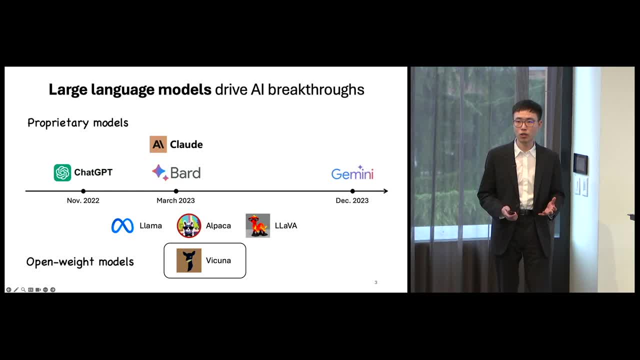 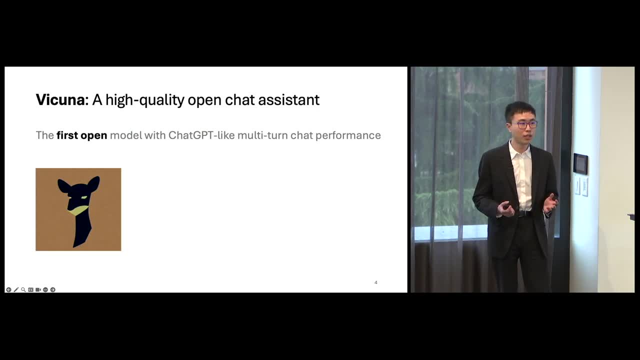 which is also one of the most popular open large-language models. So our model Vicunia, is a high-quality open chat assistant. It's very similar to ChatGPT and it has been widely recognized as the first open model to achieve. 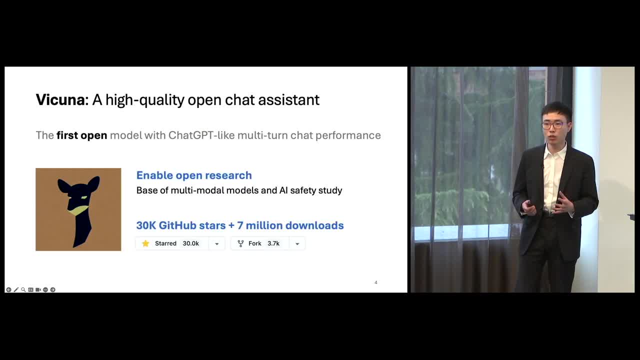 ChatGPT-like multi-turn chatting performance And, thanks to its openness, people can customize it, so it enables frontier research in multiple areas, such as multimodality and AI safety. Since its release, it has received over 30,000 GitHub stars and 7 million downloads. 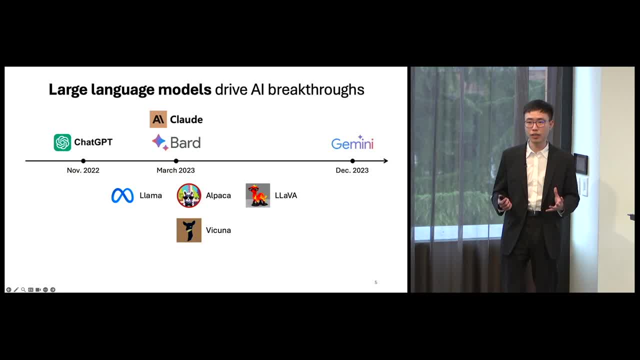 Well, Vicunia is just one example of the recent excitement in AI. Let's go back to this timeline. The achievements of the last year are remarkable, but it's crucial to recognize that they stand on the shoulders of many years of research. 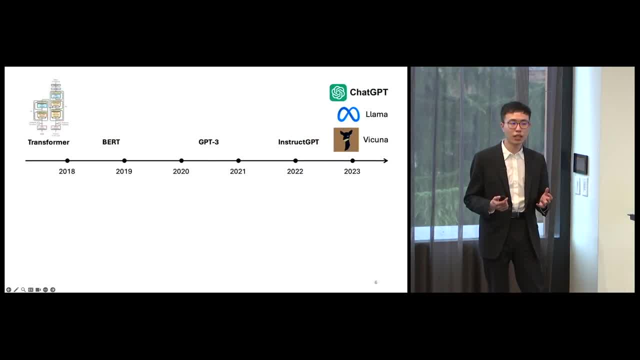 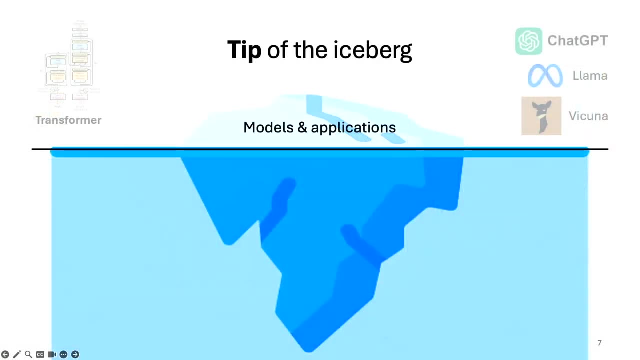 including the transformer architecture and earlier AI explorations from decades ago. Moreover, I want to tell you another significant body of work that has made this achievement possible, And if we take this into account, then the models and applications we see here are just tip of the iceberg. 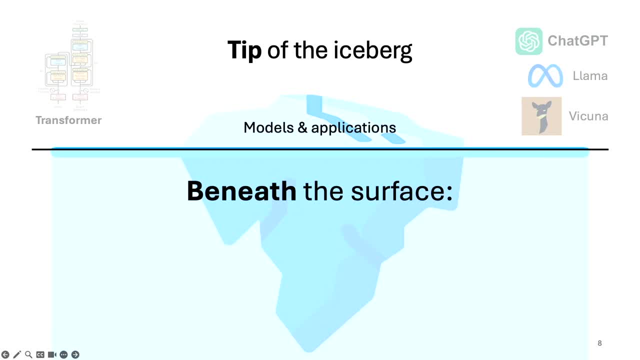 Beneath the surface lies some foundational bedrocks. This includes the hardware for performing accelerated tensor computation, the compilers for connecting the hardware to software algorithms and the large-scale data centers for running distributed data. This includes the training and the serving and high-quality data for feeding the knowledge into the models. 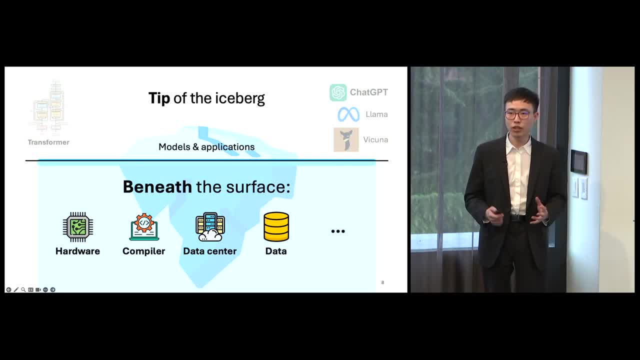 So these underlying elements are as important and challenging as the machine learning algorithms themselves, And the research here is just about how to connect these elements together to build solid foundation systems for large models. So I would like to call all these systems for large models as Large Model Systems, or LMC's for short. 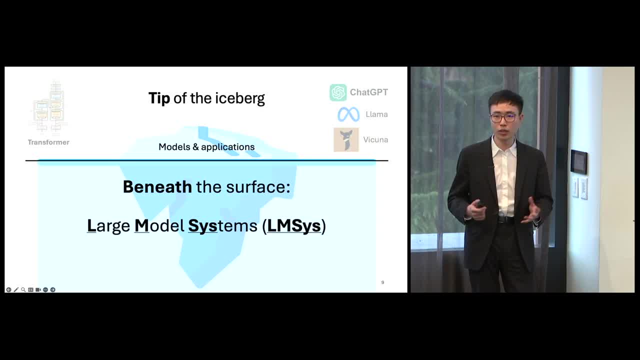 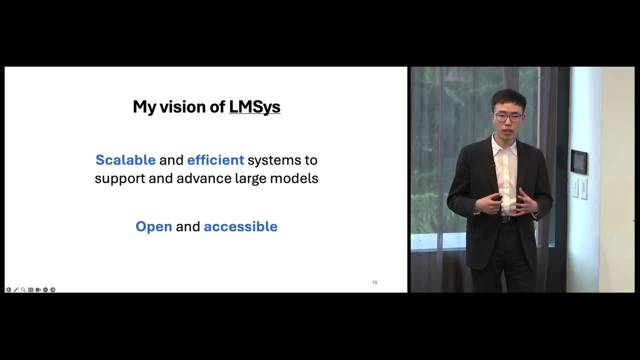 And my research is about designing and building these systems. So my vision for LMC's is to build scalable and efficient systems to not only support but also advance the development of large models. On the other hand, as I said, I place a high priority on openness and accessibility. 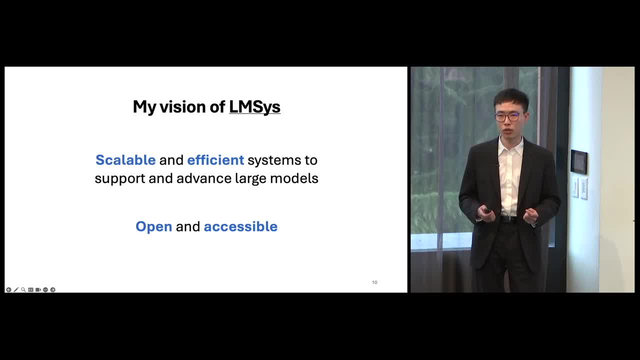 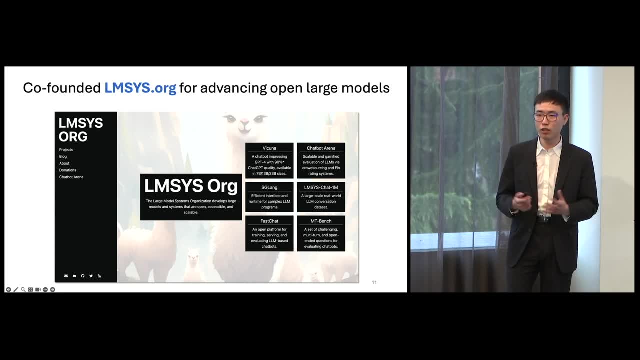 enabling everyone to contribute to the development and benefit from it. So, guided by this vision, I co-founded LMC'sorg earlier last year. It's a multi-university open-source research collaboration And it turns out we have made a huge impact on the open model space by developing high-performance systems, high-quality models and evaluation methods. 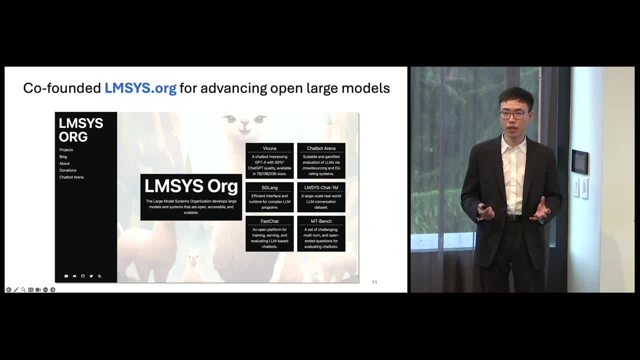 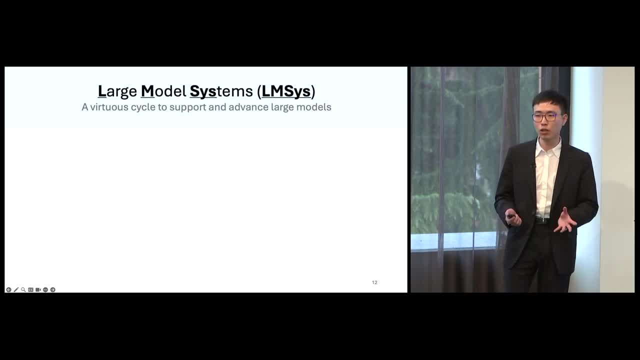 So in this talk, I will share this line of research and share the lessons we learned. So, to organize the project, I will draw a full lifecycle model and I will present the associated challenges and introduce our solution. So, as I said, I will connect these elements together as a virtual site. 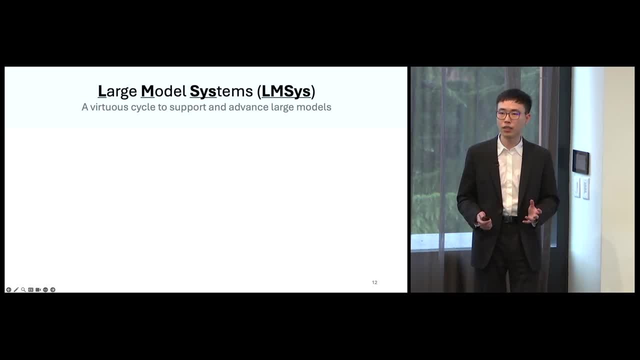 So to organize the project, I will connect these elements together as a virtual site To support and advance large models. So to build a good model, we start with training For these large models. we aim to train models with billions of parameters on the internet-scale data. 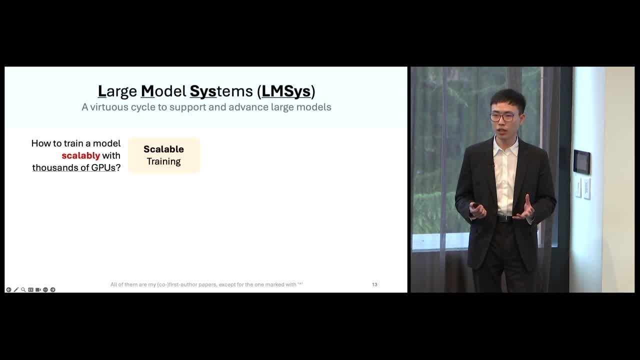 So the challenge here is how to train a model scalably, potentially with thousands of GPUs. So to overcome this, I built a distributed training system called ALPHA and some memory-efficient training algorithms like ACT-N. So the goal here is to facilitate the training of models that are 10x larger. 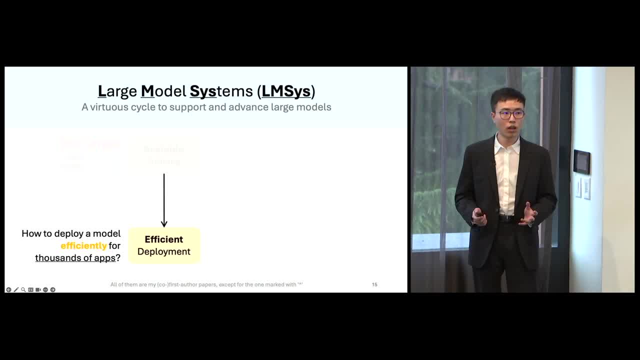 After training a good model, we want to deploy it. So because these models are so large, even using them for inference requires significant computational and memory resources. So the challenge here is how to deploy a model efficiently. On this side I made contributions by developing some high-performance, fast inference engines. 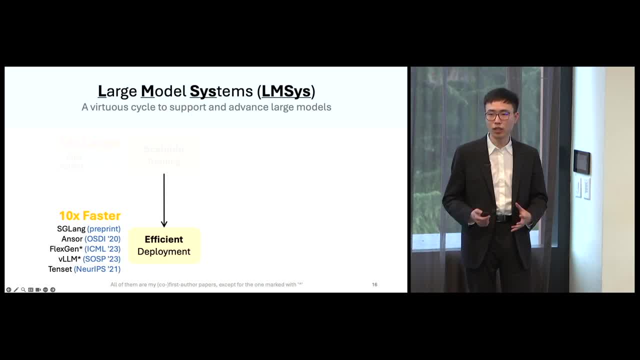 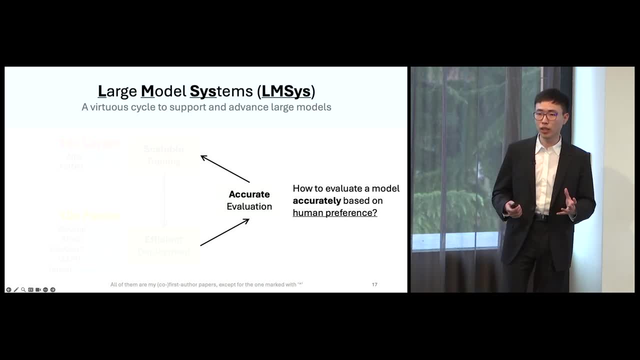 like SGLAN, FlexGen and VRM, with the goal of making inference run 10x faster. So, after deploying a good model, the next step is to collect some feedback of these models. This involves evaluating the quality of these models. 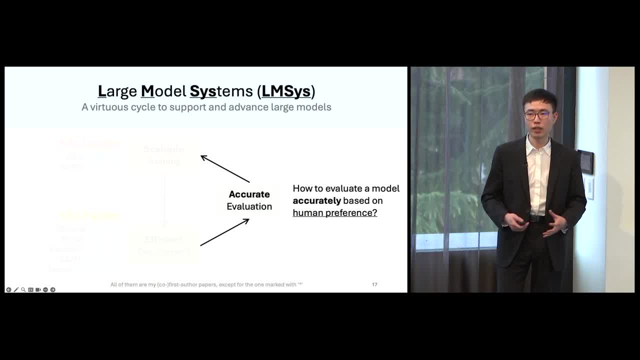 which can also help us with the building and training of next-generation models. So, on this side, the challenge is: how do you accurately evaluate a model quality, particularly in terms of human preference, because these models are often designed to interact with humans. 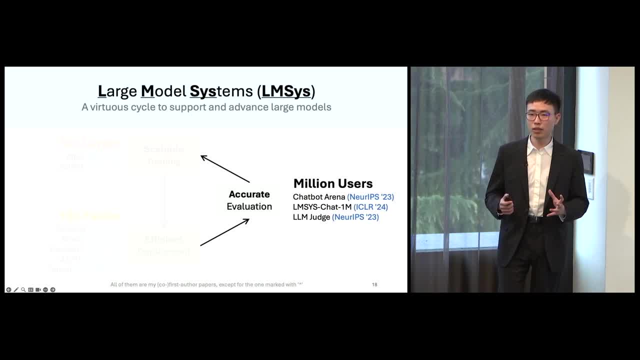 On this side, I made contributions by developing some innovative evaluation methods, such as the crowdsourced platform Chatbot Arena, which is now gathering accurate, fresh, diverse human feedback from over 1 million crowdsourced users. So, basically, I worked across the entire lifecycle of the model. 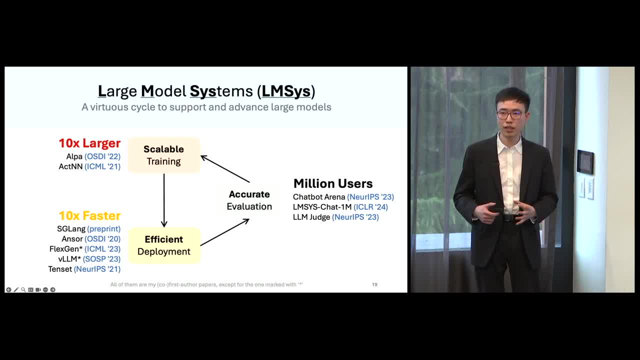 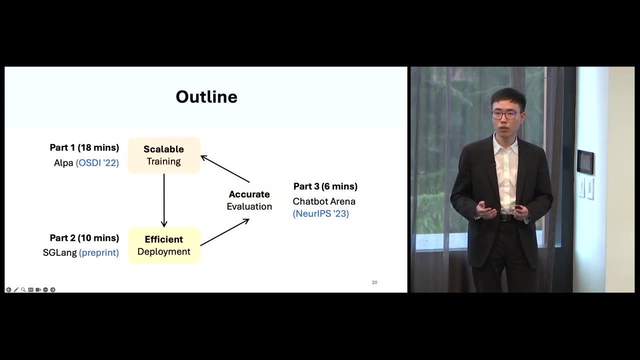 developing solutions from top to bottom, and these elements mutually supported each other and enabled more people to conduct research and build applications on top of them. On this talk, I will focus on several projects. In the first part, I will introduce ALPHA for automatic scalable training. 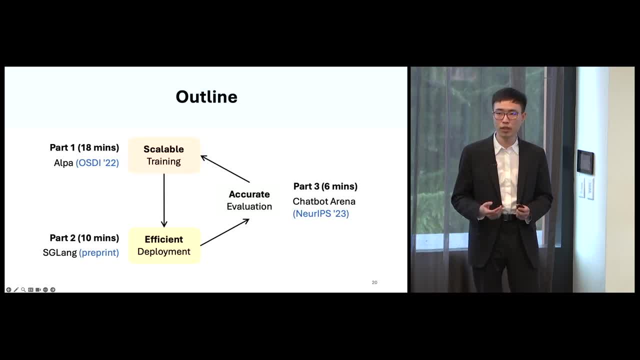 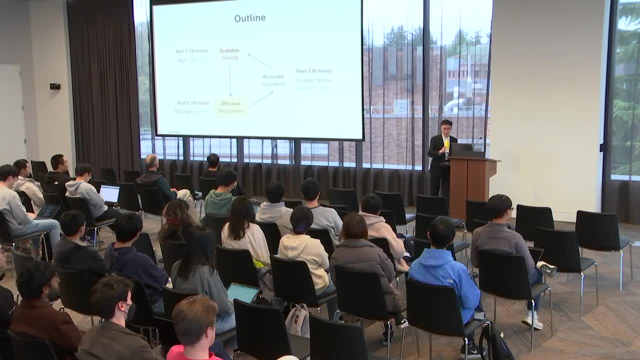 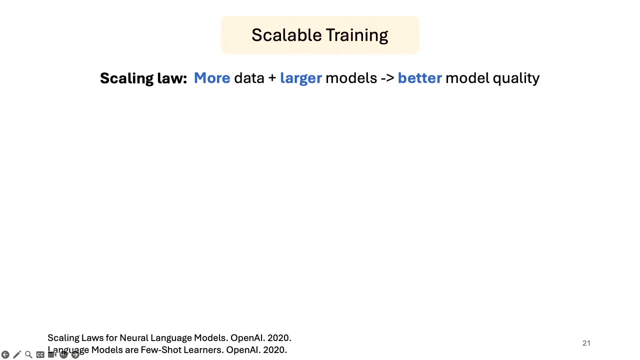 and then I will discuss SGLang for efficient deployment Towards the end. I will briefly touch upon our model evaluation efforts and outline future research directions. Okay, we can start with the training part. When training large-language models, there is a principle often referred to as the scaling law. 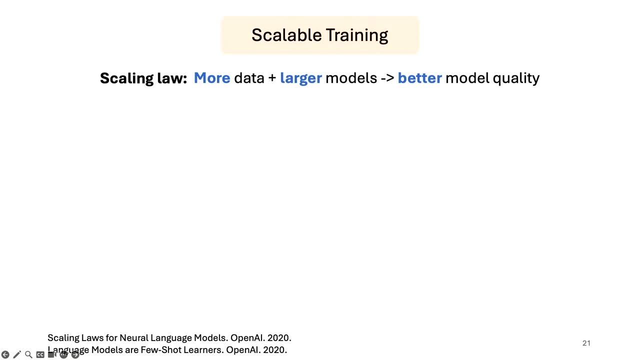 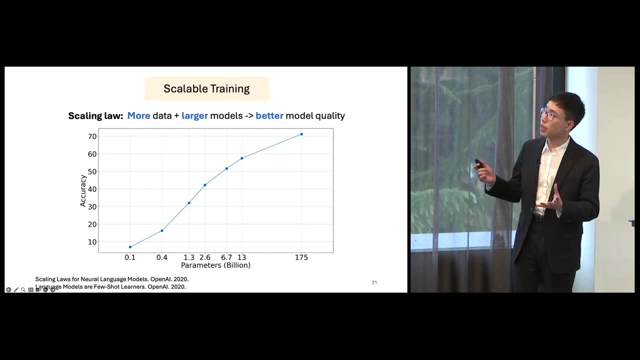 It suggests that to improve the model quality, one needs to scale both the dataset size and model size together. Essentially, this principle can be illustrated by the following figure from the GPT-3 paper, where the x-axis is the model size in terms of number of parameters. 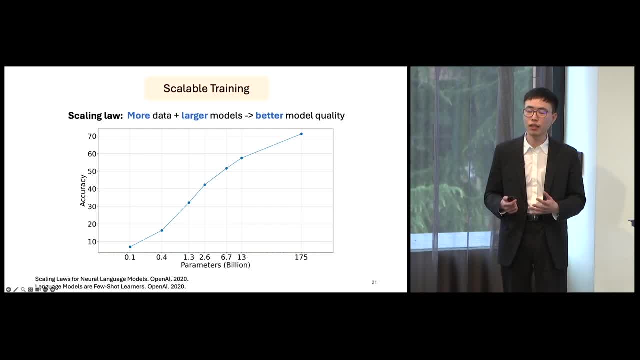 and the y-axis is the accuracy on a question answering task. As you can see, increasing the model size can greatly increase the accuracy. so this principle has guided OpenAI in scaling their models from GPT-1, GPT-2, GPT-3,. 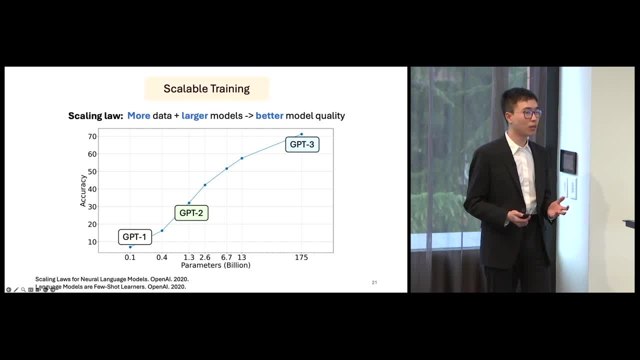 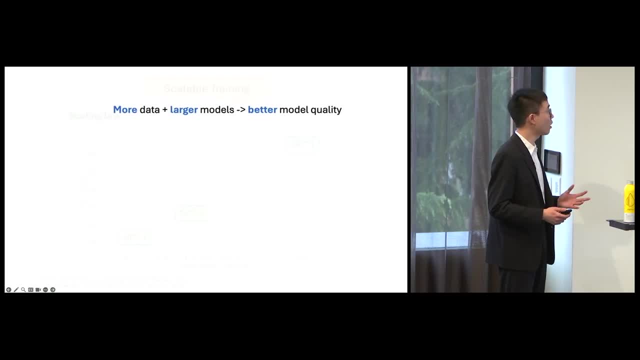 all the way to GPT-4, leading to AI breakthroughs. So now we know the secrets of OpenAI, then how can we implement that? So in this talk I will focus on the system perspective. From the system side, handling more data in the larger models. 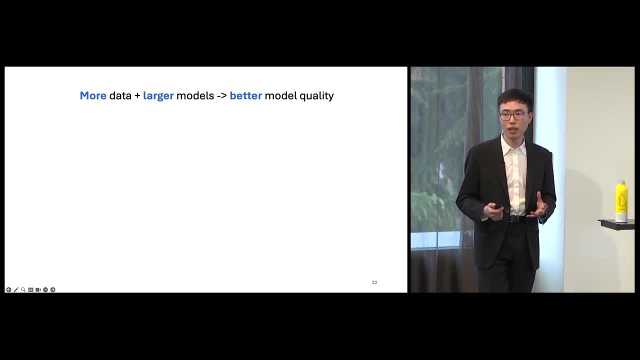 means we need to leverage parallel computing and go distributed. So for more data it's actually easier. The approach is called data parallelism. If we have two GPUs and our model is small enough to fit into a single GPU, then we can simply duplicate the model across both GPUs. 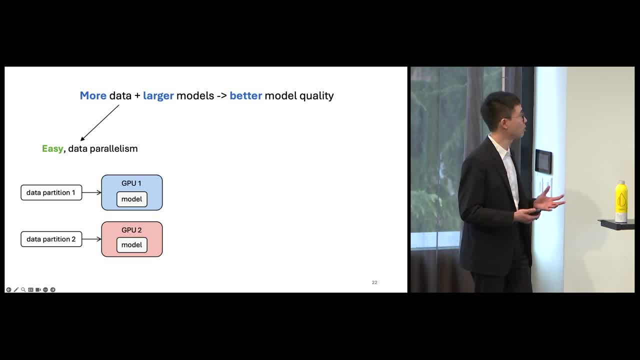 and feed different partitions of the data to different GPUs, because the dataset is just a long list of files, so partitioning it is easier. However, when we are dealing with large models, that's where the real challenge begins. Take GPT-3, for example. 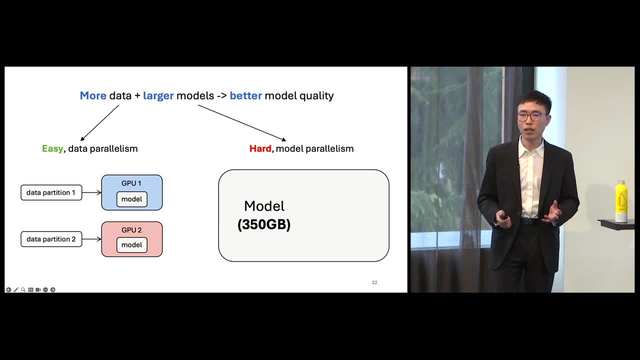 It's a massive model with over 300 GB, far exceeding the memory capacity of a typical GPU. So training such giant models would require partitioning the model itself, and because the model is a complicated computational graph, so partitioning it is much harder. 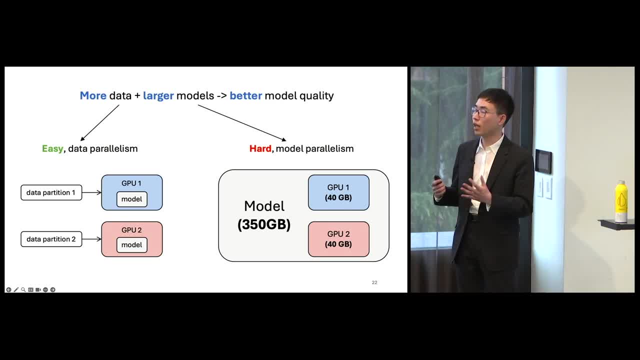 And in this talk we will focus on the second, harder part, model parallelism, and I will show you how we can apply some optimization techniques, compiler techniques, to make model parallelism much easier so you can easily train some large models. 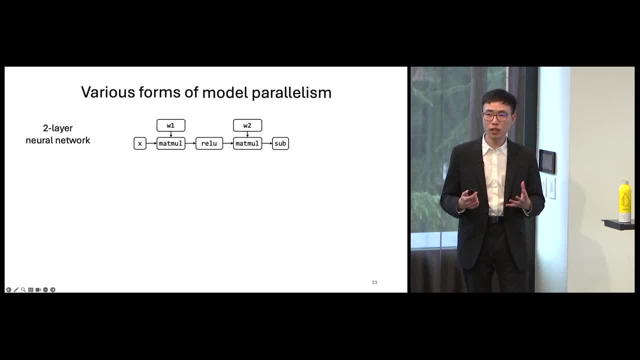 Okay, before we start, let me introduce some basics to the concept of model parallelism with some simple, concrete examples. We can start from a two-layer neural network. We can view a network as a computational graph, and here I draw the forward propagation part of the graph. 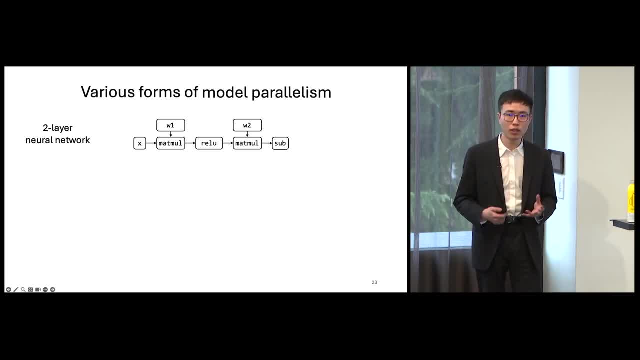 It begins with an input x and then followed by some operators such as matrix multiplication and ReLU activation, And w1 and w2. here are two weight matrices. So if we have two GPUs, how can we parallelize the graph across two GPUs? 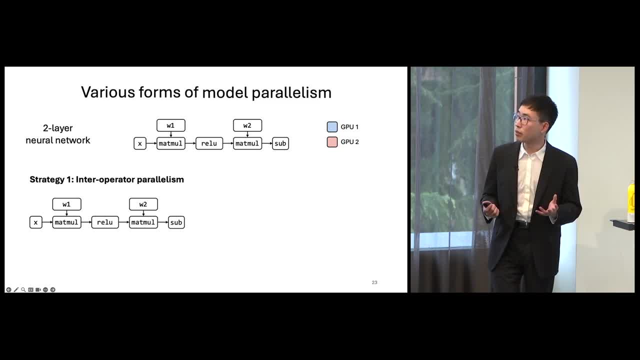 The first approach is called inter-operator parallelism, because we want to leverage parallelism across different operators And for the graph, we can cut the graph in the middle and put the first part on GPU 1 and the second part on GPU 2.. 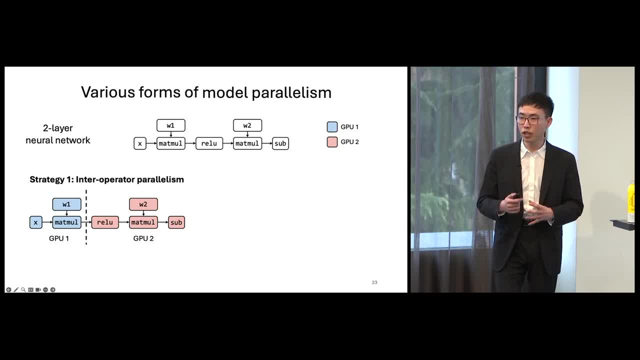 So this cut is actually not too bad because the communication across the cut is small. However, due to data dependency, the second device cannot always be busy because it has to wait for the first device to generate its input, leading to some idle time. 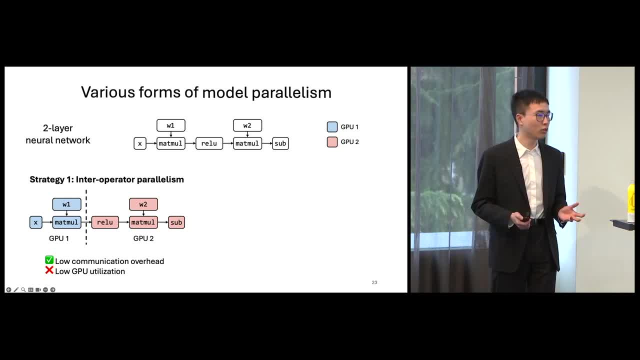 And although this can be alleviated through pipelining, it still results in some device idle time due to the dependency between forward propagation and backward propagation. Now, if we want all devices to always be busy, what should we do? So here comes the second approach. 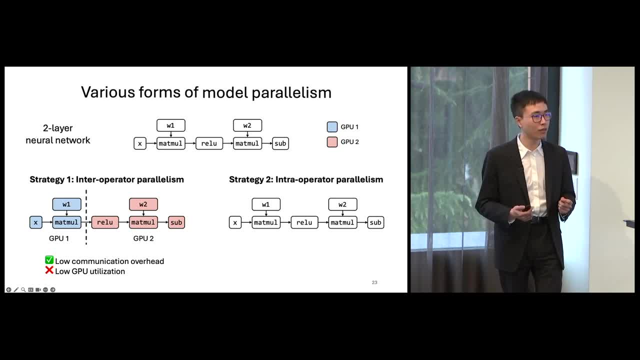 Instead of partitioning at the graph level, we can partition at the operator level, allowing different devices to work on different regions of the same operator, And in this way we can keep all devices busy, but it leads to more frequent communication, as devices have to synchronize after one operator. 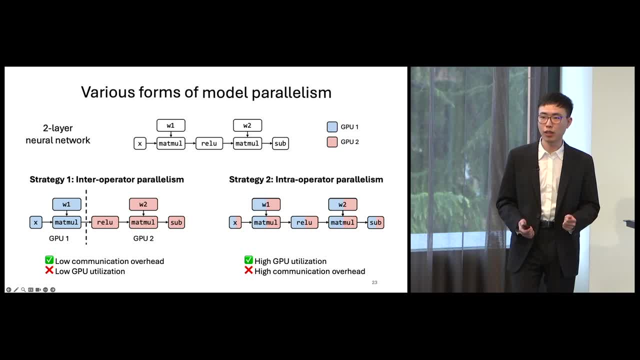 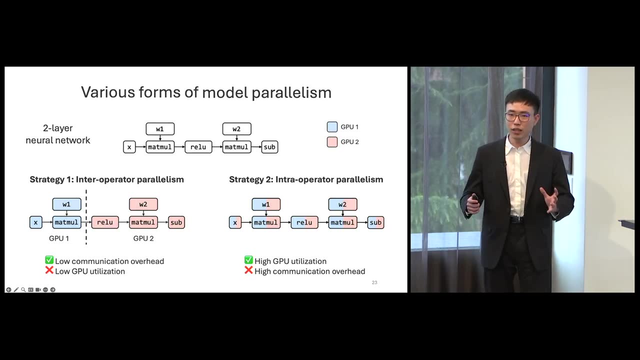 if the next operator cannot preserve the previous partition. So, basically, this page shows two basic patterns of partitioning a graph and there are trade-offs between them in terms of GPU utilization and communication overhead. Under this classification, there are also more variants. 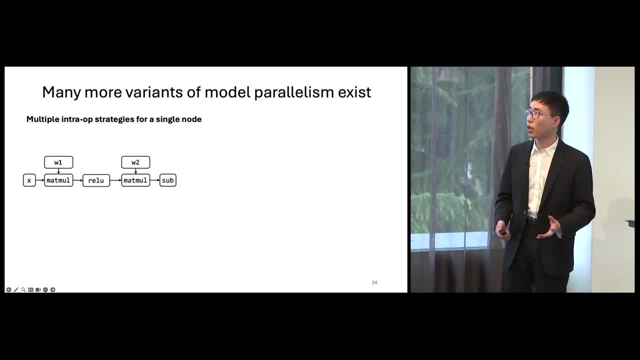 which makes the problem more complicated. For example, multiple strategies exist for a single node, For example for matrices. we can partition it along rows or by columns, or some we can entirely replicate them. So for higher dimensional tensors, the range of possible partition strategies also expands. 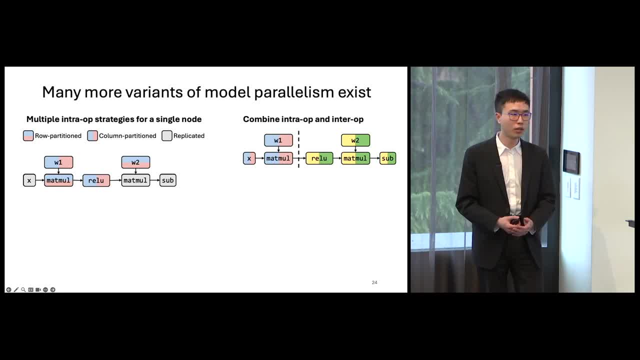 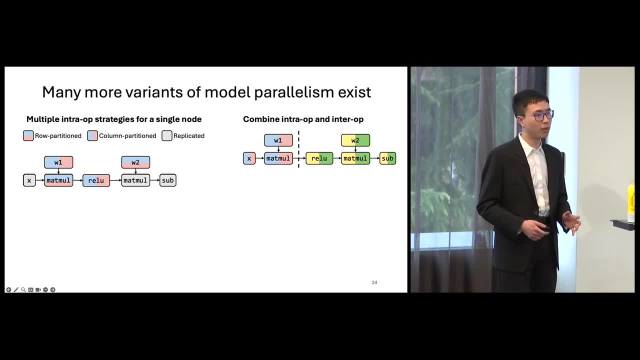 And we can also combine inter- and intra-operator parallelism. So in this case we can cut a graph as two parts for inter-operator parallelism, then within each subgraph we apply intra-operator parallelism And we can show: this combination is very useful. 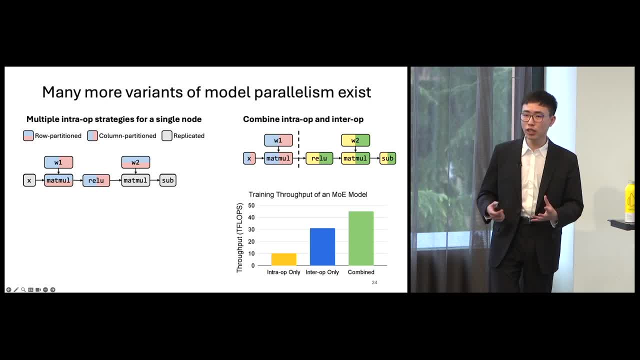 when we are training a MOE mixture of expert model. Only when we combine these two kinds of parallelism we can get the best performance. And showing this figure, the combined bar gets the highest training throughput. And there are also some other scheduling techniques. 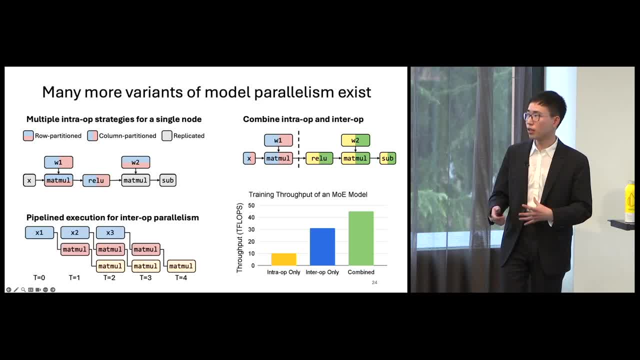 called pipeline parallelism, For example. in this case we can place different layers on different devices and let them work on different input batteries together in a pipeline fashion. So this can resolve the dependency and increase device utilization. Okay, so all these kinds of partition strategies? 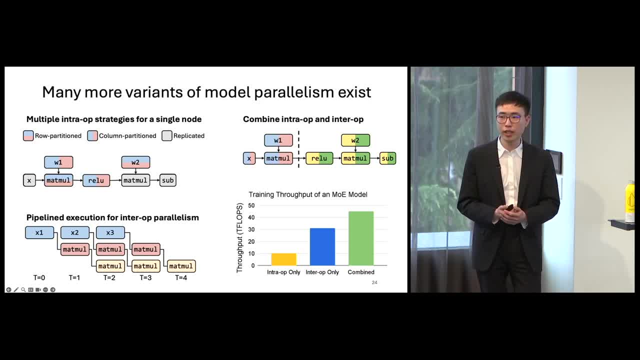 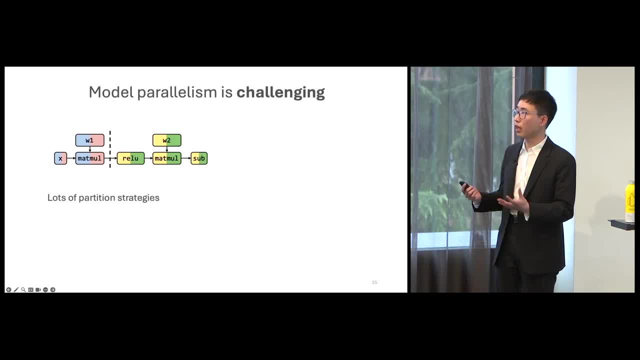 and scheduling techniques create a very large search space, especially for larger graphs with thousands of nodes, which makes the problem very challenging. And to briefly summarize: on the left side we have lots of possible partition strategies and on the right side we have lots of GPU. 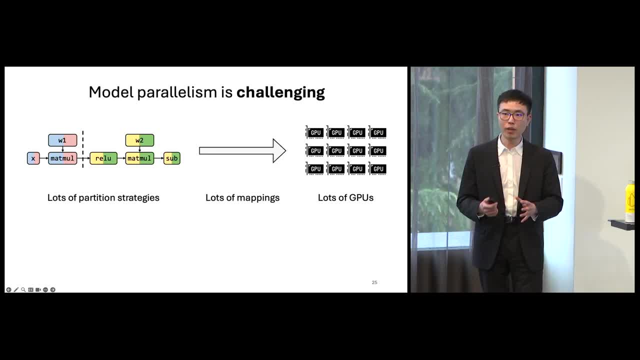 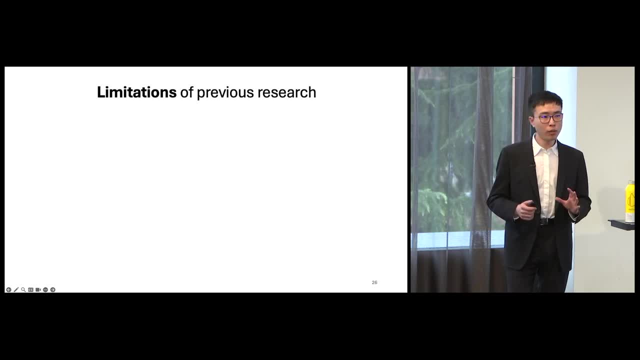 And in the middle there are lots of possible mappings. So these elements create an exponential search space, makes the problem very challenging. Because the problem is both challenging and critical, it has attracted attention for years At NVIDIA. it took four years of engineering. 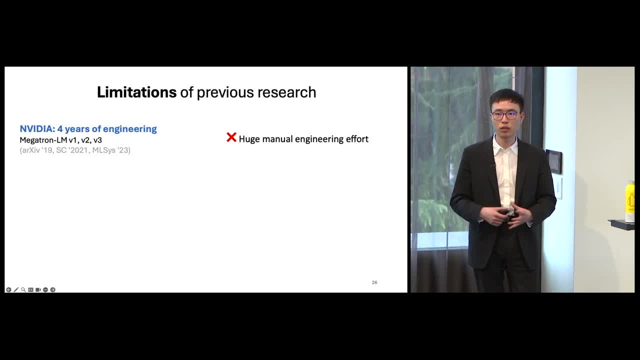 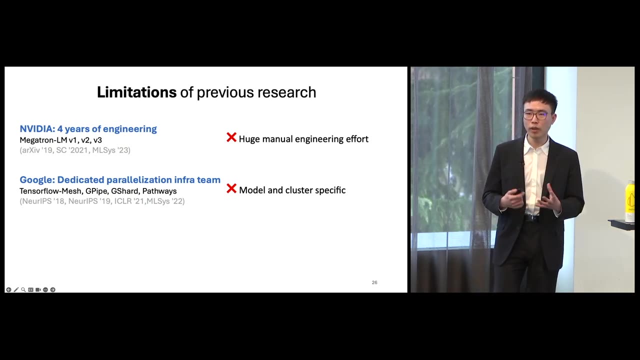 for them to develop a distributed training system called Megatron RM. It incorporates several manually designed parallelization techniques. As you can see, it requires a huge amount of human effort. Similarly, at Google, dedicated teams are required to parallelize the models for their researchers. 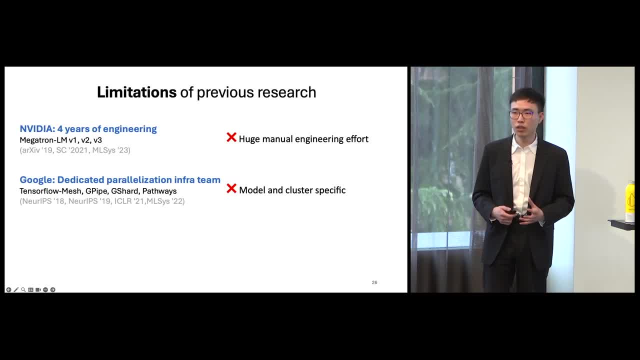 So their manual strategies are often specific to certain model architecture or clusters, So they have to redo it every time for a new model architecture In academia, although there are some autoparallelization works. however, they struggle to run large models because they only handle 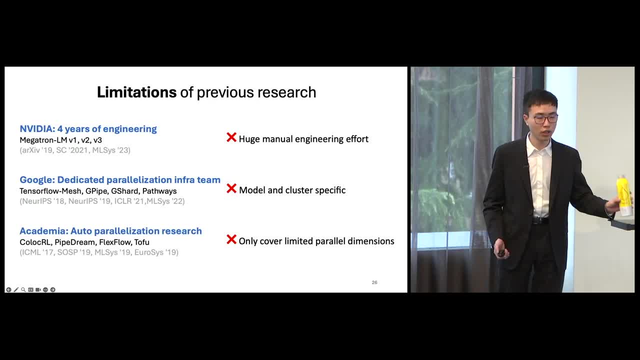 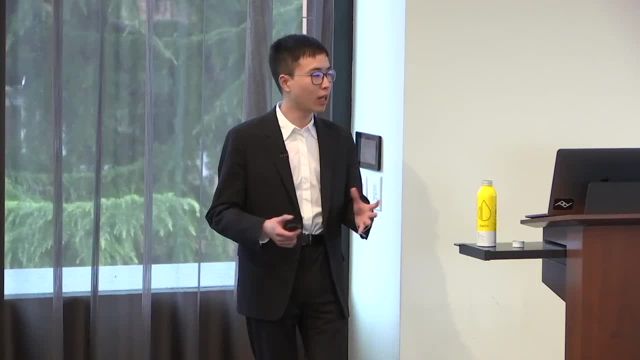 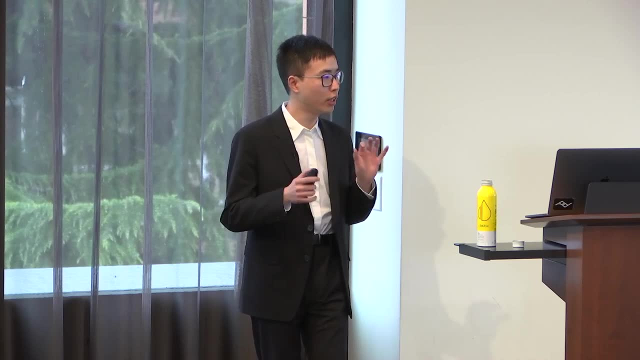 a limited number of parallel dimensions and they don't have an efficient search algorithm. Okay, so I will go through some details and use a table to compare several existing systems. I will categorize existing techniques under the classification of inter- and intra-operative parallelism. 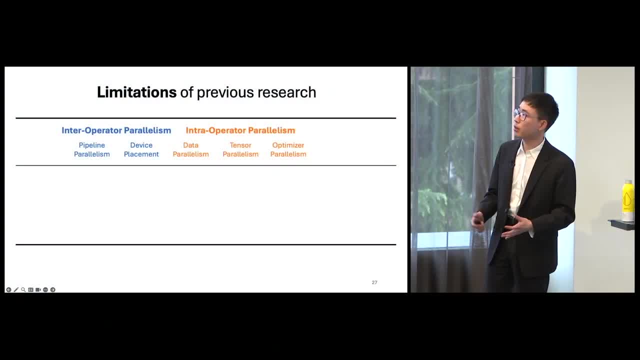 So common techniques include pipeline parallelism, device placement, data parallelism, tensor parallelism and optimized parallelism. You probably don't need to fully understand these systems. They are essentially just different combinations of the inter- and intra-operative parallelism I just mentioned to you. 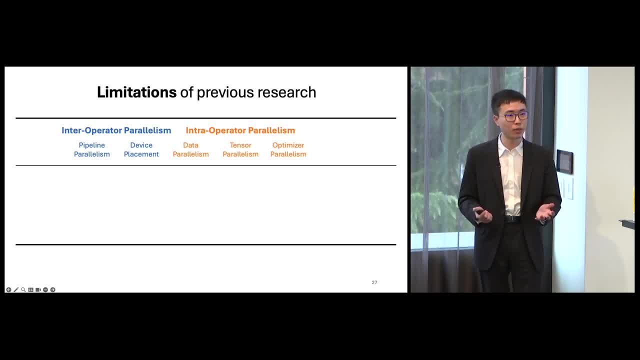 People just give them different names because they don't have a unified representation. So in Megatron LM- the system from NVIDIA- it supports some of the most critical parallelization techniques. However, it's a manual system so it can take weeks to months. 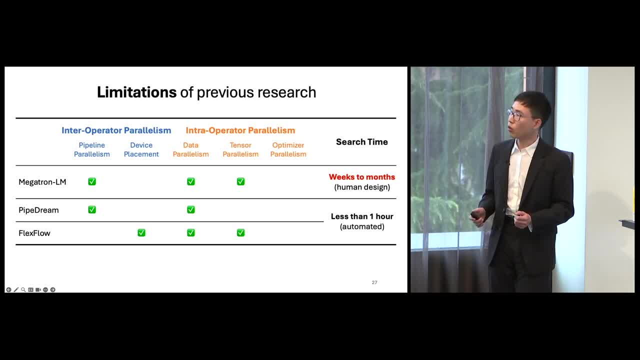 for it to adapt to a new architecture. On the other side, some autoparallelization systems like NVIDIA and FlexFlow. they can quickly generate a parallelization strategy for a new model architecture within one hour of search time. However, as you can see in this table, 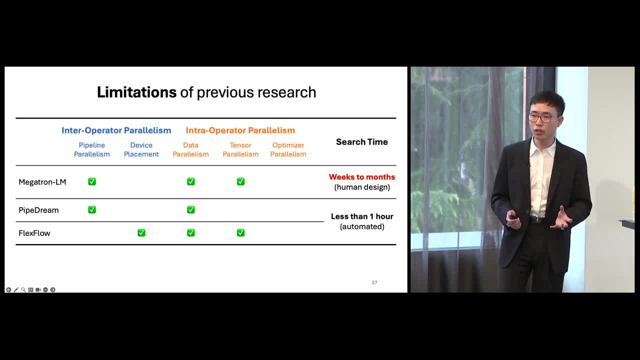 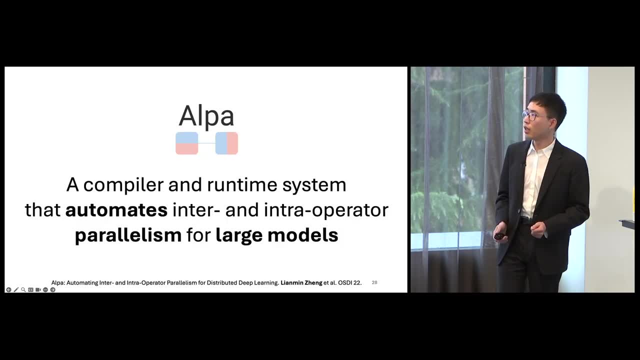 none of the existing systems can cover all the parallel dimensions, leading to some suboptimal performance when training some models. In this project, our goal is to tackle this challenge by building a new system called ELPA. It serves as both a compiler and a runtime system. 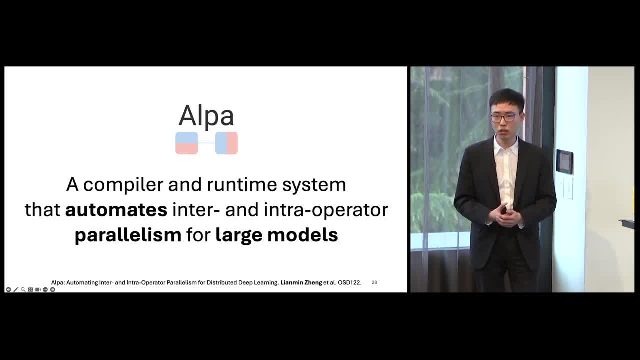 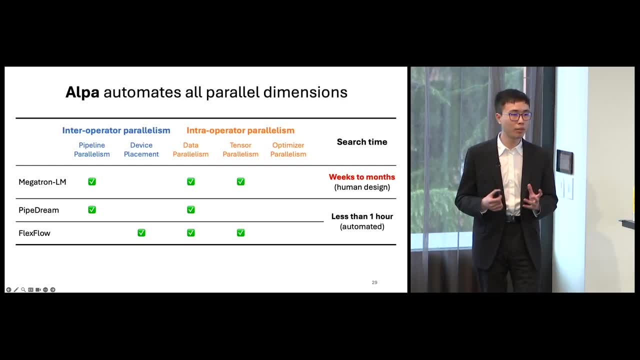 that tries to unify and automate all these different combinations of inter- and intraoperabilism. So let's bring back this comparison table and see how ELPA compares against the existing projects. So these are the existing projects and this is what ELPA looks like. 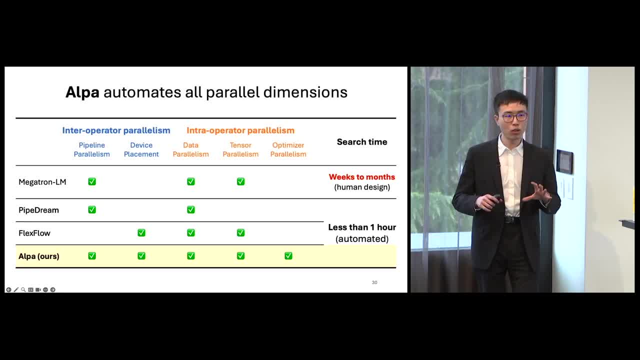 in this table. As you can see, ELPA is able to cover all these possible parallel dimensions, So ELPA seems to be the solution that captures all the benefits. How do we make it possible? Because model parallelism is a complicated search problem. 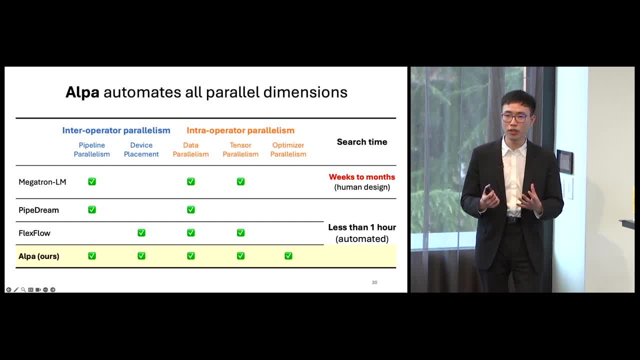 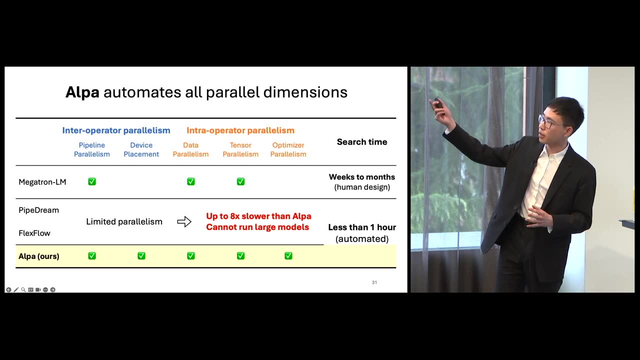 So we ask: can we leverage some structure of the search space to make the search easier? Interestingly, thanks to the structure of the computational graph, there are some things that we can utilize. So we find okay. so like, yeah, like this: 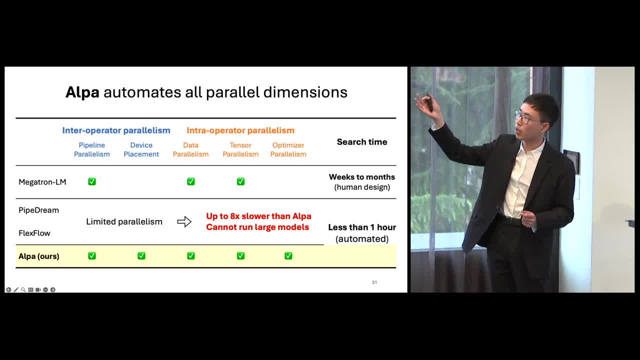 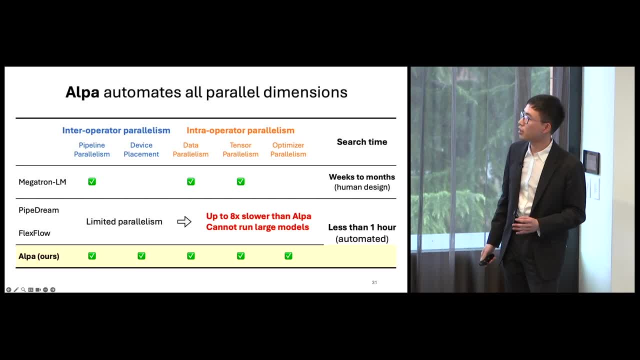 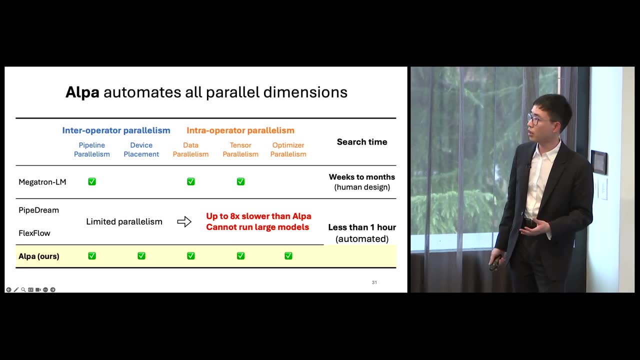 it shows like ELPA. compared to prior automatic system. ELPA, like also has some significant advantages. I probably skipped the slides, So like, because in ELPA we think this is a search problem. we like how do we make the search easier? 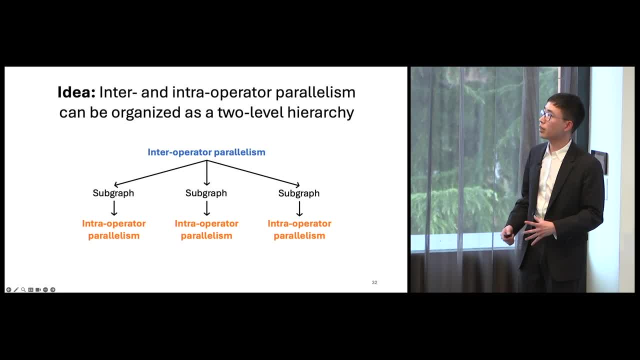 So actually we find we can organize the inter- and intraoperabilism as a two-level hierarchy. So at the top level we first search for inter-operabilism. This will give us several smaller subgraphs, And then for each subgraph, 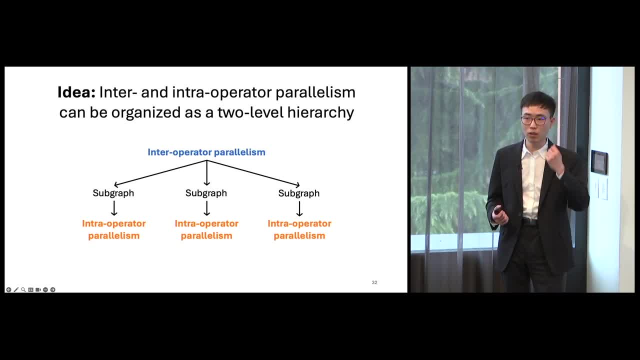 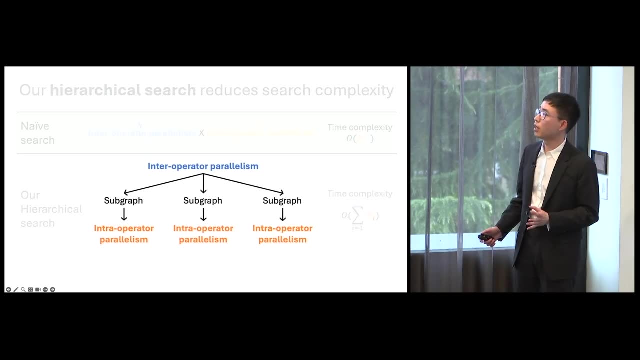 we search for the intraoperabilism within each subgraph. So by doing this we can greatly reduce the search complexity And it also allows us to solve the problem layer by layer. So I will compare this against a naive approach of search. 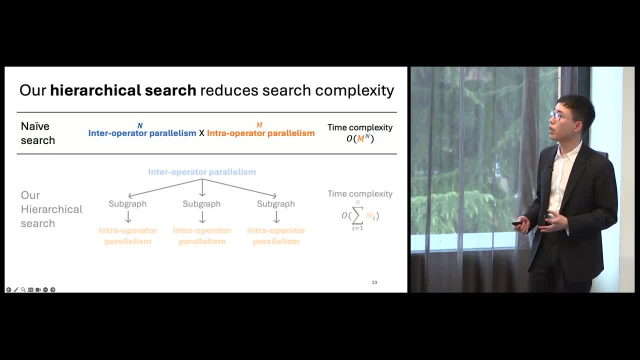 Naively, if we want to search for all the combinations of inter- and intraoperabilism, then the complexity is roughly the number of possible intraoperabilism to the power of the number of possible interoperabilism. So this is a very large space. 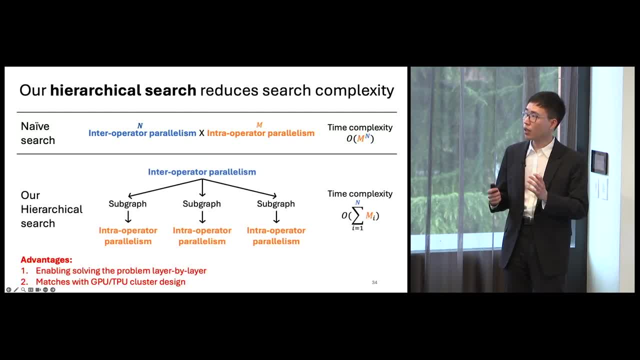 and very hard to search through. In our hierarchical way of search, as I said, we first search for higher-level probabilism and then go to the granular level to search for lower-level probabilism. You may think this is an approximation of the original search space. 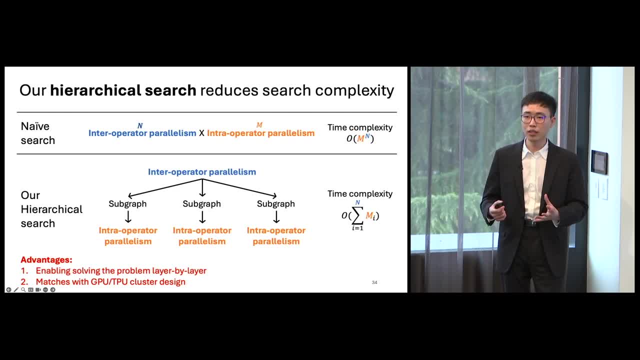 but we empirically show that this approximation almost does not harm the solution quality. This is because in a typical neural network the communication between different subgraphs are usually very small. So this approximation does not harm the solution quality And it enables us to solve the problem. 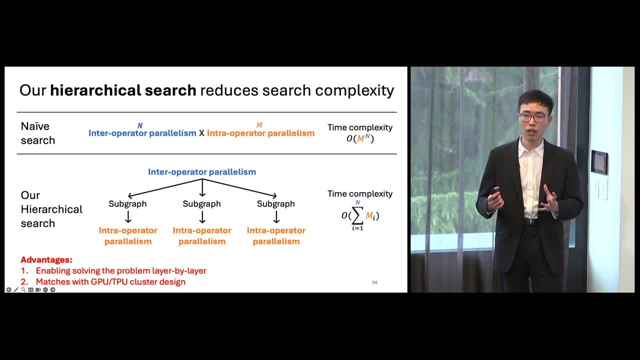 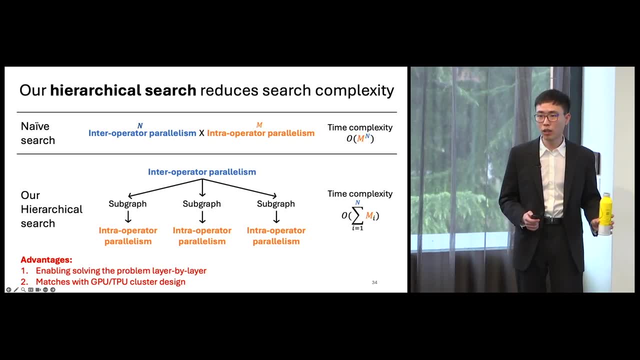 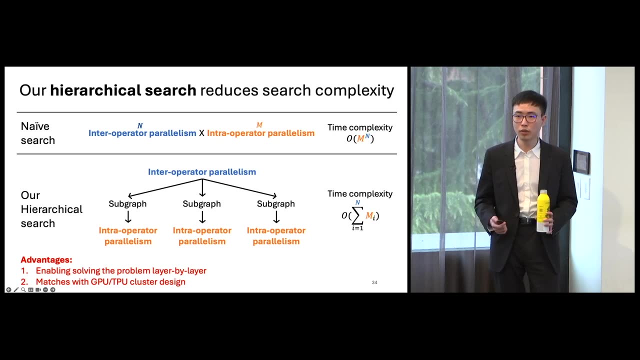 layer by layer, and it also matches the modern TPU and the GPU cluster design very well. So, while the high-level idea is intuitive, putting it into practice still requires sophisticated like optimization algorithms and high-performance distributed runtime to execute a strategy. So now 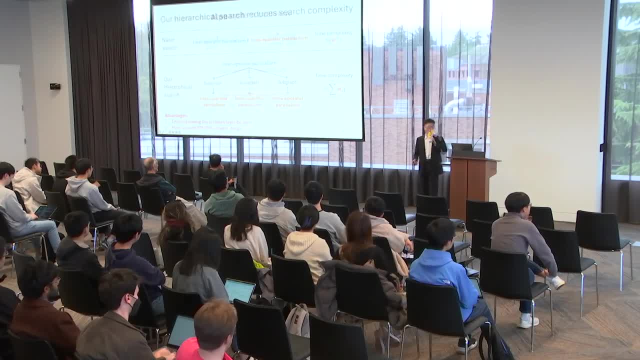 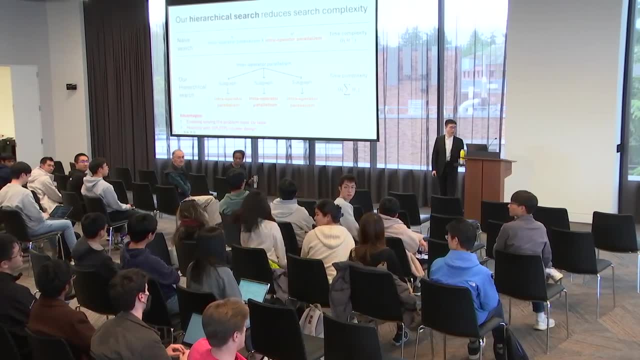 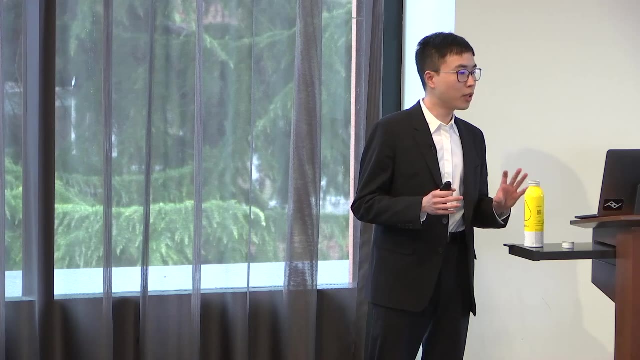 next I will go through some technical details. Okay, question: Why is this particular decomposition reasonable, Reasonable? Yeah, Okay, because you can think of that typically like: because the inter-operator communication, inter-operator probabilism, the communication is lower. 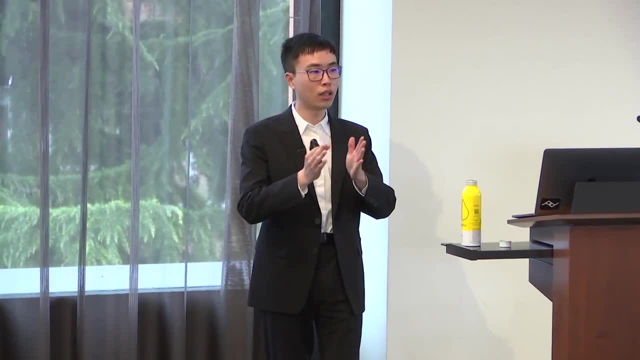 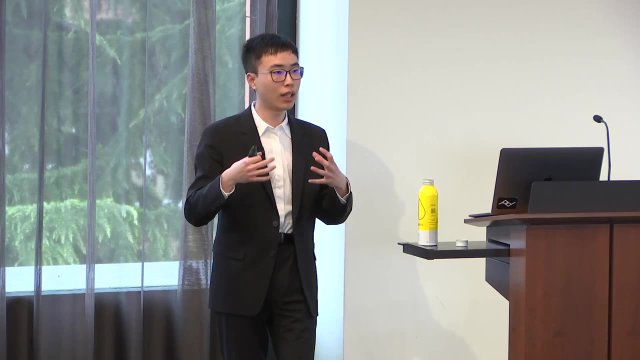 so we want to place it at a higher level. let them to go through the slower connection And then the intra-operator probabilism, because the communication requirement is higher. so we want to place it at the lower level so we can utilize some fast connections. 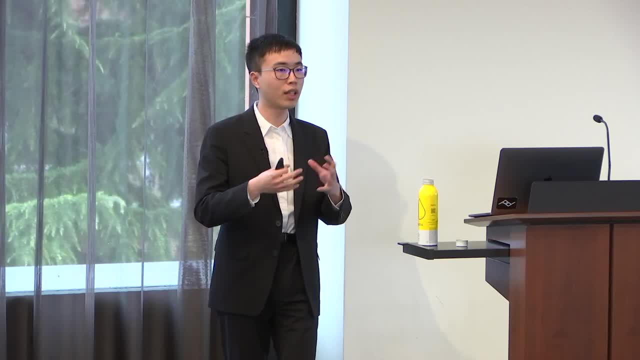 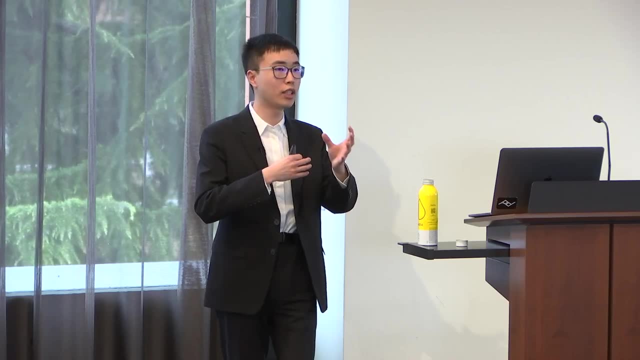 locally fast connections like NVLink inside a single node for them. So this kind of like decomposition also. it's also like highly inspired by how the GPU cluster is built. Yeah, I guess maybe you're getting to it. 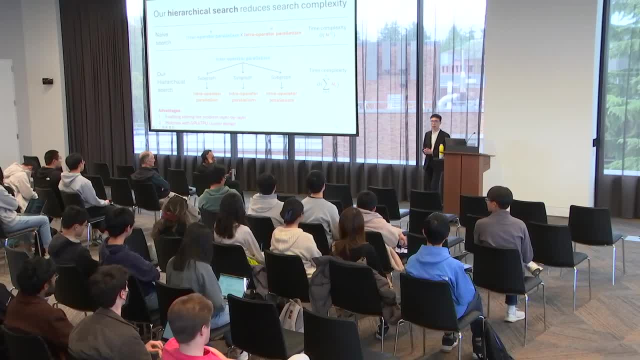 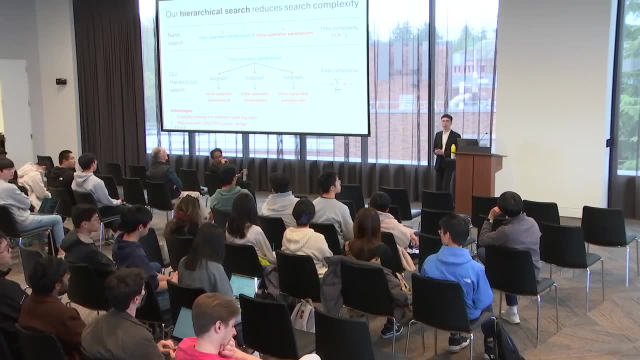 but it's, it's, it's, it's, it's, it's not clearly why you could make the inter-operator probabilism decision independent of knowing the intra-operator. Okay, yeah, yeah, this is a very great question, so I will show you. 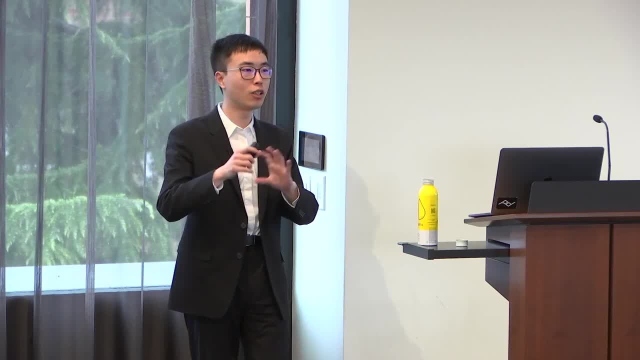 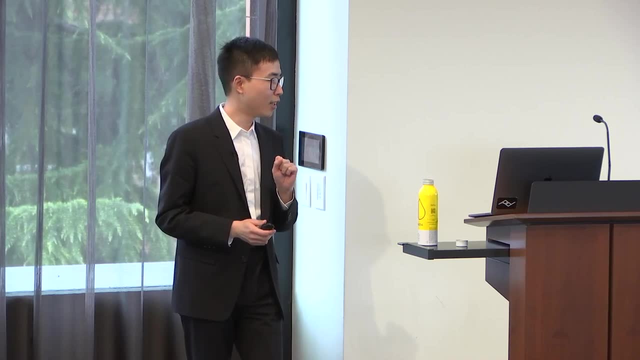 like they are not totally independent- yeah, although I like draw this composition, but later I will show you like they are not totally separate. Okay, great, Okay. so I basically follow this decomposition idea. we design a system. 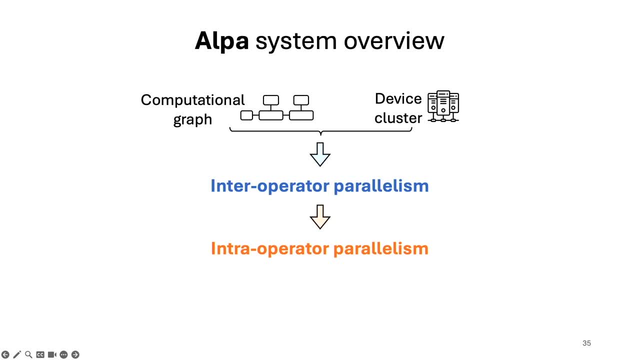 alpha. this is the problem as a computational graph for training large models and the device cluster, which can be a GPU or TPU cluster and, as as I said like, it's a two-level search. so we first tackle the inter-operator problem. 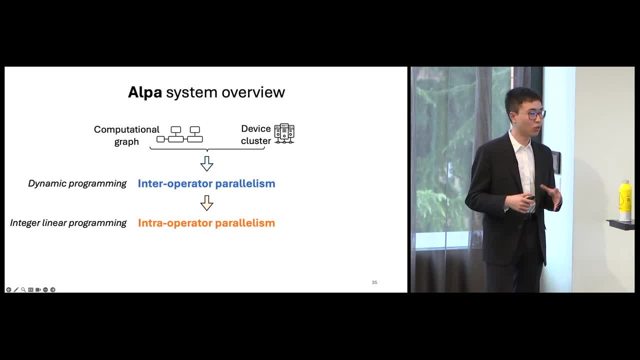 by using a dynamic programming algorithm. and then we go to the granular level, intro-operator problem by formulating it as an integer linear programming problem. So yeah, as as you said, like they are not totally separate because, like run the lower level, actually we need to run the lower level path first. 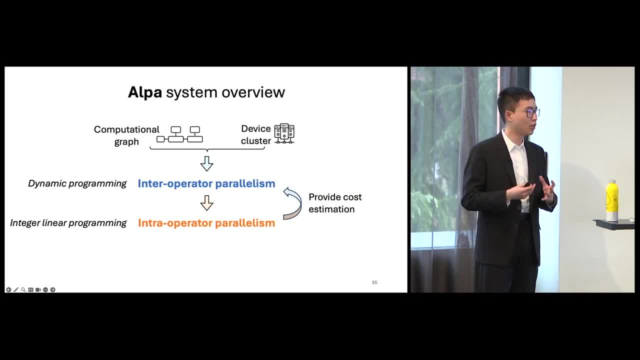 to build a cost estimation, to build a table, and then use this cost estimation, use the cost estimation from the lower level algorithm as input for the higher level algorithm and then it can make a planning for the higher level path. yeah, I think this can probably answer your question. 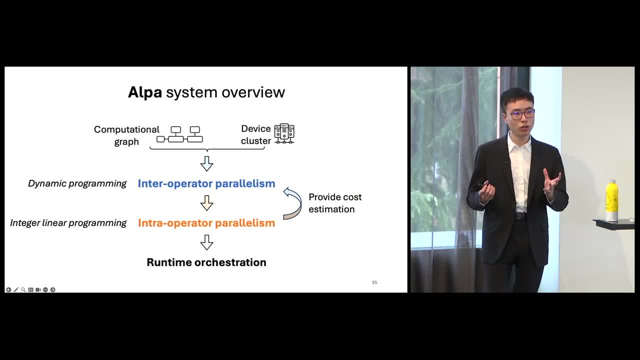 and then now because LPAR can generate a much broader array of different combinations or paradigms. so, like no existing system can execute the strategy generated by LPAR, so we also have to build our own distributed runtime to execute the strategy. so next I will go through the two major algorithms one by one. 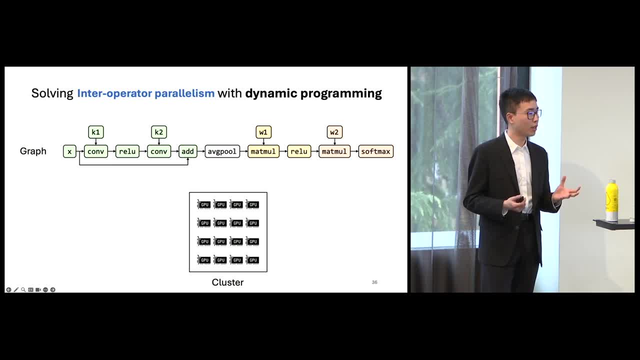 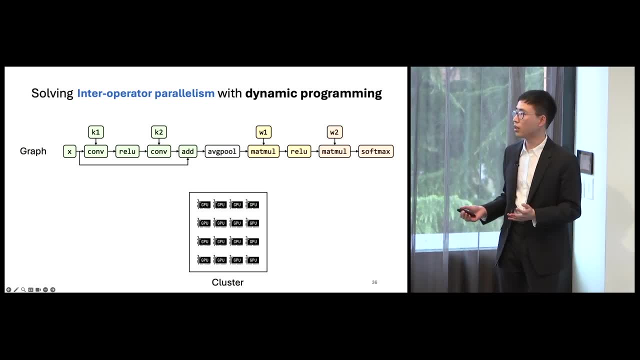 first we start with the inter of the paradigm and the goal. so here I show a graph with several more operators and skip connections, and below is a device cluster. we model a device cluster as a two-dimensional device mesh which we use different dimensions to model the communication. 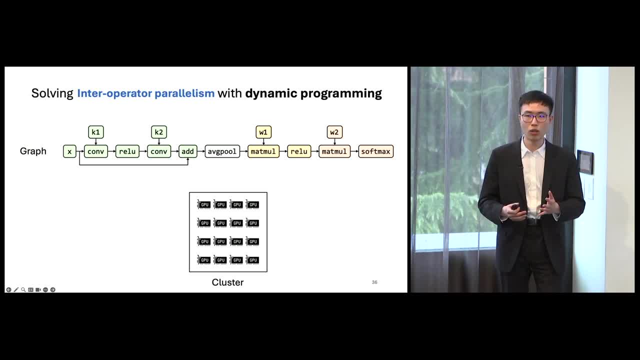 across different with different properties. for example, across row it can be like fast communication within a node and across column it can be slower connection across node. and our goal is to partition this graph into several stages and then allocate a sub-region of the cluster for this stage. 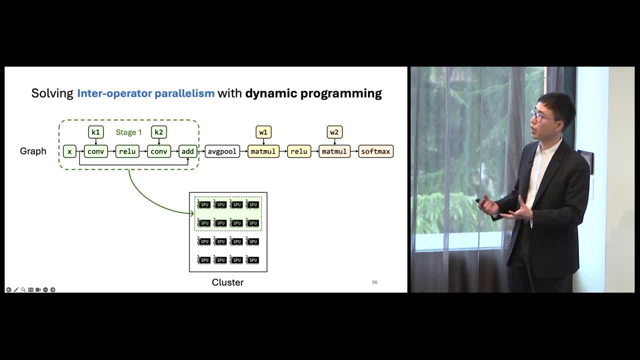 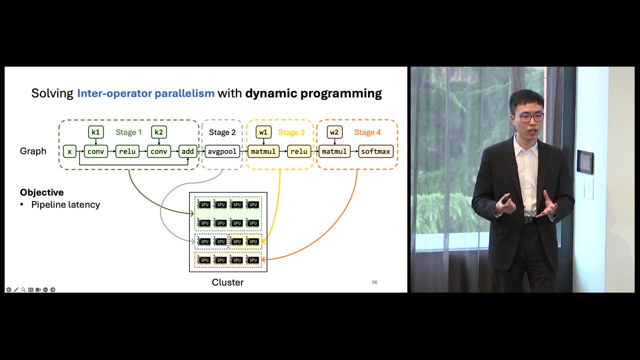 for example, we can group the green nodes together at stage 1 and allocate 8 GPUs for it, and similarly we can do it for stage 2, stage 3 and stage 4. so these stages will be executed in a pipeline fashion. so our goal is to minimize the latency of executing this pipeline across multiple data batteries. 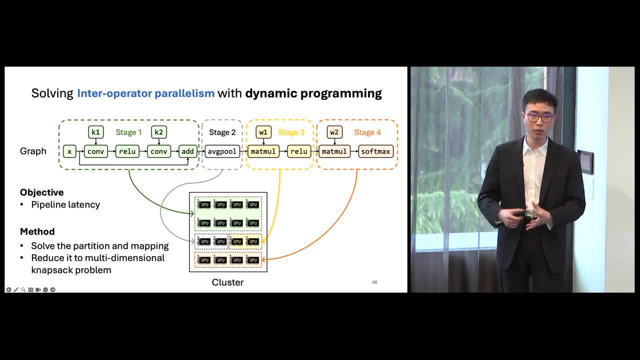 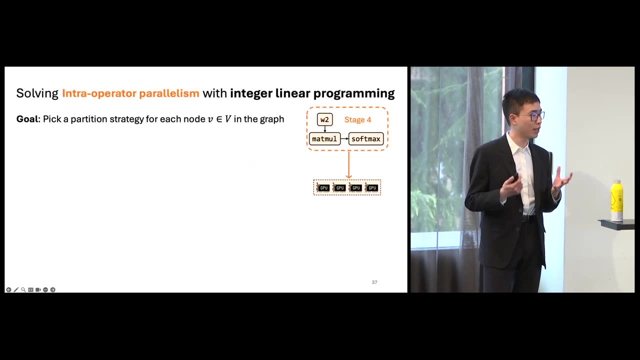 and we find that we can solve the problem of partitioning and mapping together by reducing it to a multi-dimensional knapsack problem. but I will skip the details for now. next, we can zoom into one specific stage, for example the orange stage 4 as an example. 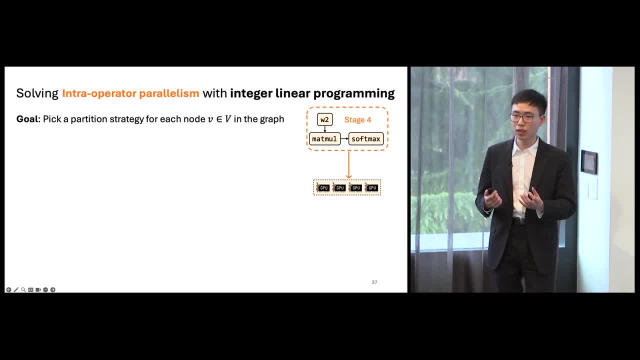 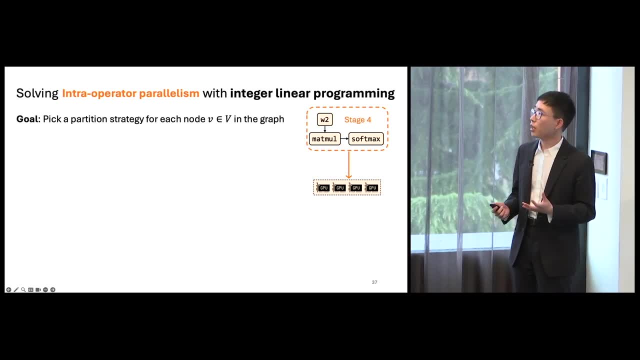 and we will solve the intra-orbital paradigm within the stage. so the goal here is to pick a partitioning strategy for each node V in the graph and because first we will define a decision vector, one-hole decision vector SV to represent the chosen strategy. because each node, they have many possible strategies to choose from. 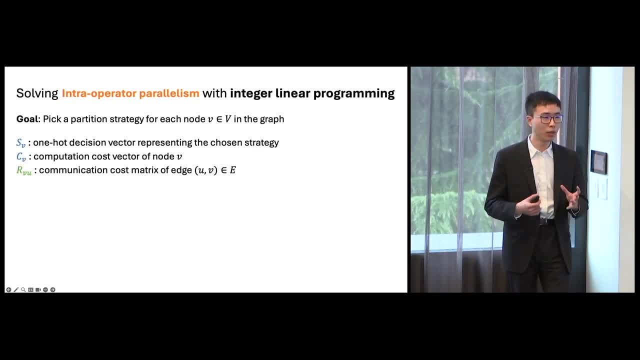 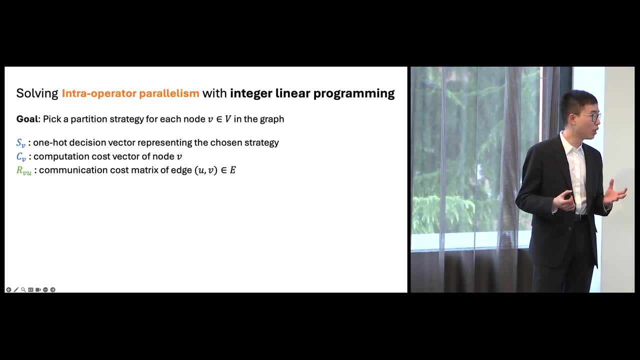 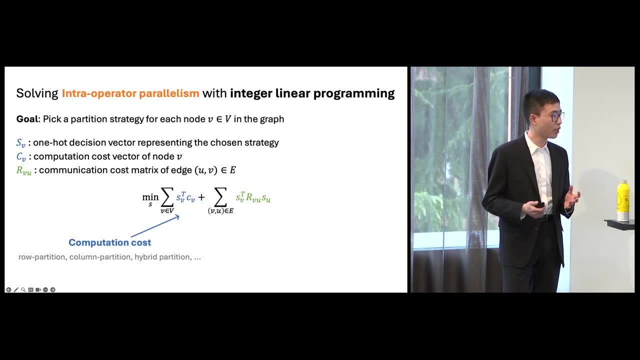 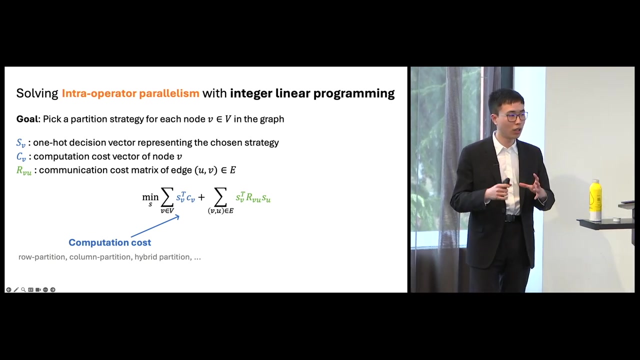 and then we use some profiling and a simple cost model to fit some constants, such as the computation cost on each node and also the communication cost matrices on each edge, and then with this constant we can write the objective. it consists of two terms. the first term is the computation cost on a node. 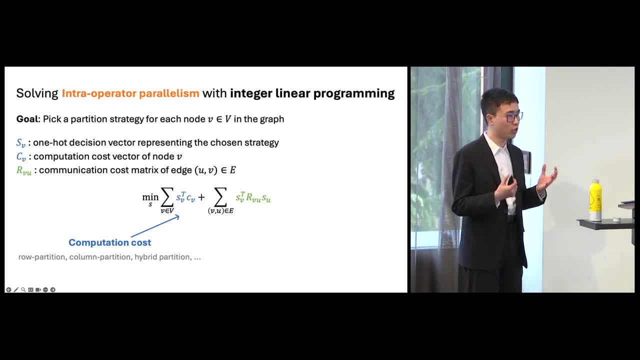 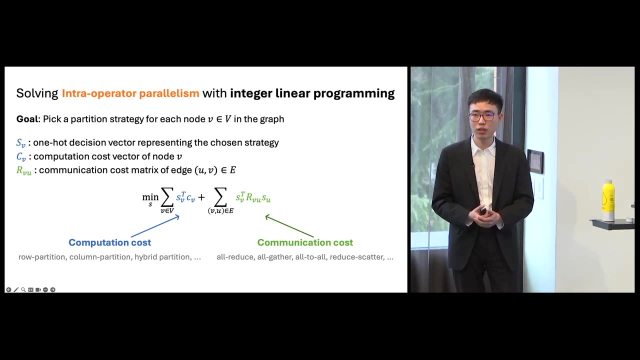 we formulate it. we integrate different partition strategies like row partition, column partition and hybrid partition. and for the second term, it's the communication cost on an edge. we formulate it using common connective communication primitives like all-reduce, all-gather, reduce, scatter. 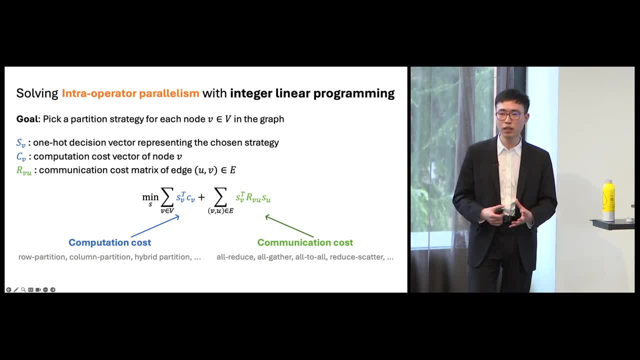 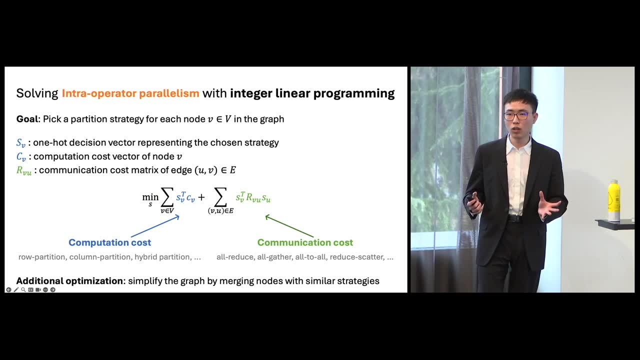 so by doing this we can build a program instance for the entire graph and solve it with integer linear programming solvers. and to handle larger graphs, we also applied an additional optimization that can merge some nodes with some similar nodes together, so this can greatly reduce, simplify the graph. 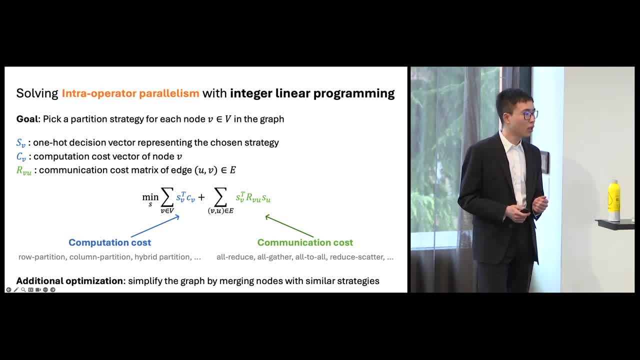 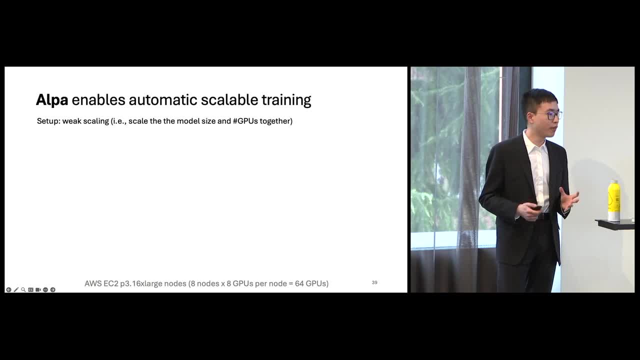 and reduce our complexity. now let's take a look at how ELPA performs. we are comparing ELPA to previous systems on three widely used models. we will test the scaling results on an AWS cluster with up to 64 GPUs. so first we benchmark on the GPT model. 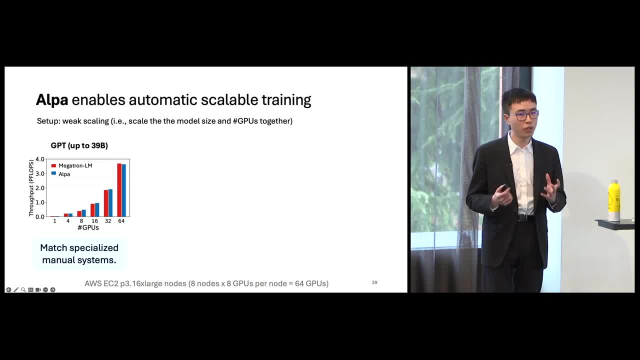 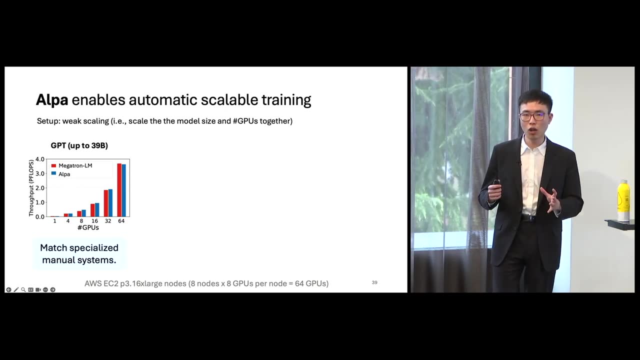 as you can see, the x-axis is the number of GPUs- we scale from 1 to 64 GPUs- and the y-axis is the training throughput, where a higher value is better on this benchmark. GPT is a standard architecture that has been heavily optimized for years. 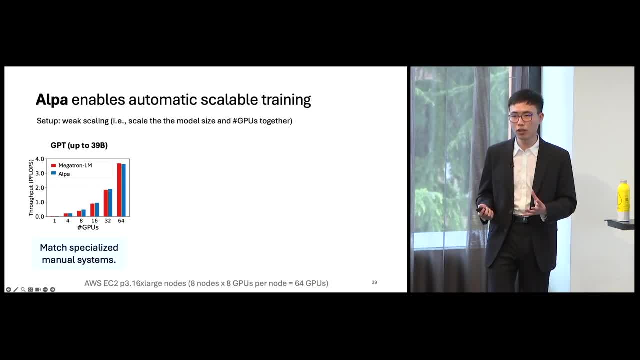 so we can show ELPA is able to match the performance of the best manual system, Megatron RLM, on this benchmark, but with automatic parallelization. and next up for G-Shot MOE, it's a transformer model with slightly different architecture, with some additional mixture of expert layers. 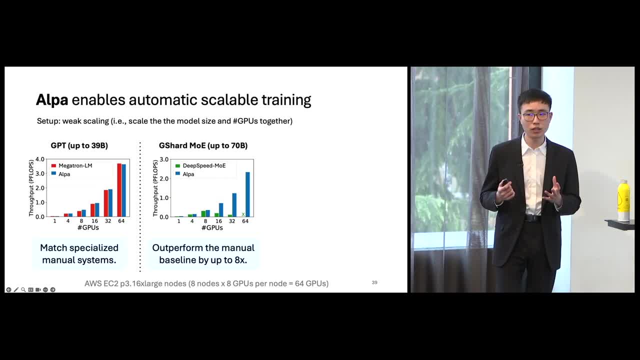 and in the figure we can see when the number of GPUs goes beyond 32. we can show that ELPA is able to outperform the best manual GPU baseline by up to 8x on this AWS cluster. so this is achieved by integrating various forms of parallelism. 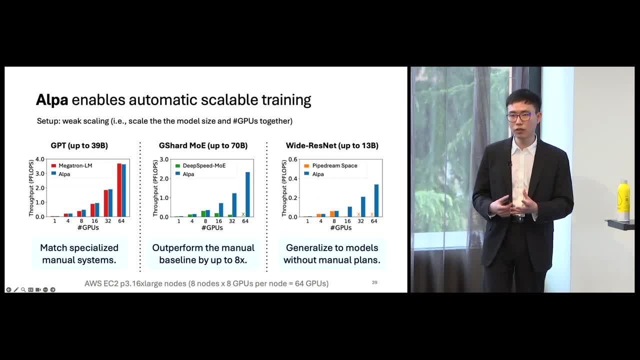 and lastly, for Wide ResNet. it's an architecture very different from transformer and previously there is no existing model parallel strategy for it. so we show that ELPA is able to generalize to this previously unseen architectures without manual plan, and you can see when the number of GPUs goes beyond 32. 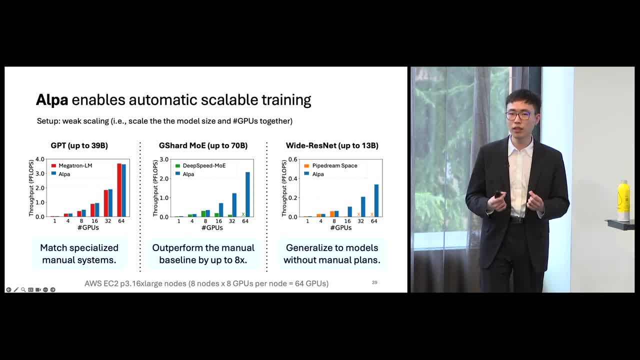 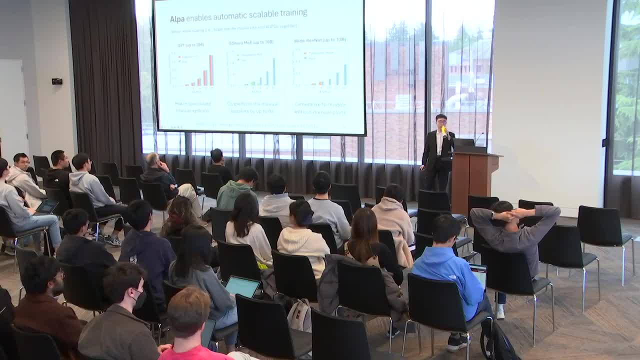 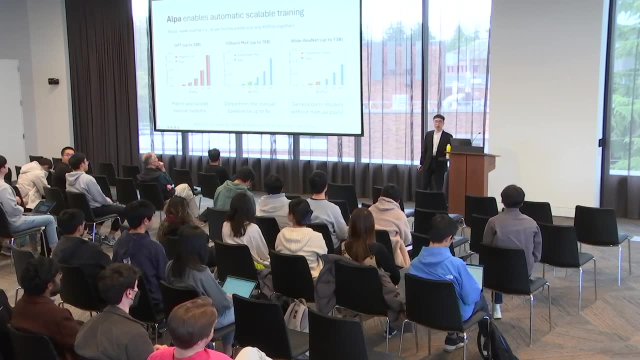 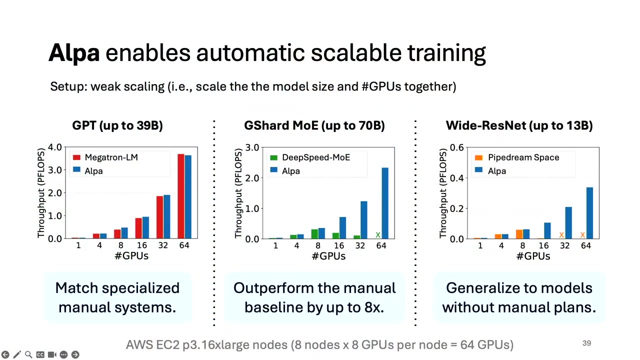 ELPA is able to almost maintain a linear scaling, but the best existing auto-parallelization system failed because of auto-memory, the memory footprint or the standard parameters or the training gavel set size. okay, so this: B are the number of parameters. for example, 39B is the 39 billion of parameters. 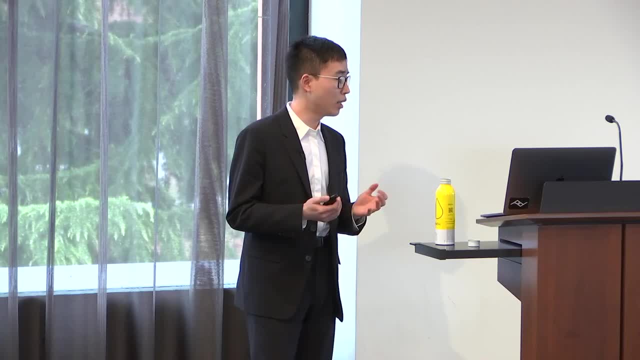 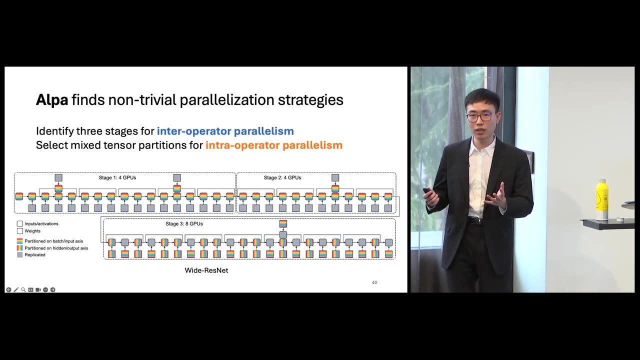 great. so here is an example of the optimal strategy we find for Wide ResNet. it's a massive graph but it's just an example to show you that these strategies are non-trivial and it's very easy and very hard to manually design and cannot be found by 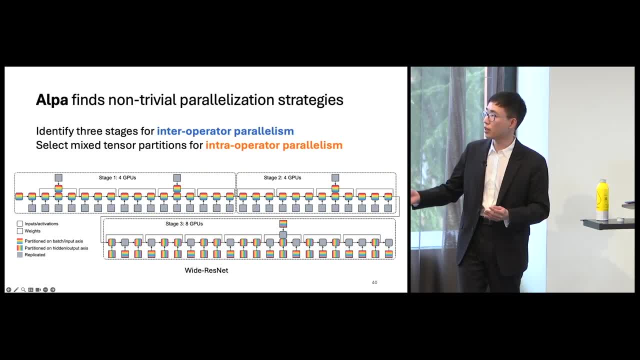 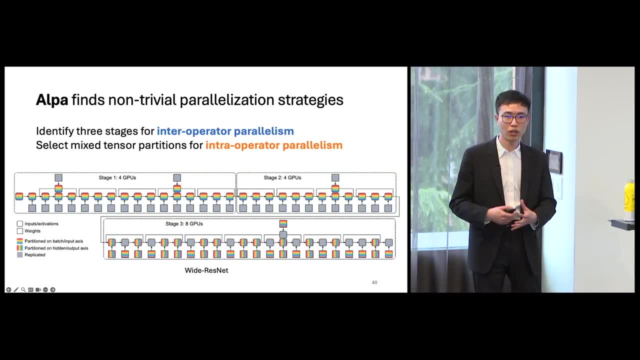 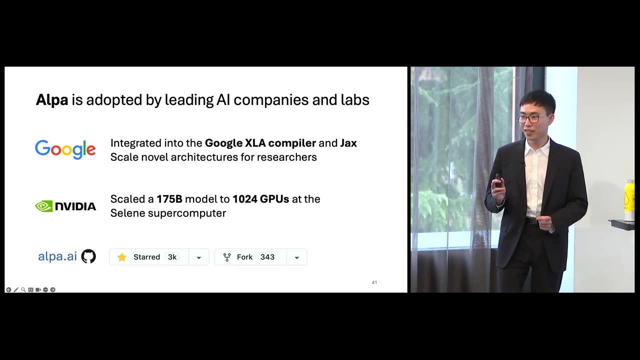 previous auto-parallelization systems and you can think of, you can see the stage 3, where the different colors indicates different tensor partition strategies on input dimension, output dimension, different channel dimensions. so okay, let's take a step back. I just wanted to revisit the question from earlier. 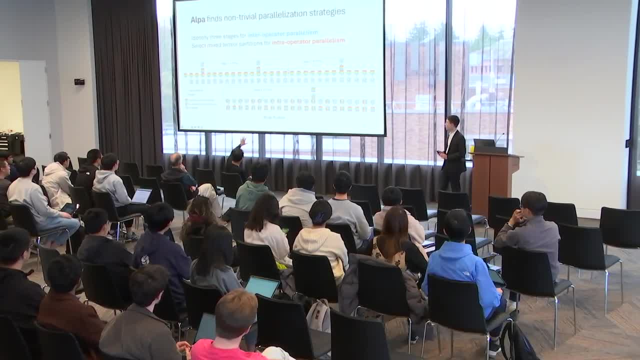 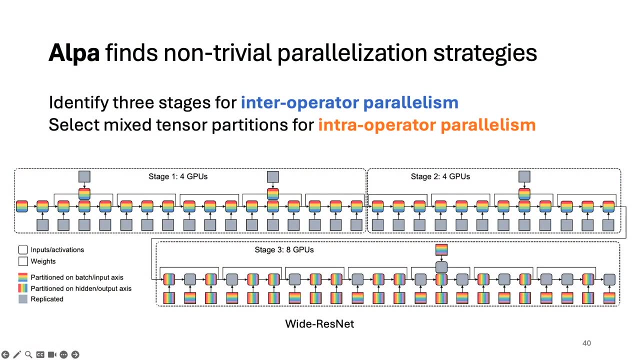 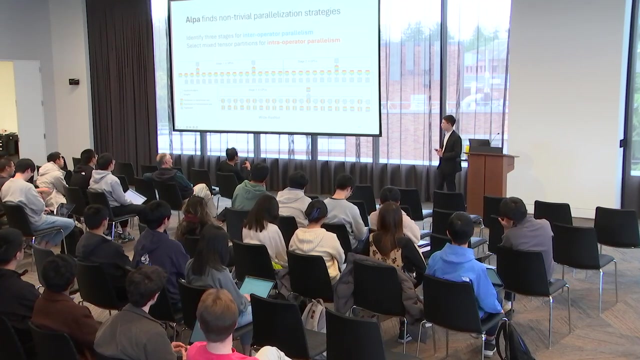 so if I look at something like this, this allocation, like this, there's an answer. but there's an aspect of you know the you need a model of what the intra-operator parallelism is, to understand how many GPUs to allocate to some number of stages, and that is going to be a function of 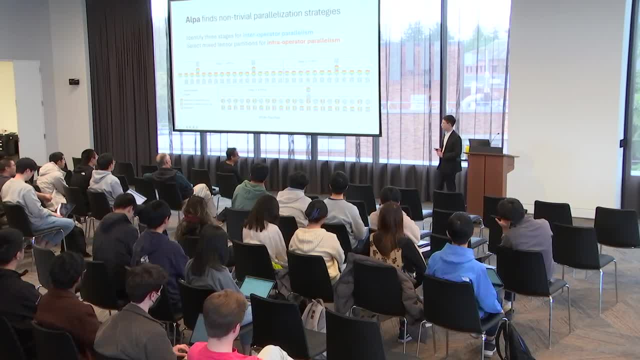 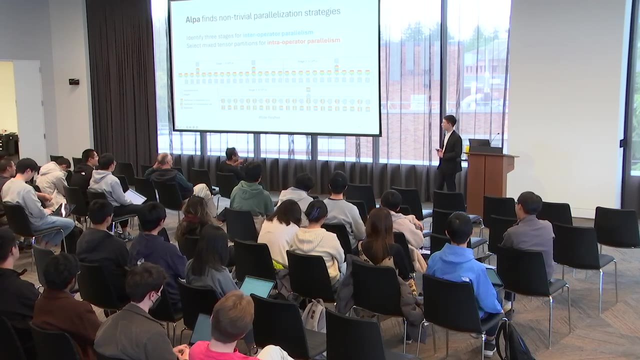 maybe the layouts across stages potentially? or what communication? what would be the communication cost across stages? so it seems like fundamentally the whole system optimization problems. can you comment a bit more on why the can you have enough information of the intra-operator parallelism to be able to feed into this inter-op parallelism? 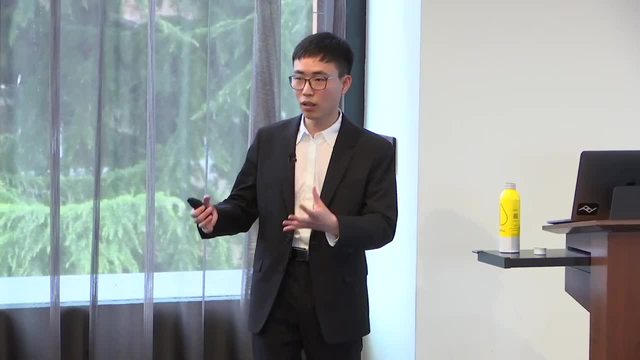 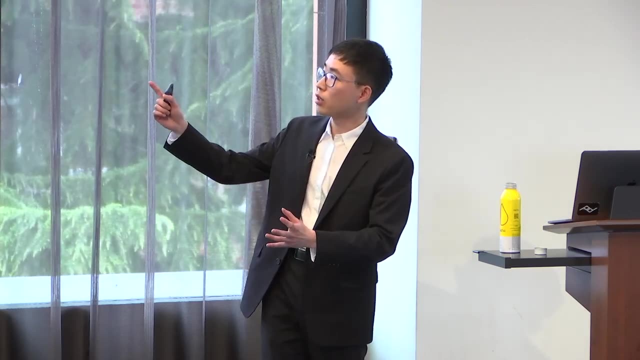 okay, yeah, I think we do it like from lower level to higher level, and for lower level, we'll enumerate a lot of things, we'll enumerate a lot of possible stage partitions, and then we build a table and this table can be done. the construction of this table. 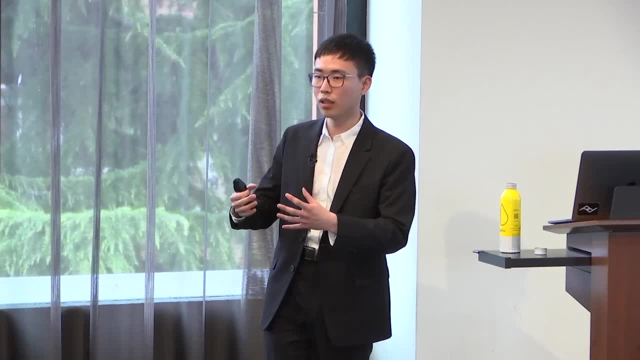 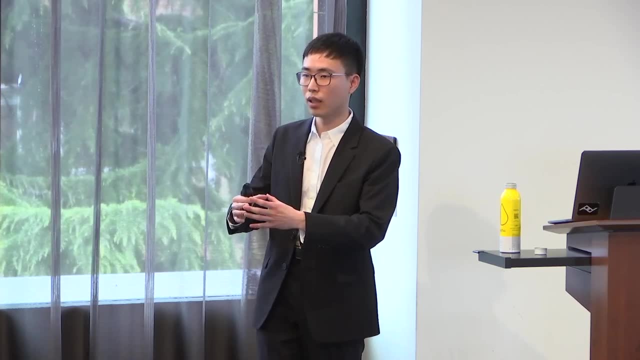 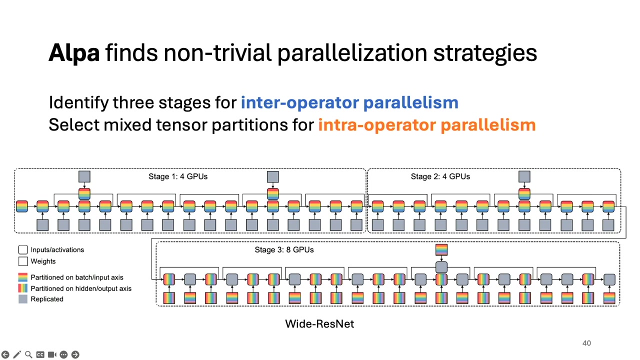 can be done in parallel. so we parallelly enumerate a lot of things like the size of sub-cluster and like the size of sub-graph, this kind of things. we enumerate all of them and solve all of them and build a table and then use this table as the input. 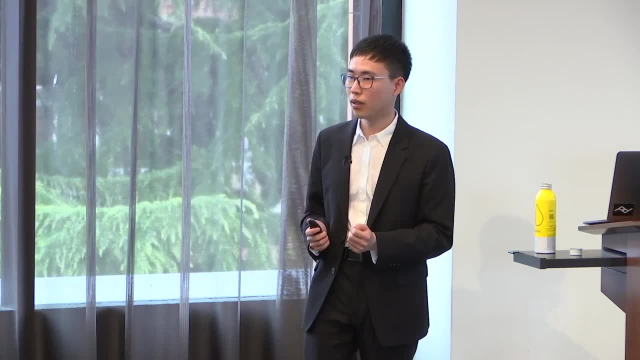 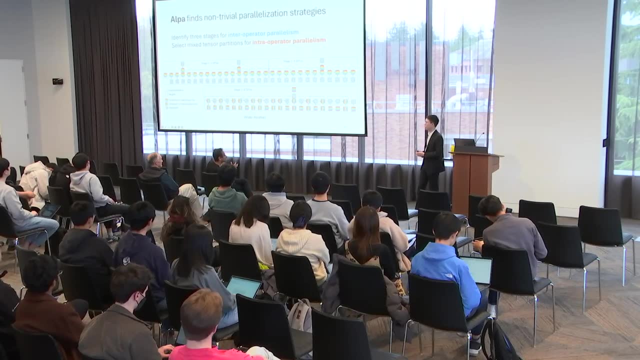 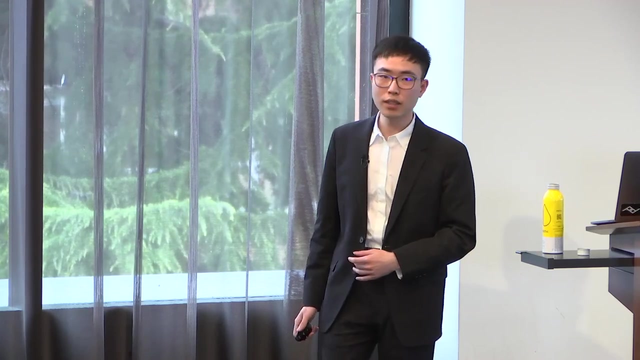 for the higher level dynamic programming algorithm. so in some sense the output of the lower level is also parametrized by the amount of resources that you allocate to each. yeah, yeah, yeah, okay, so let's take. okay, one more question. yeah, I was curious also how your solution would work. 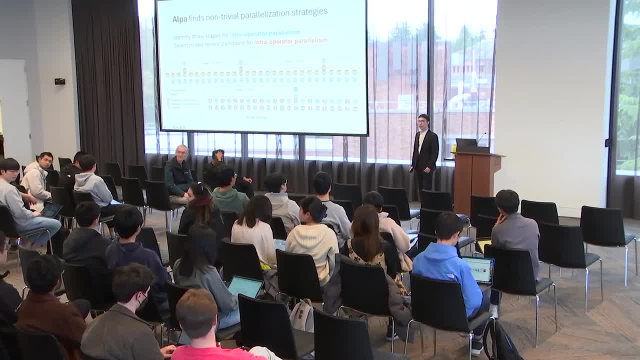 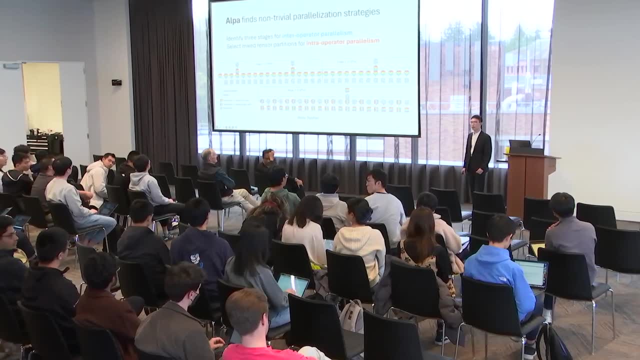 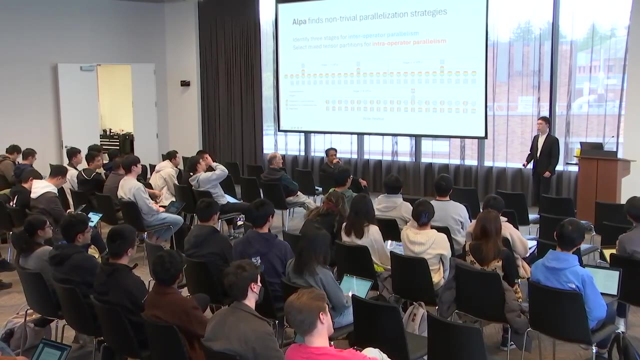 if you're also considering kind of different schedules for the intra-operator. so is it like: do you support like just one schedule right now, or because, like, if you have to consider different schedules, then that seems like maybe another dimension that you need to add on. okay, so you are talking about. 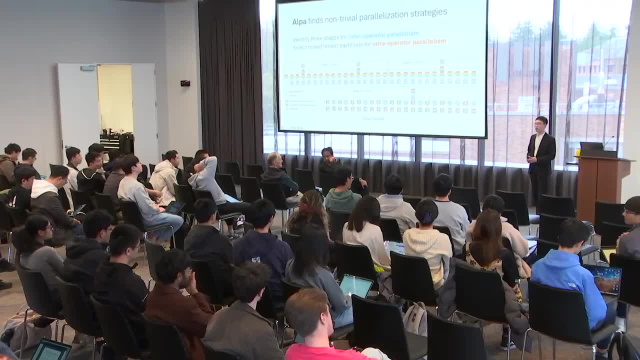 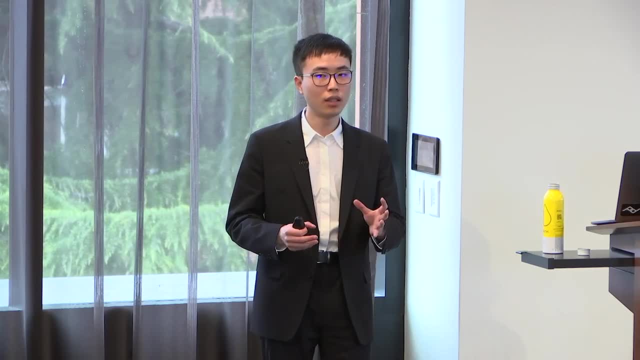 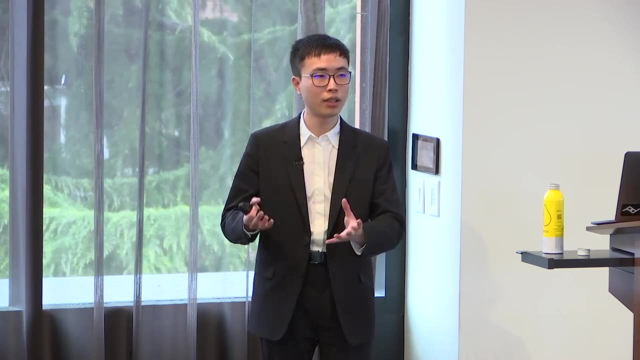 are you talking about like pipeline parallelism schedules? yeah, so currently we fix like one forward, one backward schedule. that's a standard schedule. yeah, and it can already work well for our programs, like the bubble is more so we design our objective given this schedule, but in the future definitely. 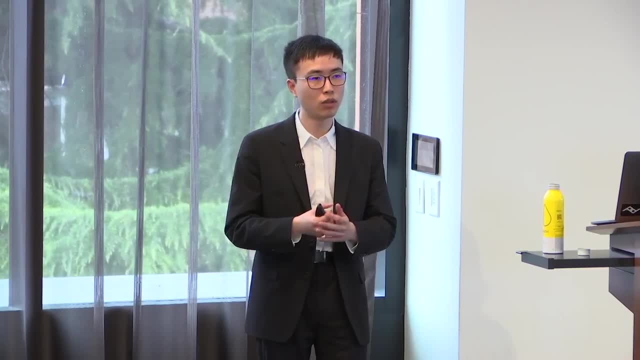 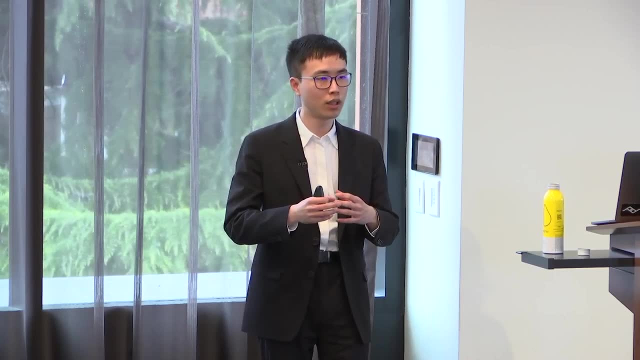 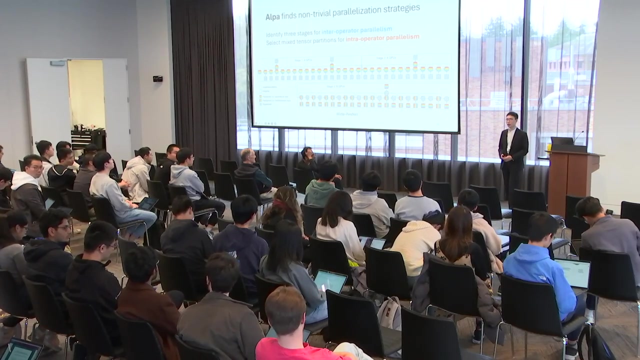 you can relax this a little bit and try to also search for different pipeline schedules, and it can probably give you some more advantage when you are dealing with like graphs with branches, something like this: do you have a sense of how that would affect the search time for search time? 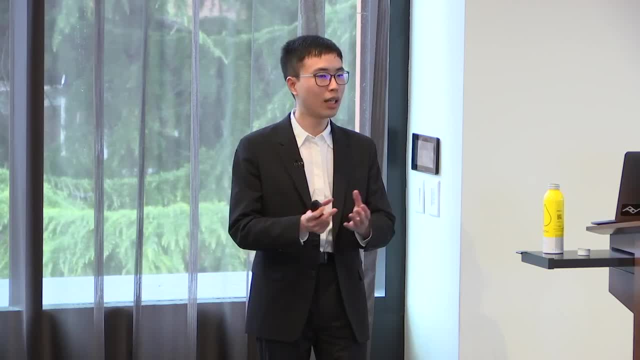 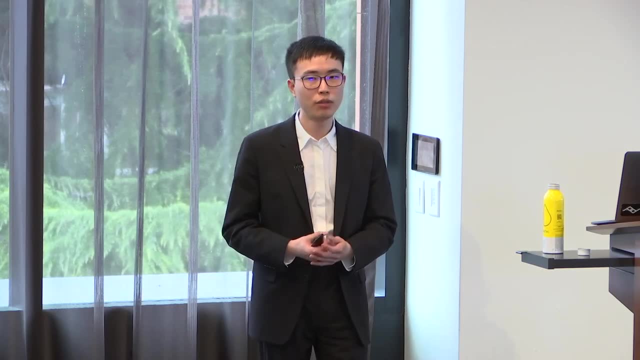 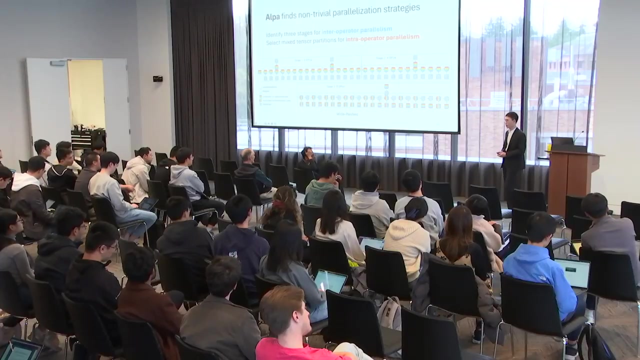 yeah, as you said, you introduced a time dimension. yeah, that would make the search much more complicated. yeah, so currently our search takes several minutes. if you add another dimension, probably that will definitely take longer, okay, okay. so, yeah, we can take a step back from the technical details. 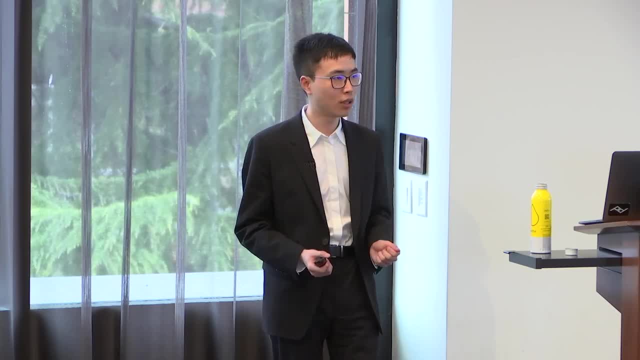 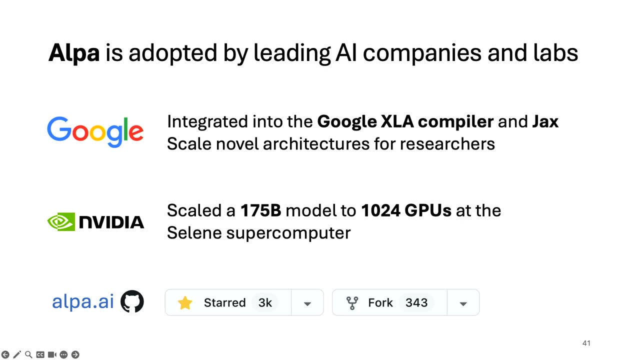 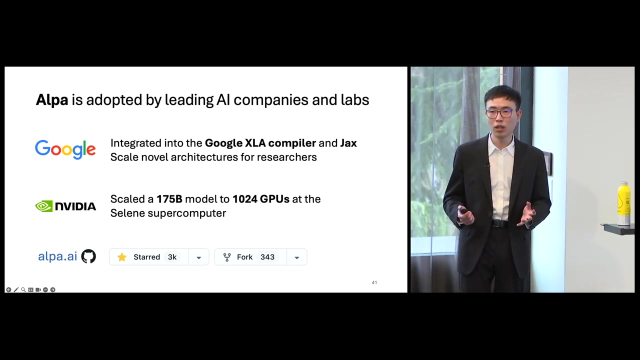 and see how ElPi is used in the real world. at Google, ElPi has been integrated into the Google XR compiler and the JAX deep learning framework. it helps Google researchers to scale their novel model architectures. at NVIDIA, we collaborate with their team to scale the training model. 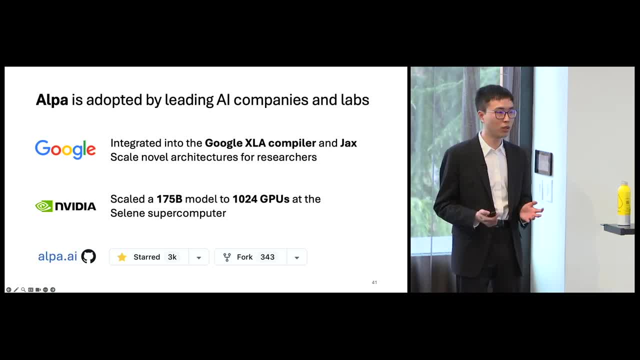 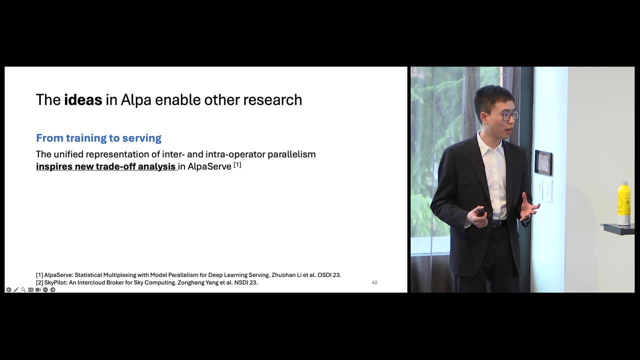 with 175 billion parameters across 175 billion models, across 700 GPUs on a supercomputer and besides the impact of the software artifact, we think the ideas in ElPi can probably last longer. so let me show you how the ideas in ElPi impact other research. 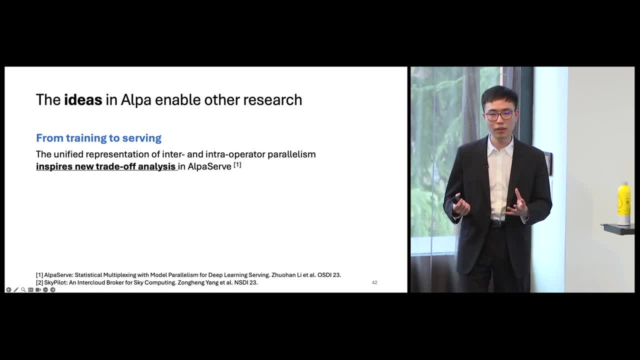 so initially we designed ElPi for training, so we have the unified reputation of inter and intrapolar capitalism. later we find the same set of abstractions can also be utilized to analyze the trade-off for the online model serving so, and the same abstraction will lead to. 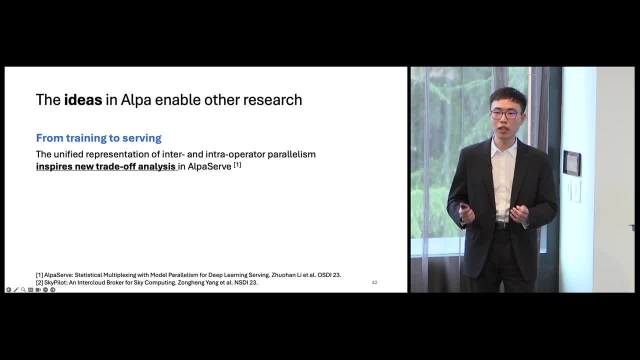 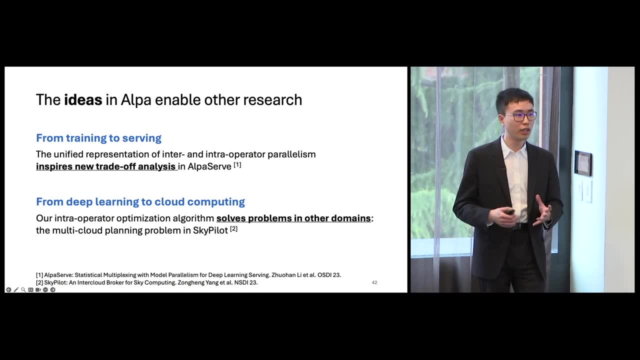 different trade-off analysis. so this leads to the ElPi server project and then initially we designed the organization algorithms to solve our own problems for the deep learning training. interestingly, the problem formulation is very general, so, like researchers from other domain can directly adopt our organization algorithms. 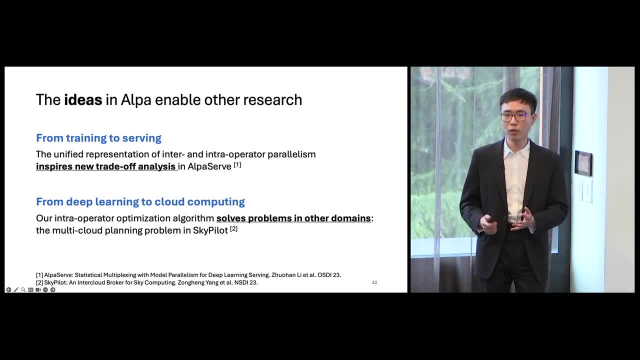 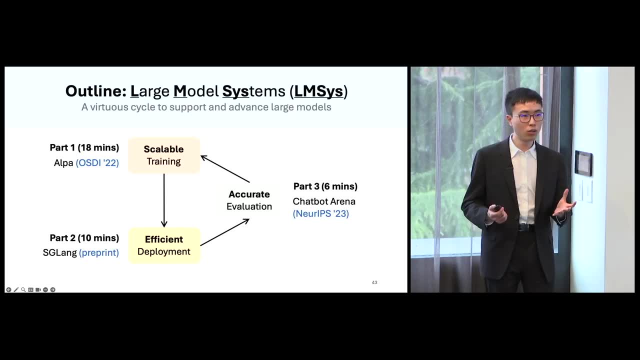 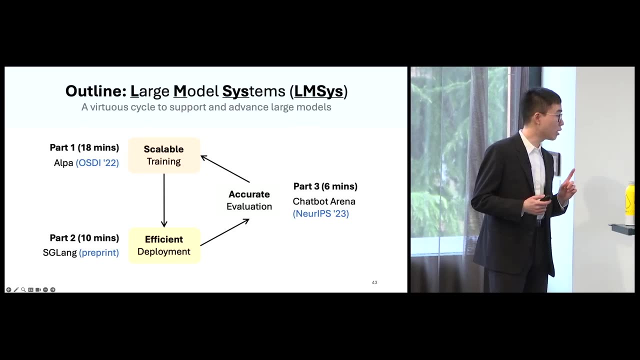 and solve the problem in their own domain, such as the multi-cloud planning problem in Skypilot. okay, so this concludes the ElPi part. let me go back to this timeline and and so next. so in ElPi we learned how to co-optimize the inter. 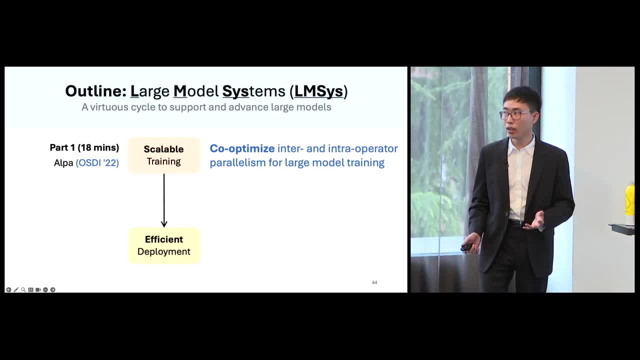 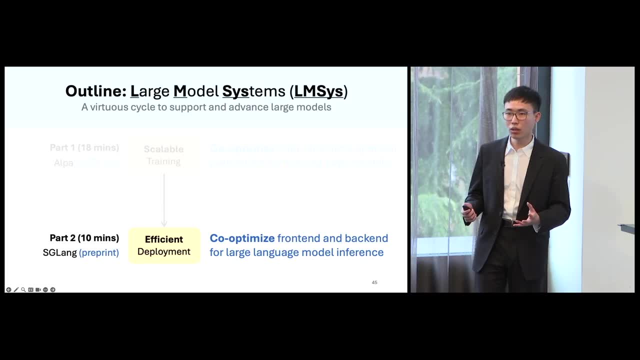 and intrapolar capitalism, for large model training and next, after training a good model, we want to deploy it for inference. so in the next project I will tell you how we co-optimize the front-end, the back-end, for optimizing large language model inference. this concept, 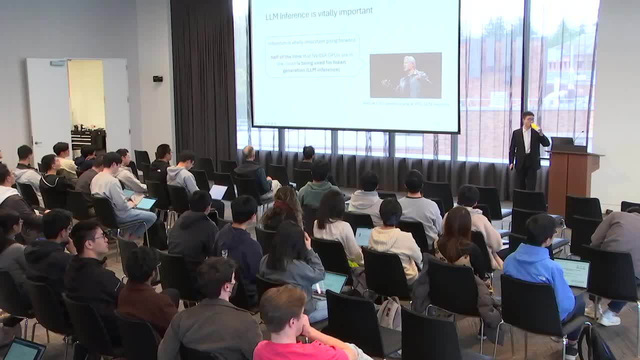 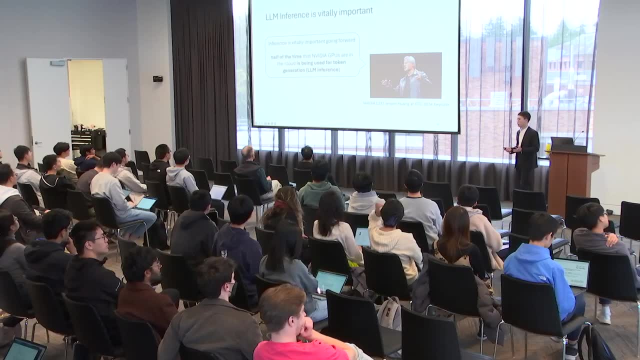 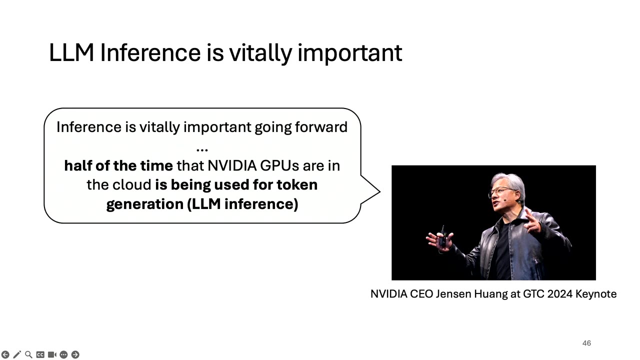 leads to the next project, SGLang. so LLM inference is vitally important going forward. so this is at the GDC keynote just happened last month. the CEO of Nvidia, Jensen Huang, emphasized this and he mentioned that half of the time the Nvidia GPUs in the cloud these days. 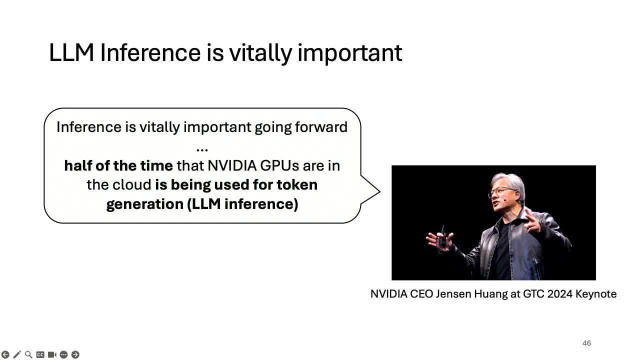 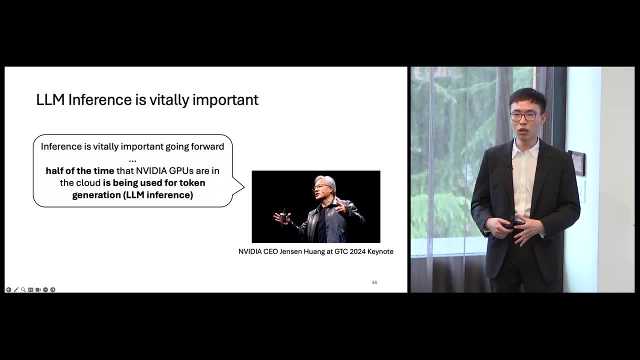 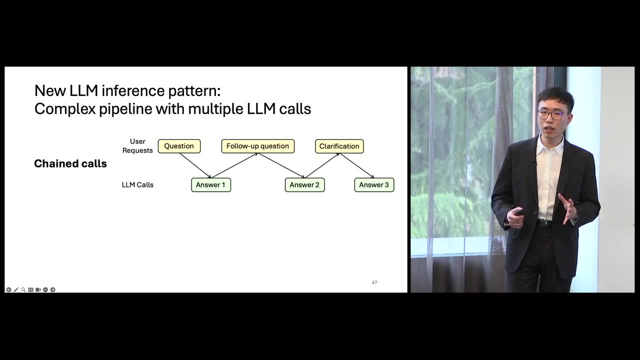 are used for token generation or LLM inference. so optimizing for inference is as critical as optimizing for training. on this part, I will show you some new common patterns in LLM inference and show you how we optimize for these patterns. so in an LLM application, if you want to, 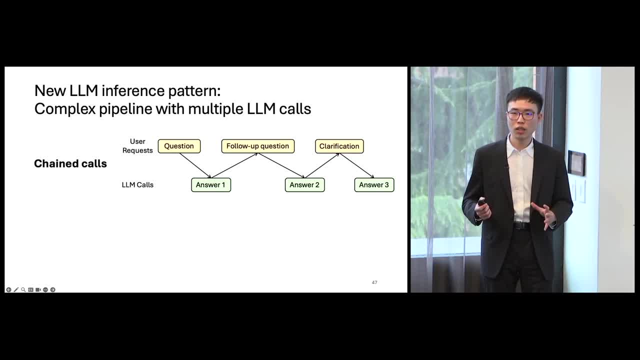 accomplish some complex task, it often requires not only a single LLM invocation, but the integration of multiple LLM codes. I will show you some common patterns. the first pattern is chained codes. for example, a user can engage with a multi-turned conversation within an LLM and the user can ask: 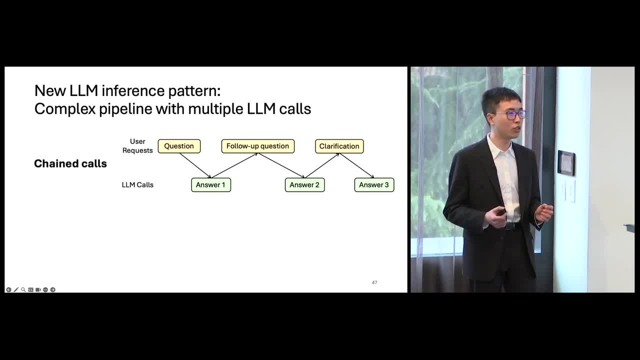 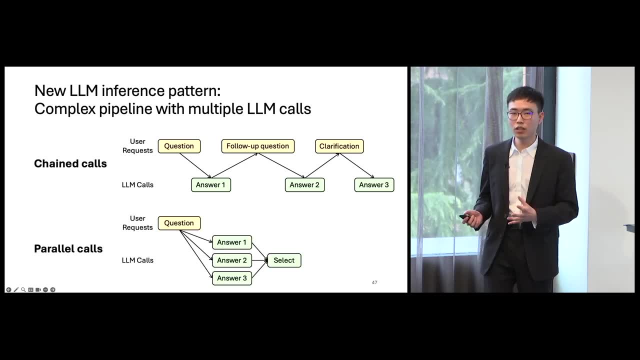 a series of questions. to generate the answer, the inference system needs to process a chain of multiple LLM codes and another pattern is parallel codes. so this figure shows a prompting technique that involves parallel codes. for example, to answer a user question. we can generate, we can launch. 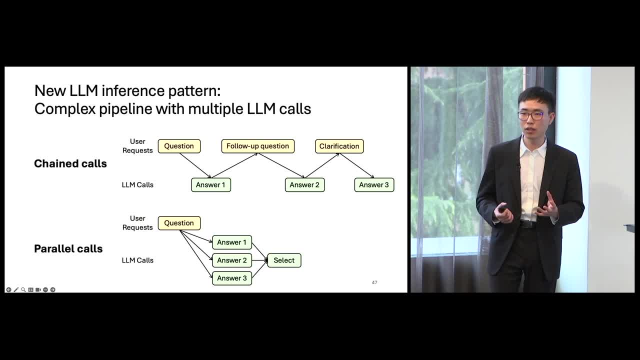 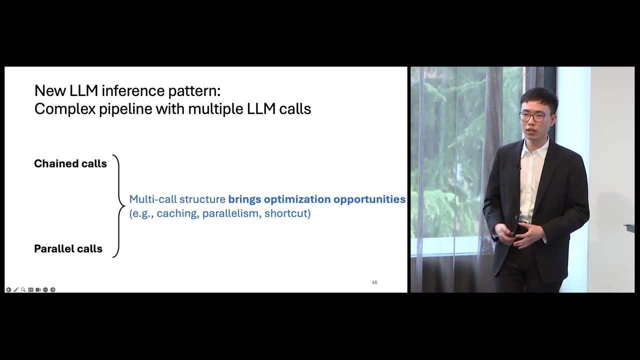 multiple LLM codes to generate different versions of the answer, and then we use another LLM code to select the best answer from them. so this can improve the solution quality. so this kind of multi-code structure brings many interesting runtime organization opportunities, such as caching, parallelism. 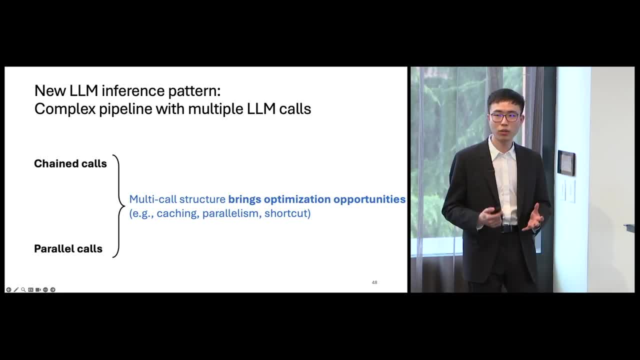 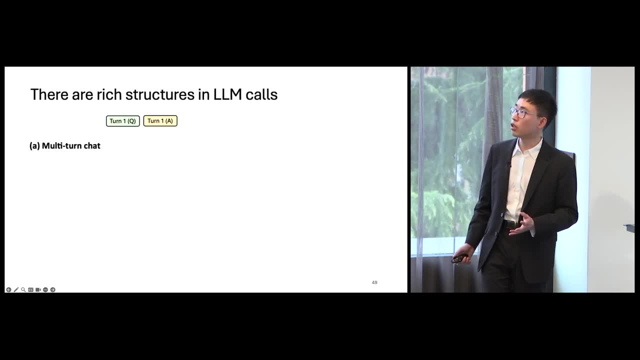 and short-cutting execution. however, these structures are very important for accelerating inference, but they are largely overlooked by existing systems. so let me show you the structures in LLM code so we can start from the most basic use case of LLM chatbot. so here, in the first term. 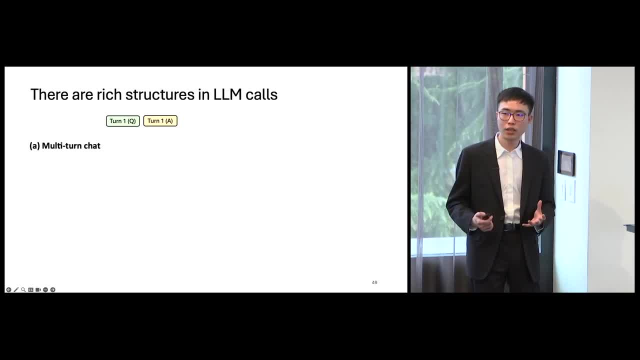 of the conversation. the user asks a question denoted as a green box here. the LLM then generates a reply denoted as a yellow box here. most systems just optimize for a single term or single pair of green and yellow box here, however, as the chat session 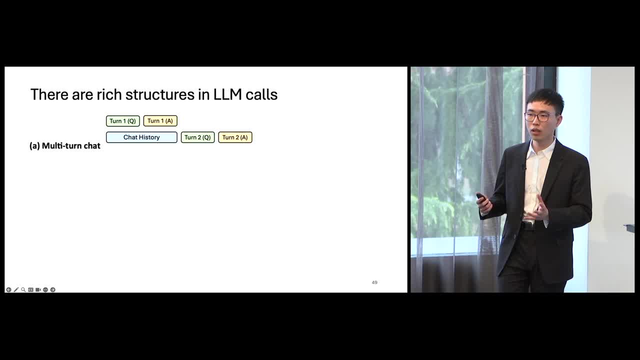 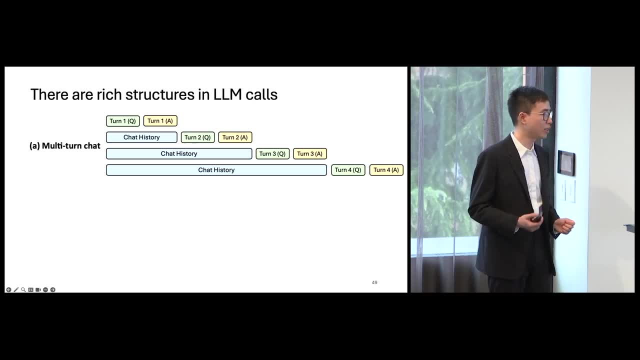 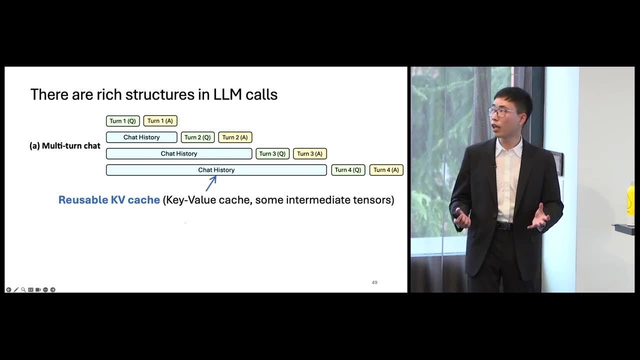 continues, we will have 10-2 and 10-3 and more times. so the chat history here is an accumulated structure with some runtime organization opportunities. so during the LLM generation process there are some intermediate tensors called kvcache. they are intermediate tensors generated during. 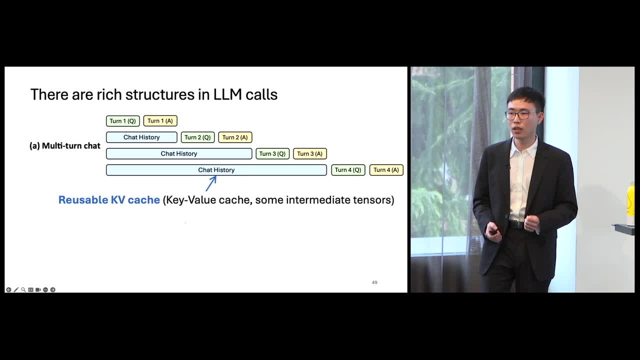 the forward pass and will be reused multiple times for decoding future tokens though, and it only depends on how many kvcaches you have, so you can see here different sequences. different requests with the same prefix can reuse the kvcache, in this case all the blue boxes. 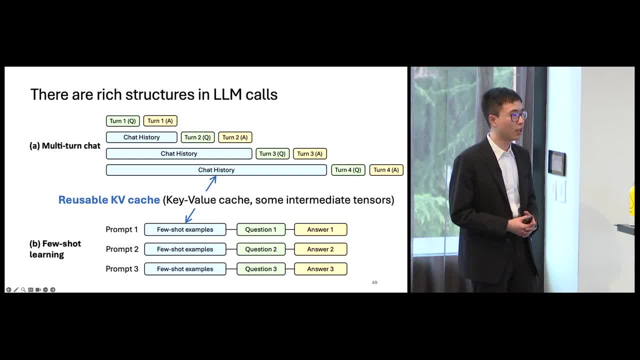 can be reused and shared, and this shareable structure appear in lots of other common LLM workloads. another case is future learning. in future learning, different requests can share the same set of future tokens, so in this case, all these blue boxes can be shared across multiple. 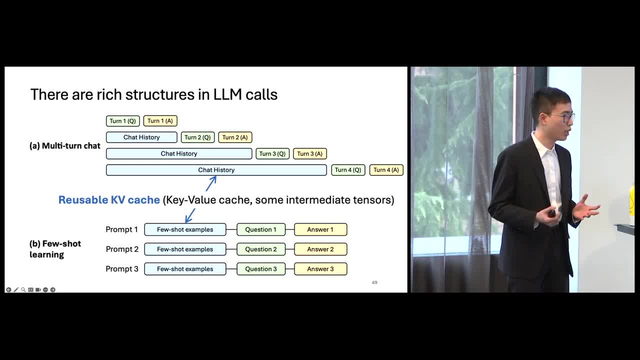 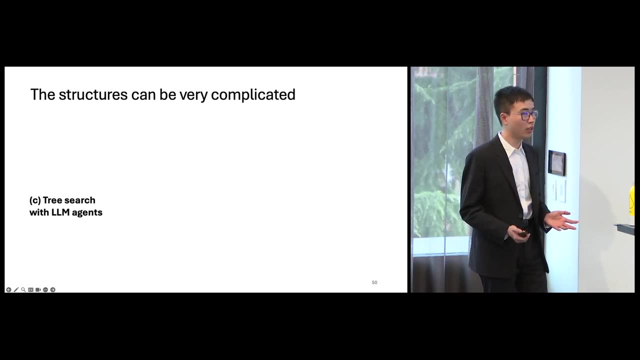 codes, but existing system just don't utilize these opportunities. this is because this shareable structure are scattered around multiple codes. sometimes it's very hard to track the state and reuse them, and the shareable structure can go very dynamic and complicated. so here I will show another complicated 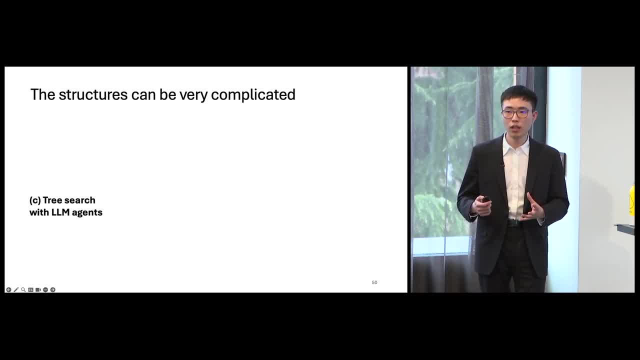 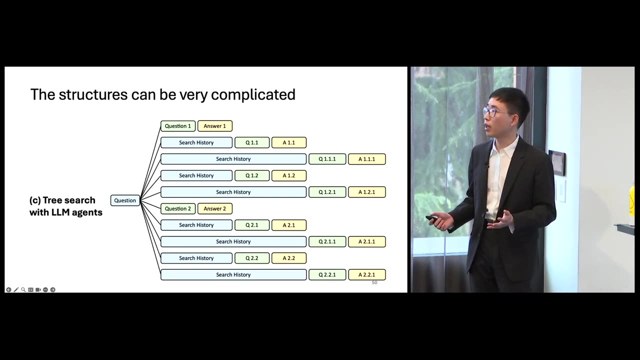 example, you want to use LLM combined with the tree search to solve the problem. so you may combine the LLM with some tree search algorithms, such as the depth first search, and you will let the LLM to explore different branches. so here I show you a search tree. 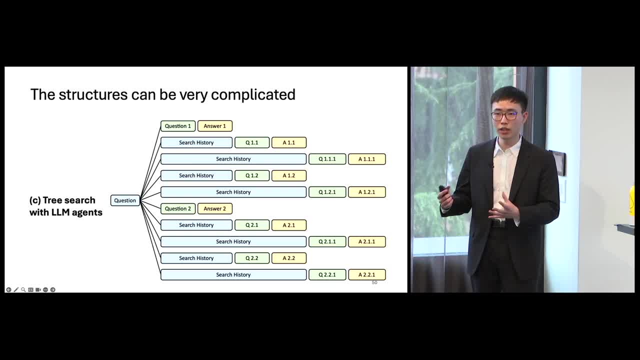 you can think of that. LLMs are exploring different branches in the tree, propose new branches and verify some new branches and prune some branches in the middle. so in this case all these blue boxes show KV cache and you can think different branches can share the KV cache. 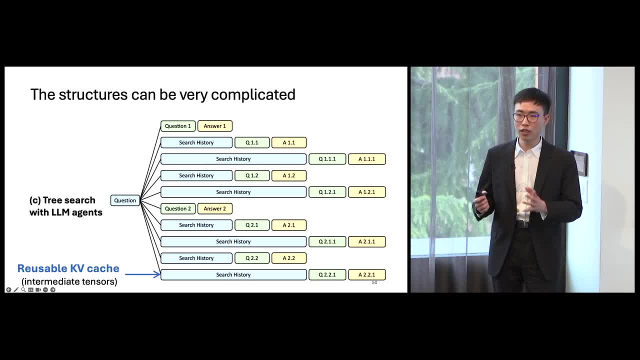 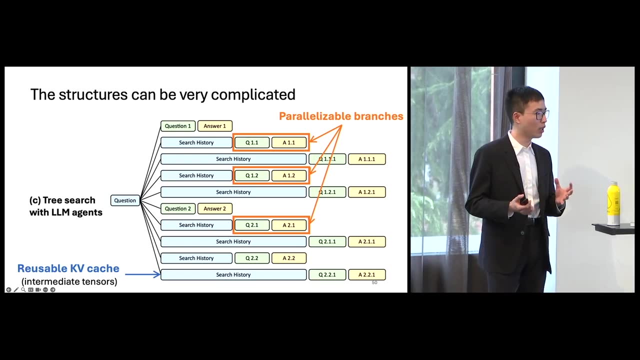 of the common parent parent nodes. so this creates a complex tree structure showing and no existing system can handle all the reuse opportunities within the tree and you, additionally, you can imagine some branches can run in parallel, such as the branches denoted as this orange box here. okay, 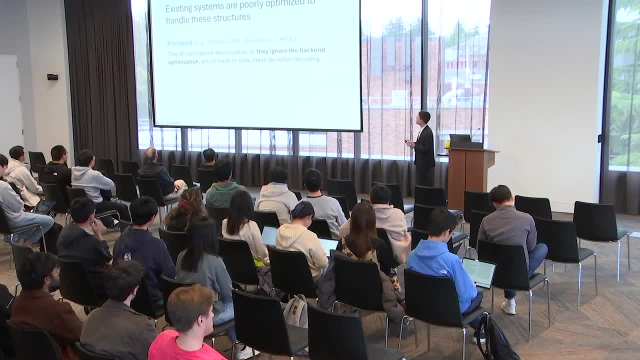 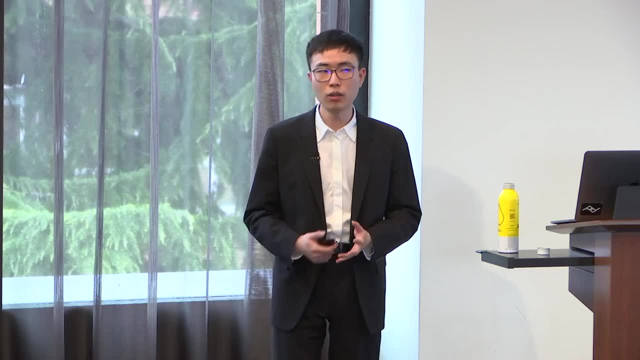 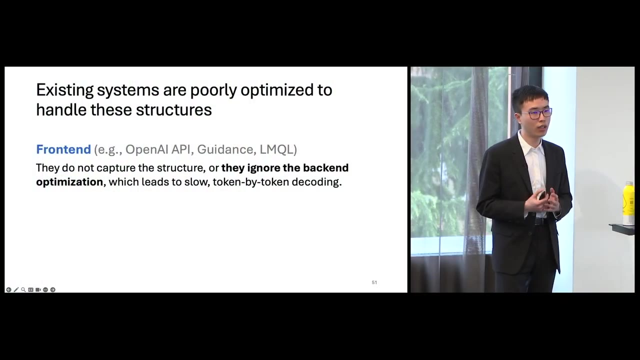 so leveraging this structure is very important for accelerating inference. but existing system are poorly optimized to handle these structures. so I will categorize existing system as either front-end organization or back-end organization. so on the front-end side, when calling large-ranged models we typically use some: 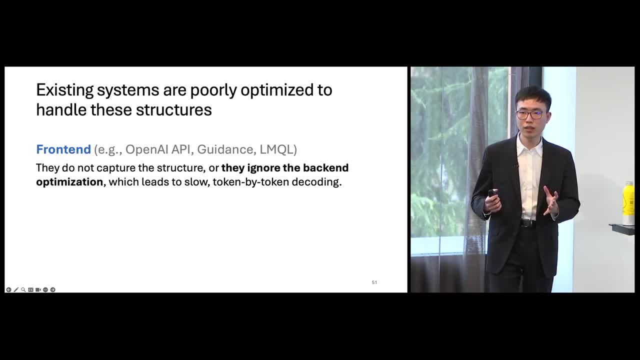 low-level API like OpenAI APIs, but they are too low level so they do not capture the structure information, although we try to build a better programming interface for large-ranged models, but they just totally ignore the back-end organizations. they cannot handle the parallelism and batching. 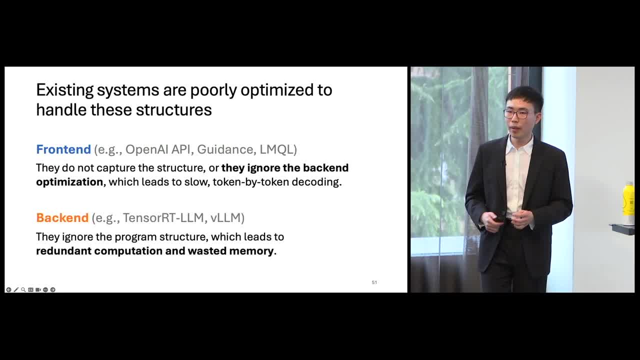 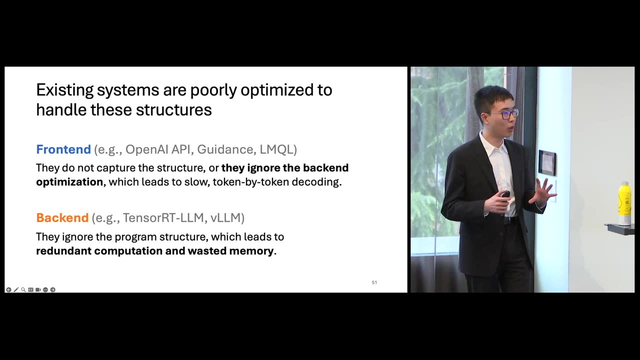 correctly, leading to slow token-by-token decoding. and on the back-end side, although there are some high-performance inference systems like tensile, TLM and VLM- I also built some of them- but they largely ignore single codes when we run this multi-code pipeline through these systems. 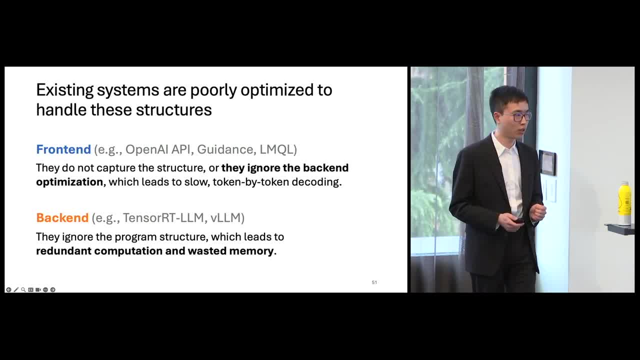 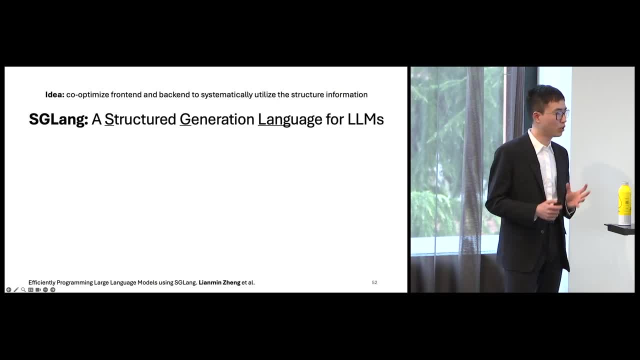 it often leads to redundant computation and wasted memory usage. so in this project our goal is to tackle this problem by co-operating both the front-end and the back-end to systematically utilize the structure information. so we proposed SGLang, a structured generation language for large-ranged models. 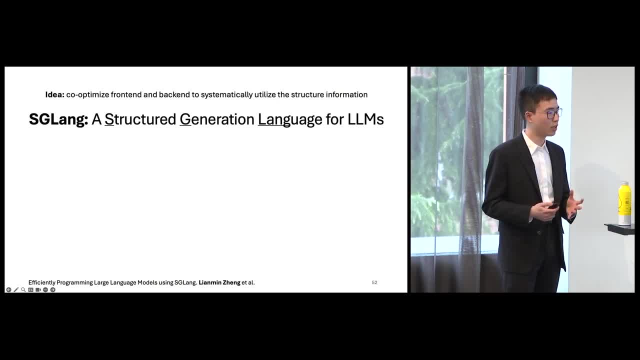 as the idea is to build something like SQL for large-ranged models. so on the front-end side we developed a domain-specific language. it provides some simple primitives for users to easily write their complex prompting workflow. so they can write their prompting technique with some structure information. 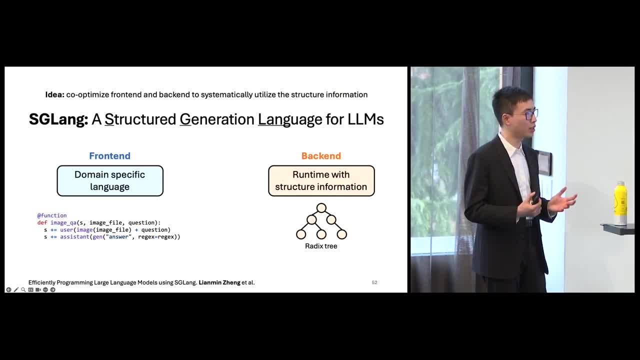 and additional constraint information. moving to the back-end side, to accelerate the inference and control the inference, and in the middle, the SGLang programs can be executed either using an interpreter or compiler. by using such a coding approach, we can think the problem from a global perspective. 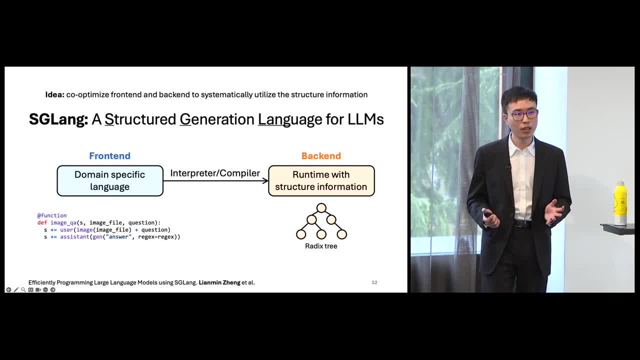 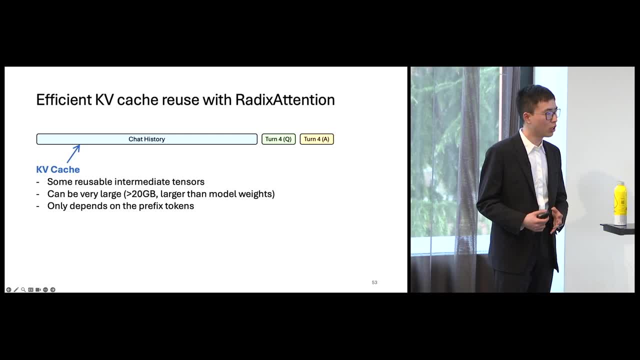 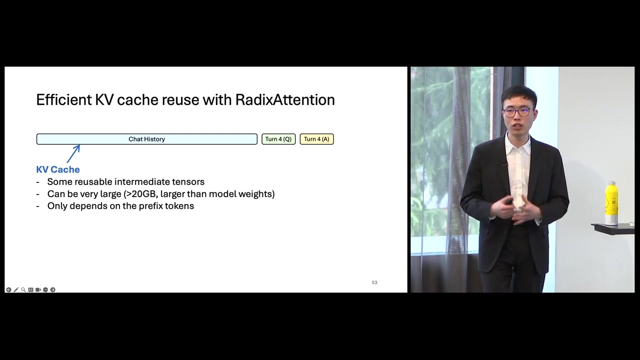 and propose some new compiler and runtime organizations. given the time constraint, I will only focus on one back-end organization, so let's move on to the next topic. the next topic. I will focus on the concept of KVCache. in the previous slides, I have briefly mentioned the 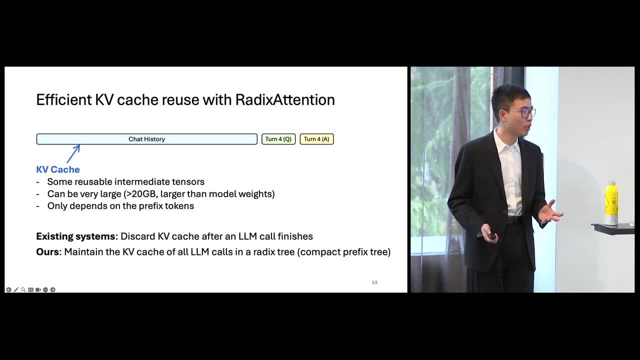 concept of KVCache in the previous slides. the concept of KVCache in the previous slides is the concept of KVCache for single LLM codes, so they will simply discard the KVCache after a request is finished. but in our project our goal is to optimize multi-code. 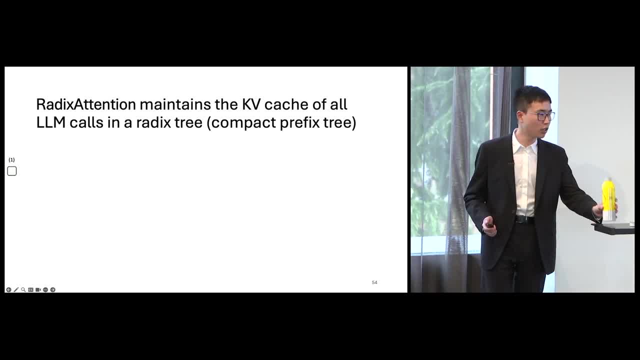 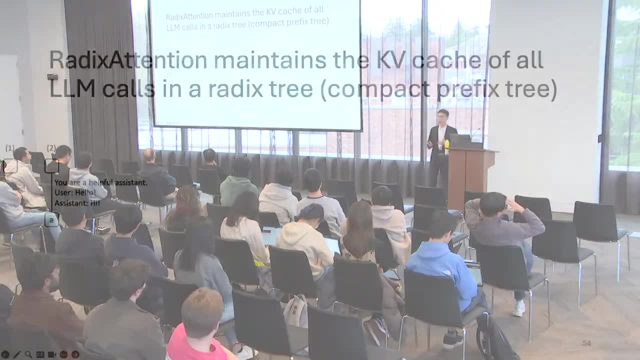 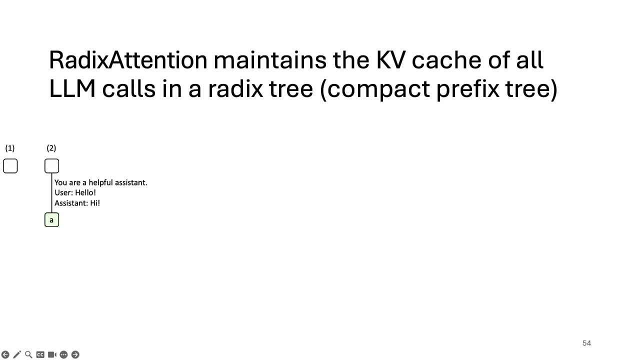 and maintain the tree. initially the tree starts off empty. in the next step the server receives an incoming user message, hello, and a response with an LLM output high, and then we concatenate the system prompt- you are a helpful system- and user message and LLM reply. we will label. 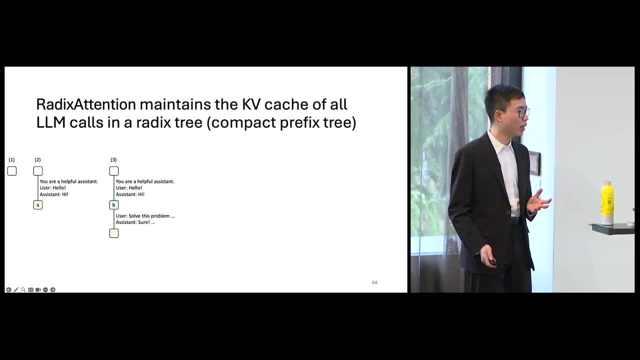 each edge with a string which is just a sequence of tokens. in the next step, the chat session continues, so the server receives a new message and it can run a prefix matching and identify. the prefix of the prompt is already in the tree, so if you distinguish different, 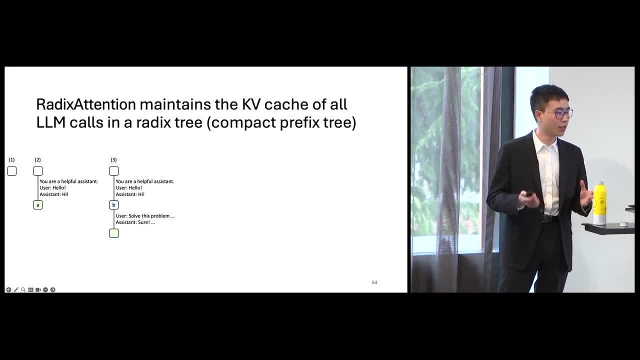 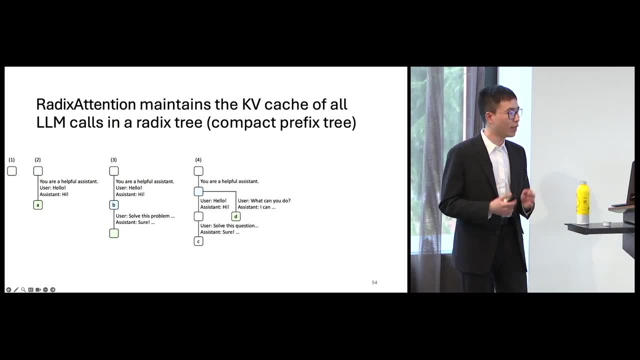 states the green for catch nodes that have been accessed and, sorry, the green for newly added nodes and the blue for catch nodes that have been accessed. in the next step maybe a new user come in and a new chat session begins. and in the last step, the second. 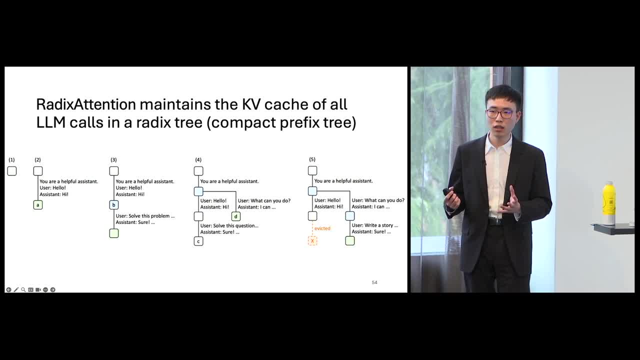 chat session continues. in this case, we may encounter the GPU memory limitation, so we have to evict some nodes. so we also designed an LRU eviction policy to recursively evict the leaf nodes. okay, you may think that the tree can be trivial, because there are many. 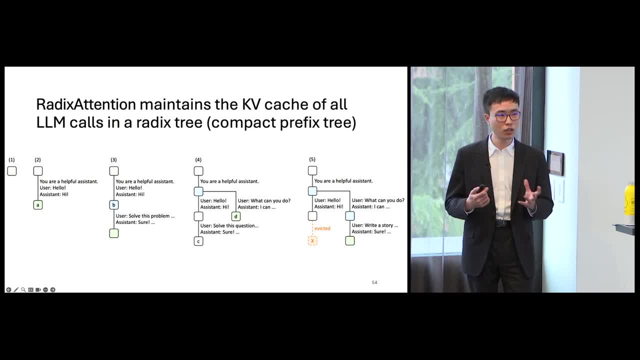 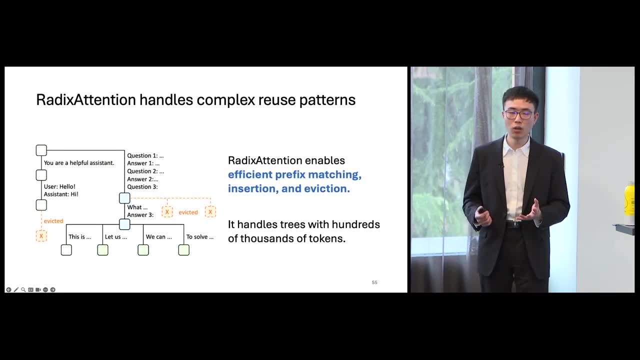 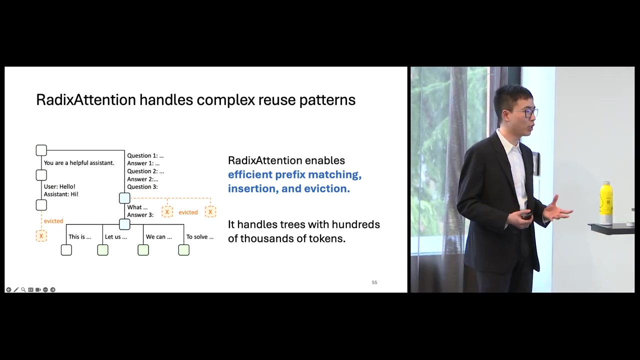 opportunities across different conversations. but this technique really shines for more advanced use cases, such as the tree search I mentioned earlier and some offline batch processing jobs. so here I will show you a more complicated pattern so you can see that in practice we can handle a tree with. 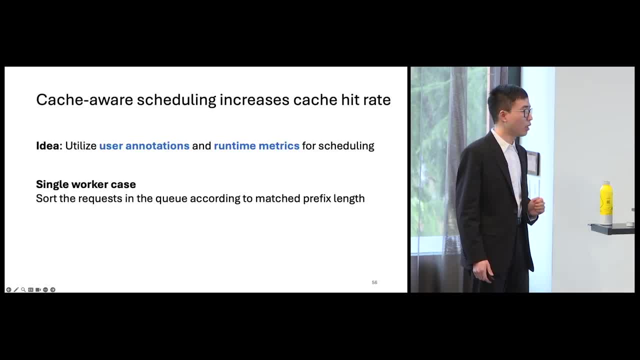 hundreds of thousands of nodes with very low overhead and high cache hit rate and to fully leverage the cache in the reading intention we also propose some cache aware scheduling so that we can prioritize the request in the waiting queue according to their matched prefix length. so we can 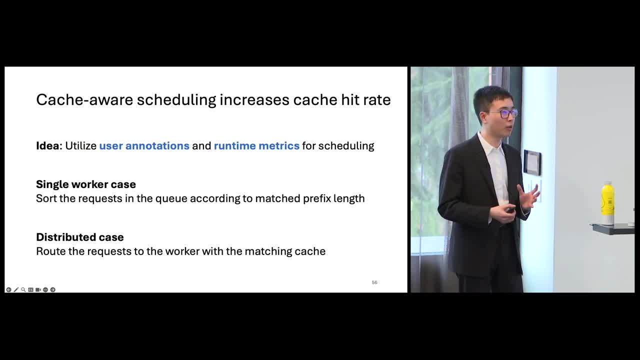 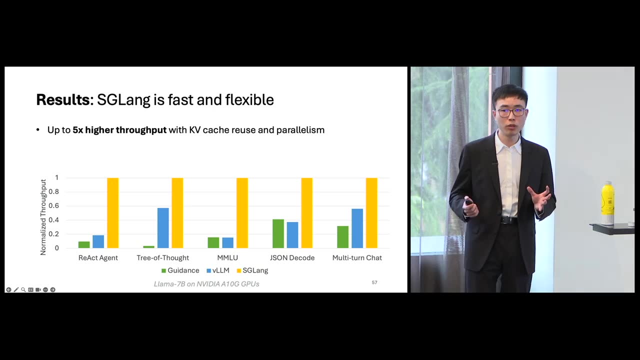 prioritize the request with longer matched prefix and in a distributed setting. we implement a router that's capable of dispatching the request to the worker with the matching cache and we have a policy that can balance the workload and the cache. so with these applications we can achieve. 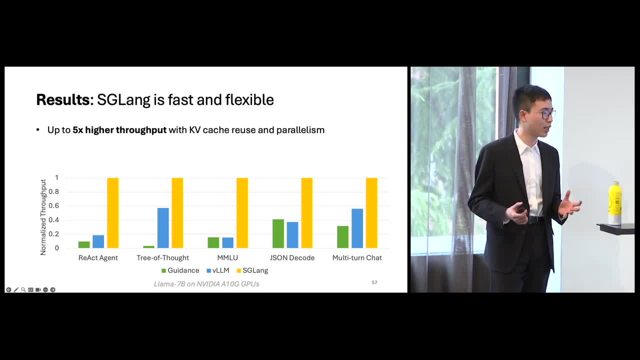 improvement of 5x higher throughput compared to existing systems like VLM and Guidance and, as shown in this figure, the improvements spans a broader range of LLM workloads, including agents, reasoning tasks to reduce the KV cache and the parallelism within a single program. and 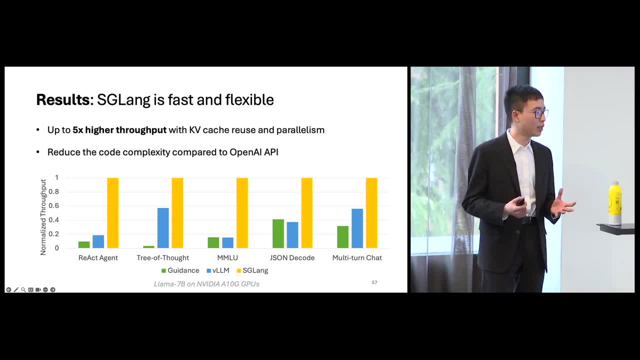 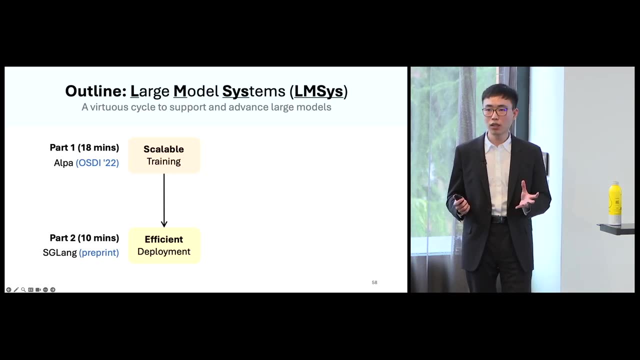 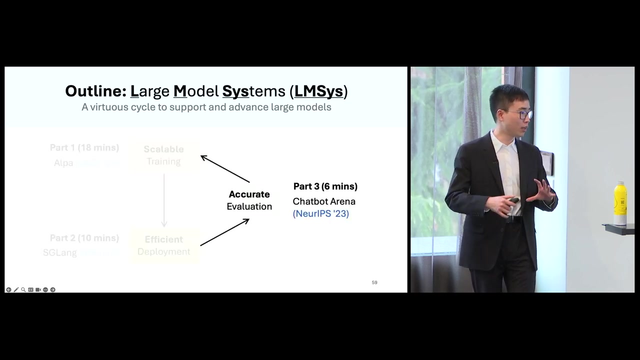 by using SG-LAN, it can also reduce the code complexity and simplify your code compared to OpenAI APIs. this is still an ongoing project and I will share more future directions at the end of this talk. great, so this concludes our talk. next, I will introduce like: 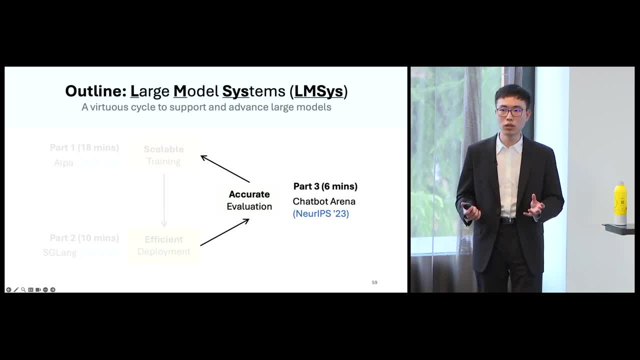 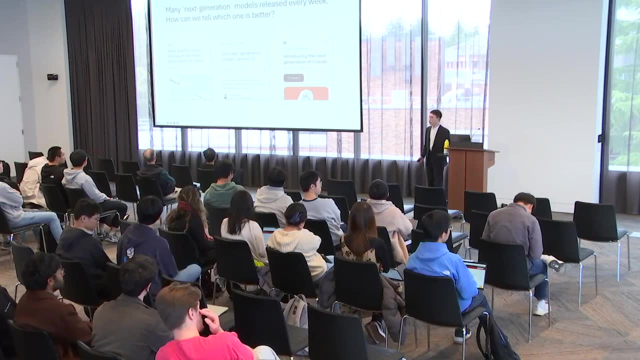 the last remaining component in this life cycle is evaluation, so I will briefly introduce our model evaluation efforts, including the tribal arena and LLM. as a judge, these tools can help us accurately evaluate a model and help us with building the next generation models. so if you follow, 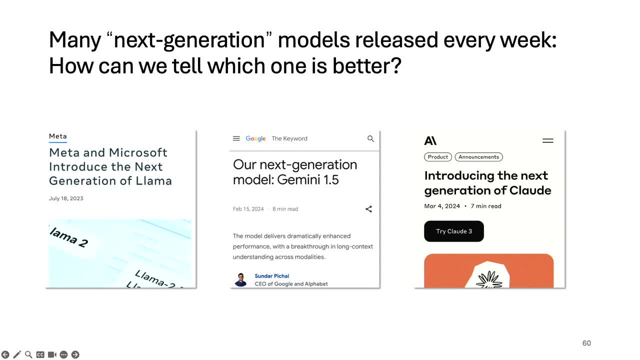 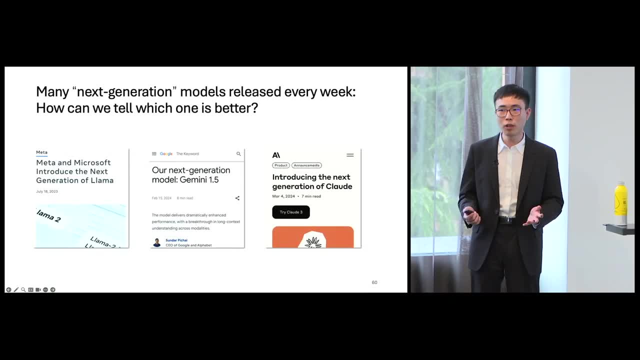 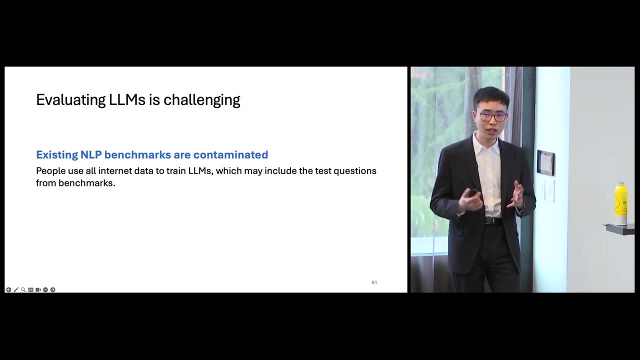 AI news recently, they all claiming their model is the best. with so many models being released every week, how can you tell which model is better? it turns out this problem is very challenging and our existing model evaluation methods are not sufficient. so why is evaluating the quality of 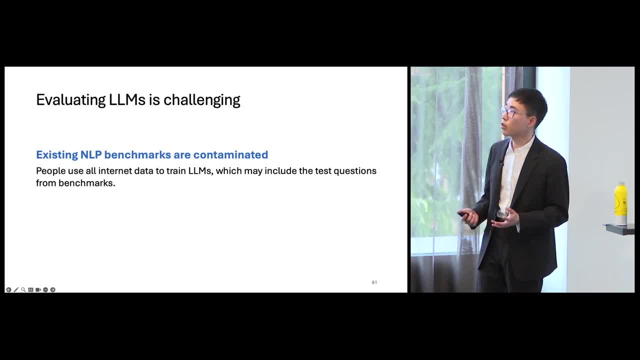 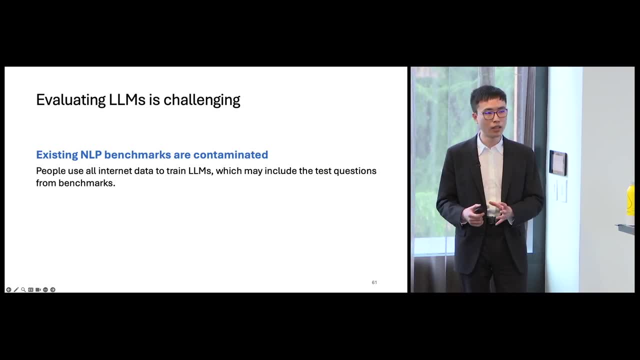 LLM challenging. here are two major reasons. the first one, like people currently typically report some accuracy of their models on some standard NLP benchmarks. however, for most NLP benchmarks the test questions are public and fixed, so over time these test questions can be included in the training set. 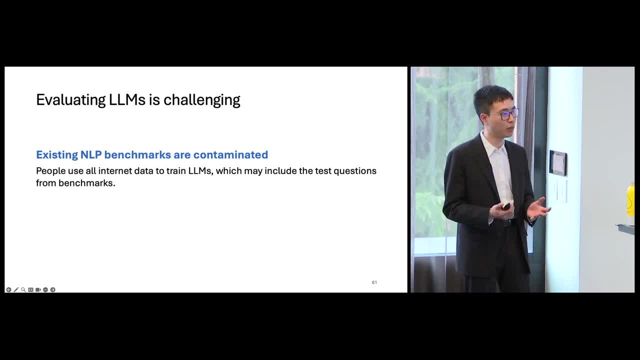 leading to a problem we call data contamination and making the benchmark result unreliable. so people can do this intentionally, just for treating, or they can do it unintentionally, because they just crawl the whole internet data for training. and the second problem is models are now much more powerful. 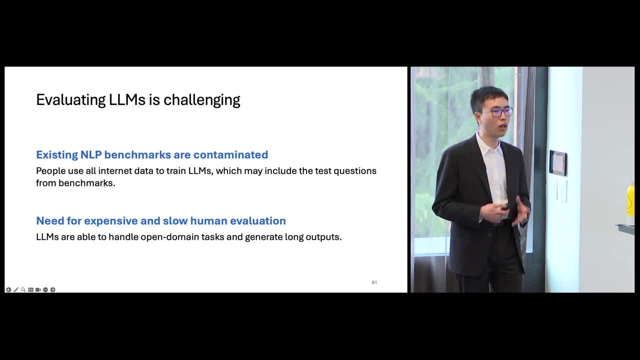 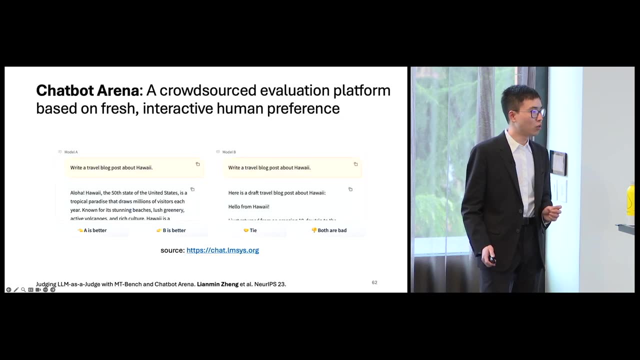 so they can handle many tasks and generate long output in this. this complexity makes it very challenging to develop automated programs for output evaluation. we often have to resort to expensive and slow human evaluation. so to address these problems, here is our approach. first, we introduced the chatbot arena. 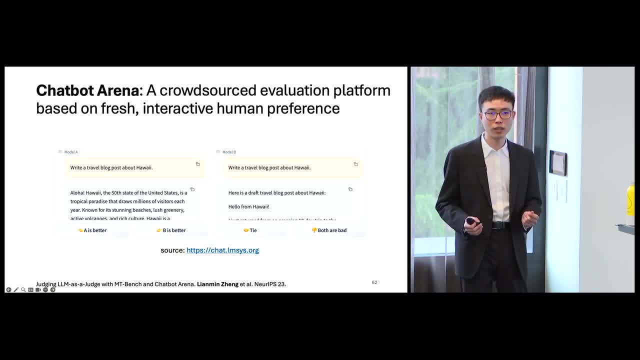 it's a crowdsourced evaluation platform for evaluating large-language models based on human preference. here you can go to the platform and you can go to the url. right now it's a free platform where anyone can go to the platform and chat with two anonymous, anonymous models. 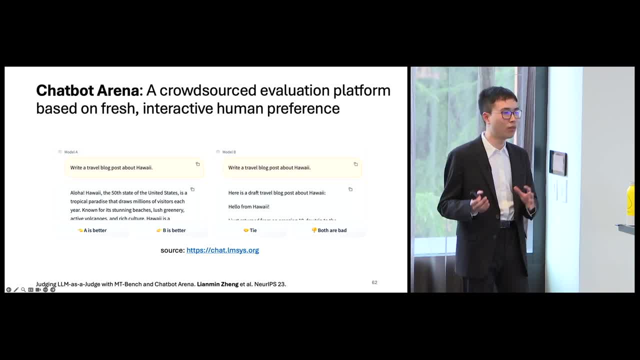 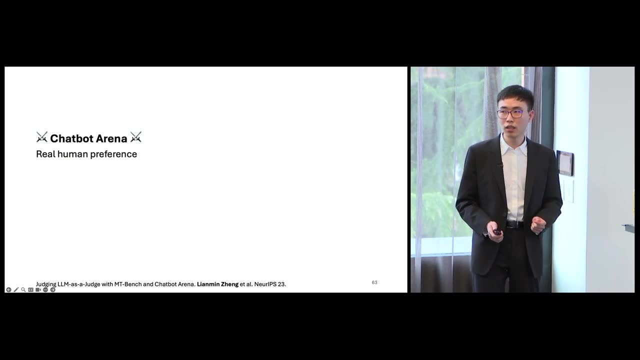 side by side. you can bring any challenging and interesting new questions you have and then vote for your preferred answer. the idea here is to collect fresh, diverse human feedback from crowdsourcing, and while human preference is a gold standard to obtain, so we also explored whether we can. 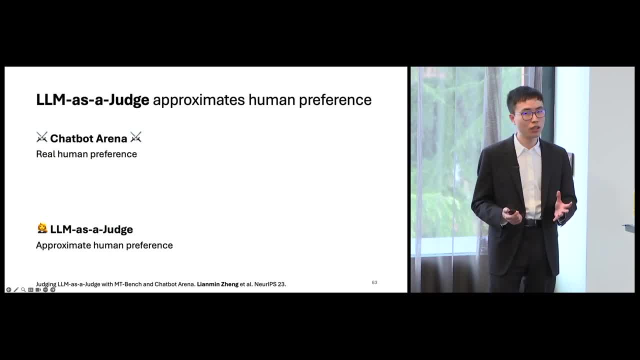 quickly approximate human preference by using an lm as a judge. the idea here is to prompt a strong lm such as gpt4 to act as a judge and evaluate the quality of other models output. by building these two platforms, we can actually do cross validation across them. 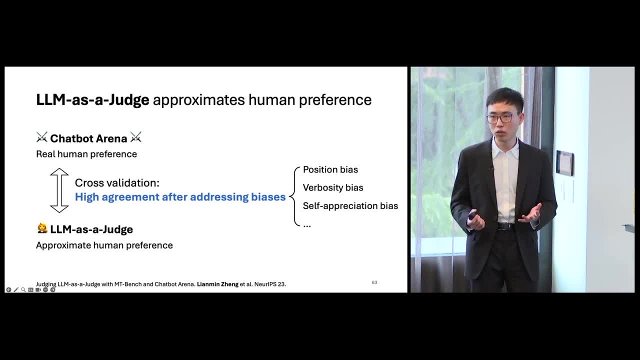 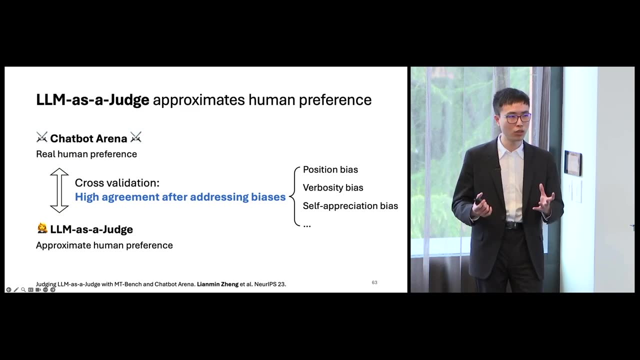 so initially we find the gpt4 judge is not that good due to some interesting biases in these models, for example the position bias, where they always favor the answer in the first position and we apply some prompting techniques to mitigate them. after that we find the agreement. 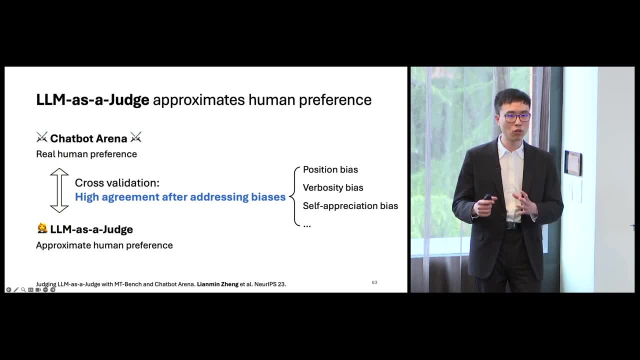 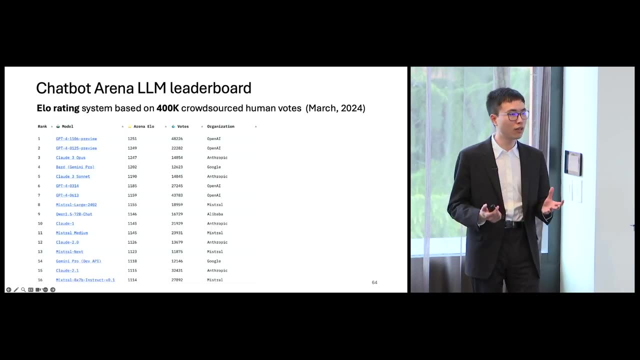 between crowdsourced human judges and gpt4 judge is actually pretty high, as high as the agreement among humans themselves. so this means we can actually utilize gpt4 as a judge in some cases and we have been running the crowdsource platform for a very large user base. 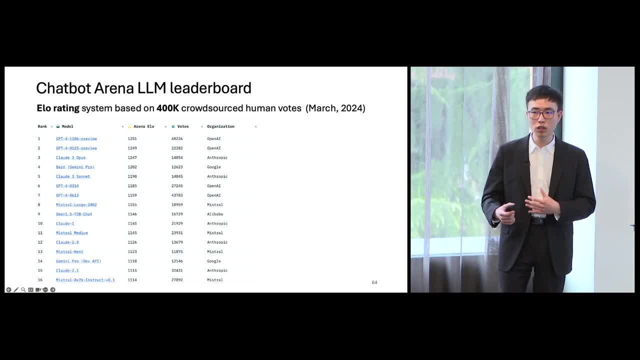 and we utilize these votes to compare a leaderboard of more than 70 models based on the ELO rating system. as you can see in the leaderboard, models from OpenAI, Google and Anthopic are ranked on the top and then followed by some open source models. most people 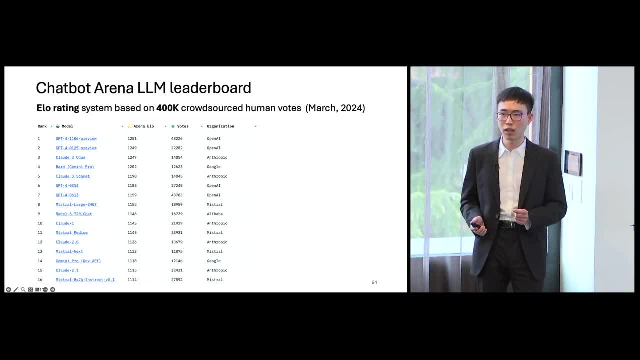 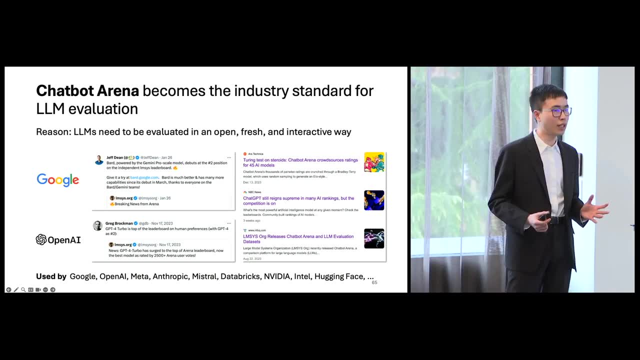 find this leaderboard can accurately reflect their own experience. it's unique value and openness. chatbot arena has almost become the industry standard for evaluating large-language models, because we just need such an open, fresh and interactive way of evaluating models. so now over 1 million crowdsourced. 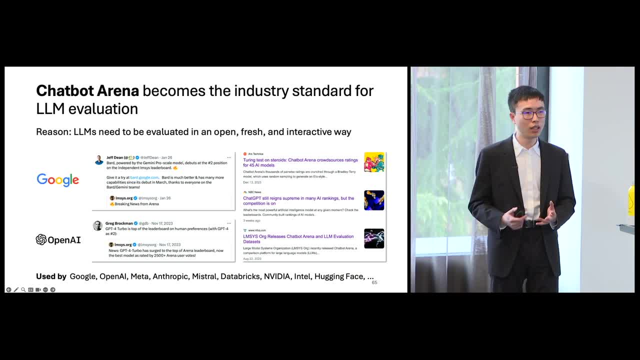 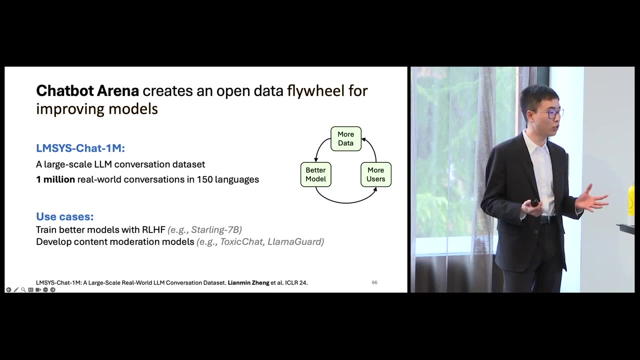 users have used the platform and it has been quoted and featured by major ALM companies and media outlets. so we are collaborating with these companies and we don't stop here. so the data we collected is not just for evaluation, it's also about creating an open data. 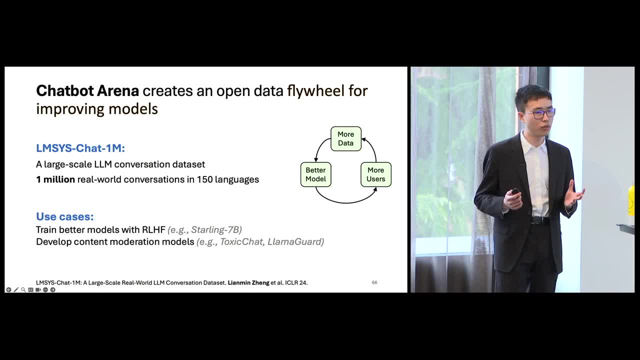 flywheel for improving the next generation open models. high quality data are very important for achieving good model quality. while large companies can easily get them, the open community often faces challenges, so chatbot arena is one of the most popular platform in the world, with over 1 million. 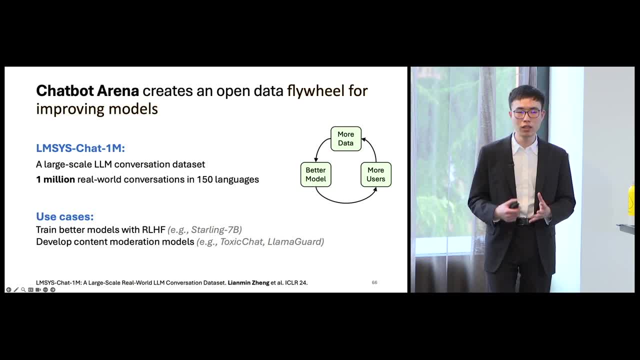 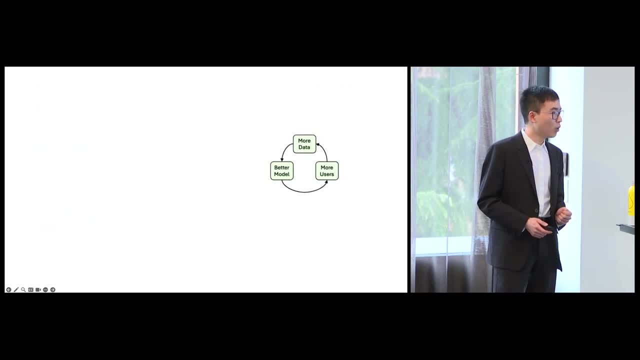 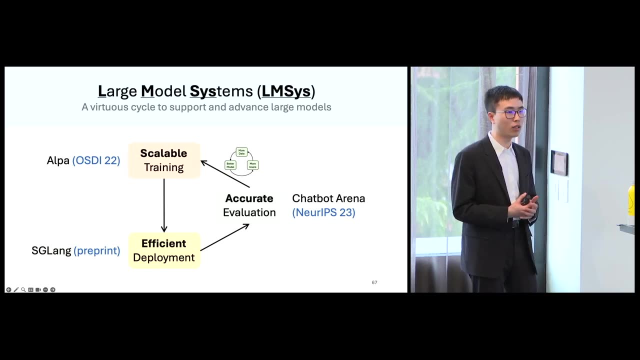 real-world conversations and people can already use it to do many interesting analysis and use cases. for example, people can change better models with IOHF and they can develop better content. so in this cycle I aim to continuously improve and improve open models. okay, so basically this talk. 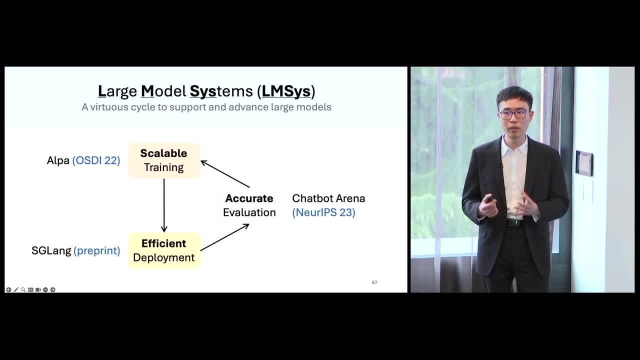 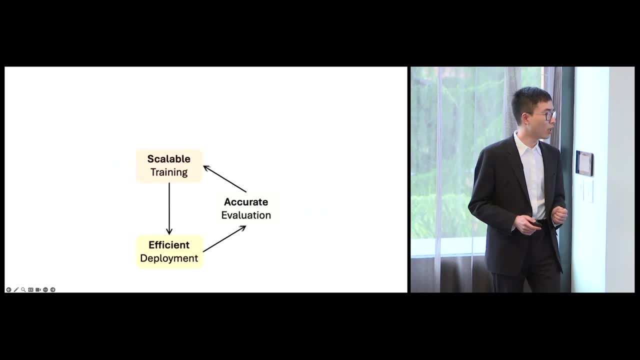 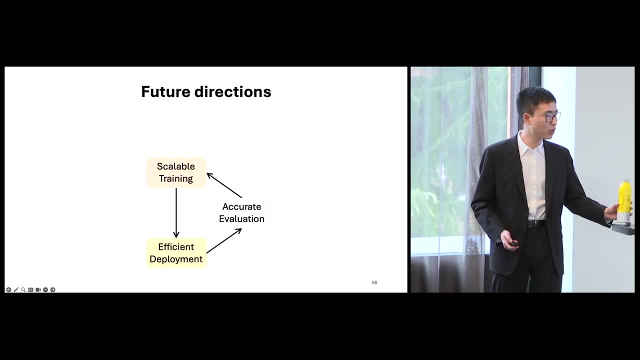 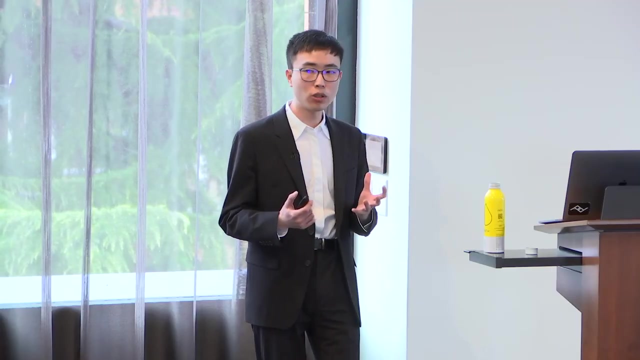 introduced three pillars of my research. I introduced alpha for automatic scalable training, SGLAN for efficient deployment and chatbot arena for accurate evaluation before the end of this talk. so on the training side, I believe we are gradually facing bottlenecks, not only in computer, but also in 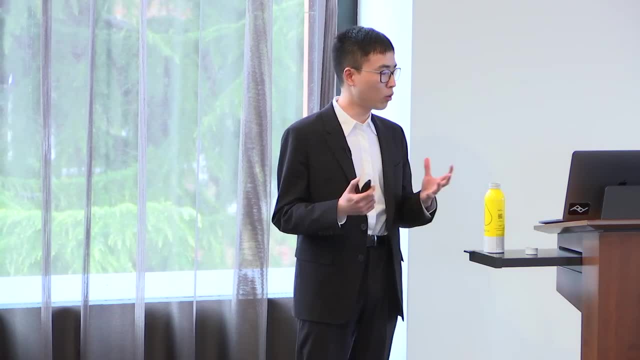 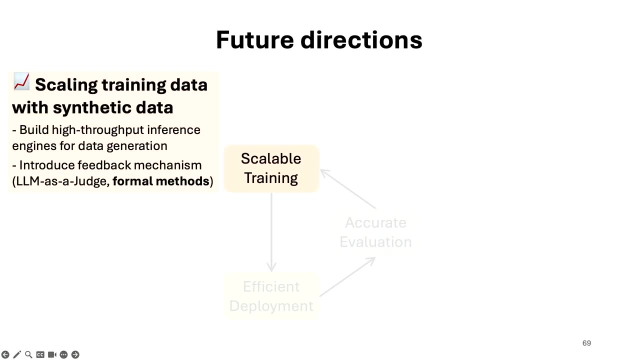 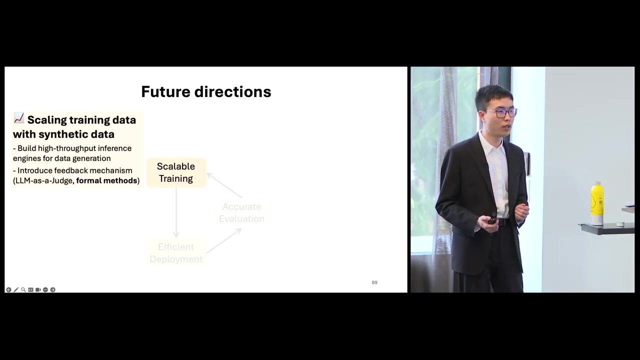 data, so probably there is a. we may quickly run out of all human generated attack data for training, so if we want to continue to scale, we need to think about other creative ways to get more data. so one promising direction is to use some advanced technique introduced in this. 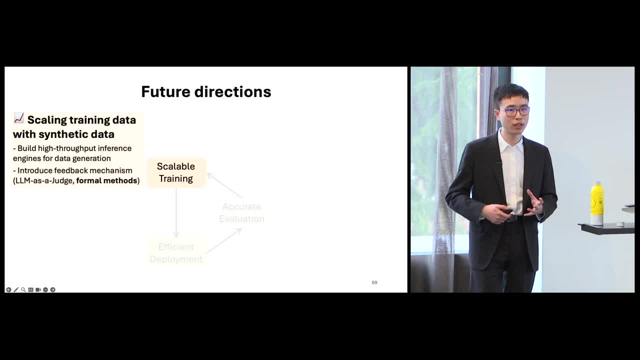 talk to help this direction. for example, in the future probably inference can take more time than training, because we have to run inference many, many times to just generate one good training example. so in this example we can use the data generation system. and then we also need to 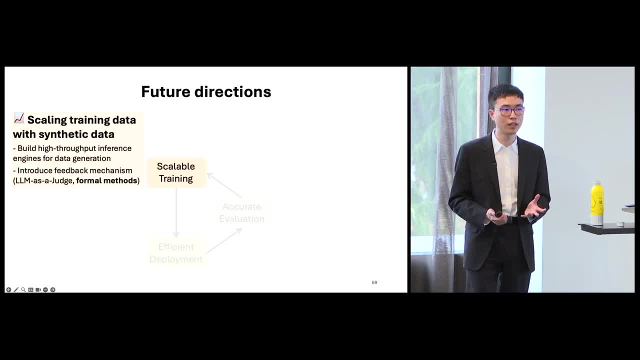 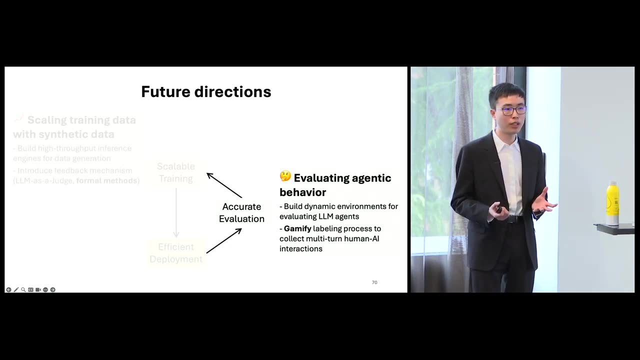 establish automatic feedback mechanism. for example, we can utilize LLM as a judge approach for some general settings, and then we then can also try some of these models as LLM agents in more dynamic and challenging settings. based on the concept of tradable arena, we can consider 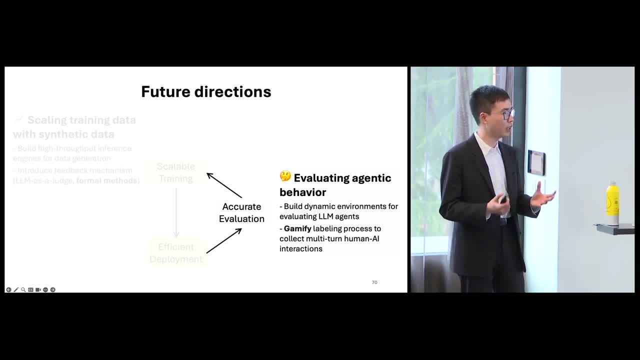 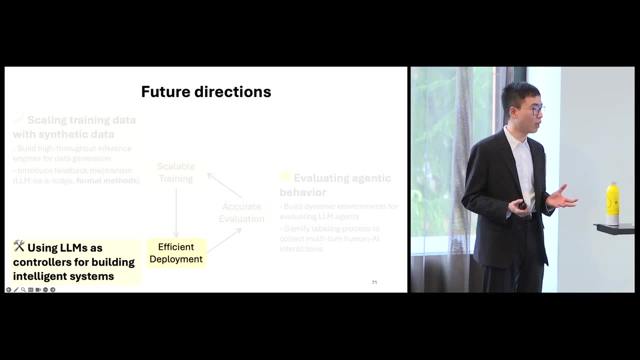 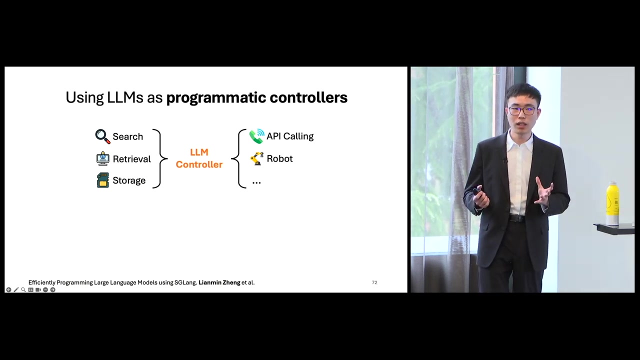 ways to gamify the labeling process, to encourage more deeper multi-turn- multi-turn interactions and feedback through deeper human AI collaborations and, lastly, in terms of LLM systems. this is the direction I'm mostly interested in, so I can go into further details. the motivation is that 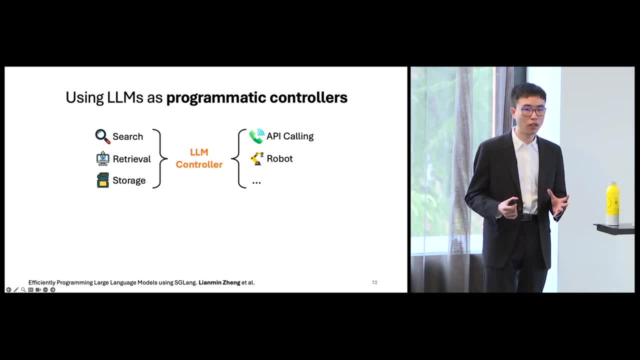 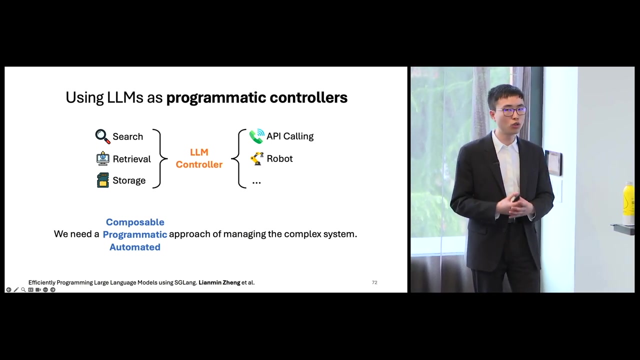 LLMs are now gradually becoming like, gradually evolving into a general purpose controller of a much broader ecosystem. the usage pattern shift from simple to complex systems. we need a composable programmatic and automated software stack, similar to how we build the operating system and programming system. 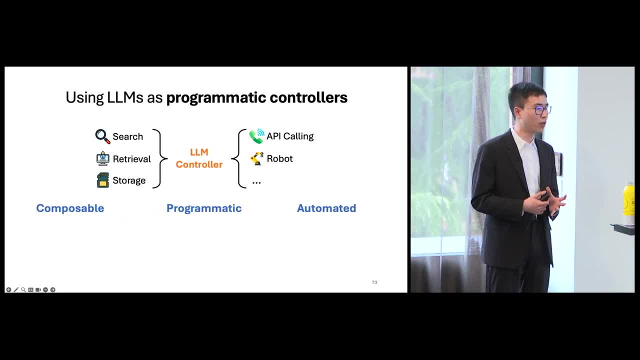 to manage and talk to the CPU. in the future I'm interested in extending beyond the SGLAN to provide such a programmatic way of using LLMs to make things more composable. I'm interested in a program code with like verification of type systems. 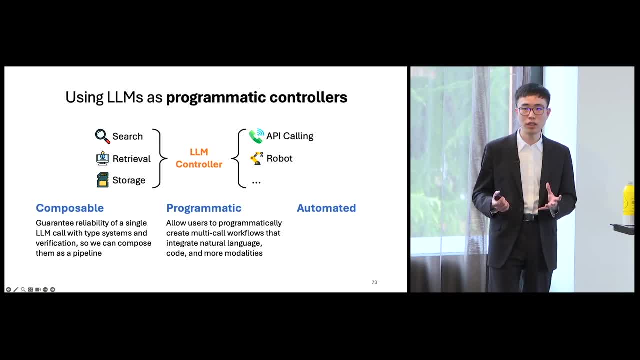 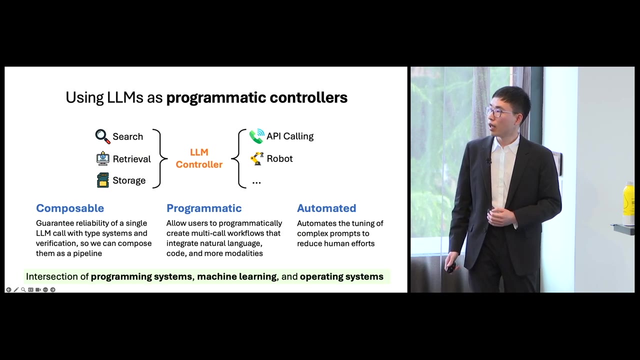 so we can ensure the reliability of a single code and compose them into a more robust pipeline. to make things more programmatic, I'm interested in developing a programming interface that can allow engineering so we can reduce the human efforts, and by pushing for these directions I aim to 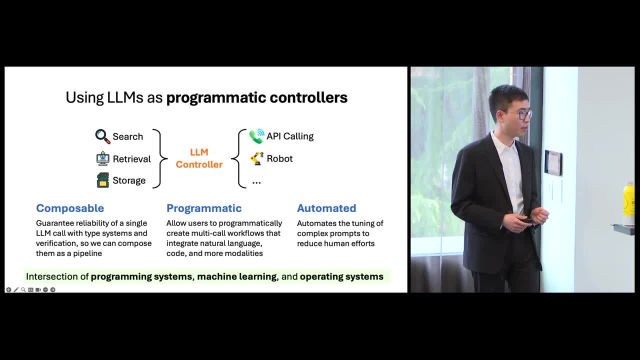 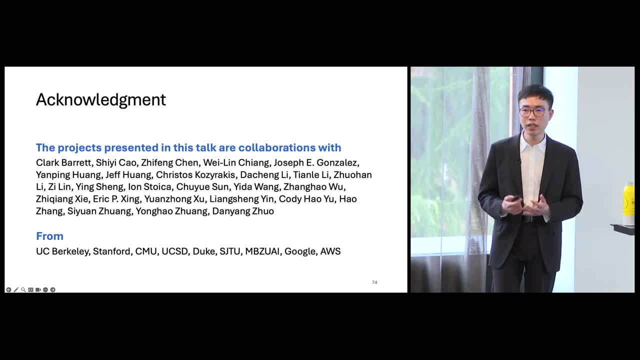 bring people from programming systems, machine learning and operating systems to all work on large model systems. and, lastly, I want to thank all my collaborators who made this talk possible. it has been an amazing experience working with- probably looking for some Udall people here, as they are. 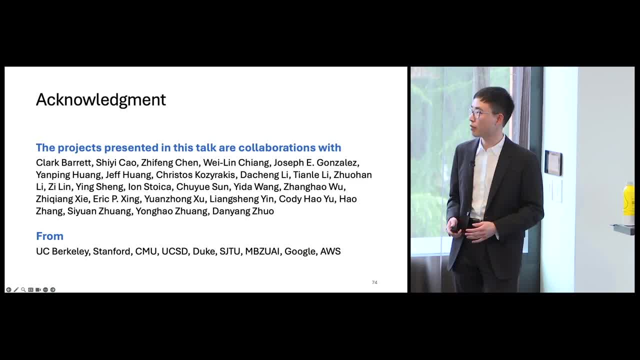 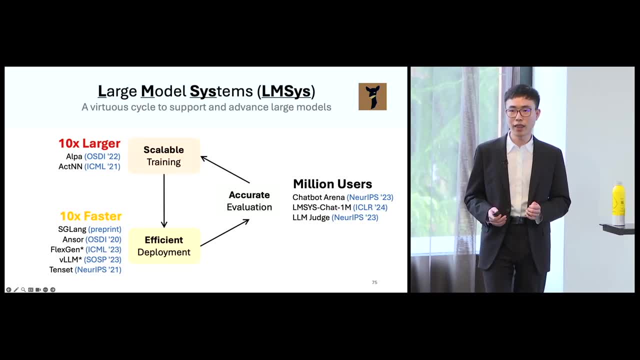 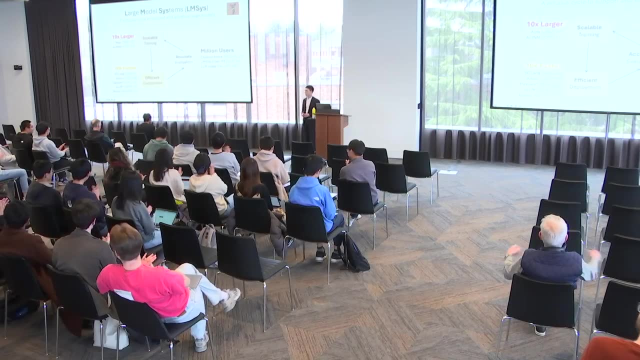 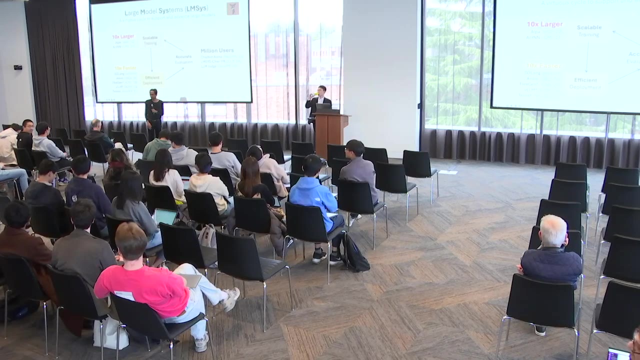 not listed here, but previously, when I was an undergraduate, I also actually collaborated with a lot of Udall faculty, so here, okay, so this is all about my talk on large model systems and thank you for listening, and I'm happy to take any questions you may have. 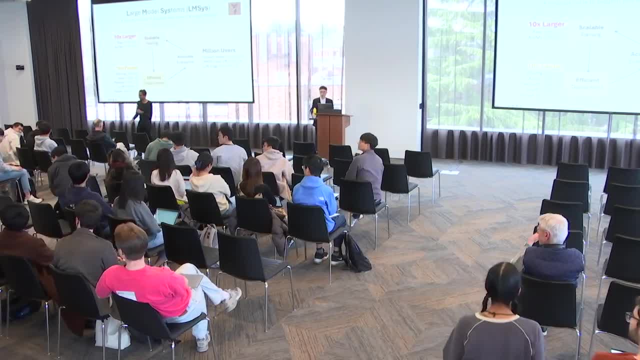 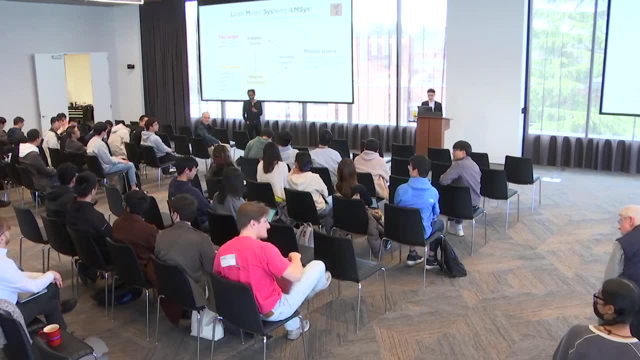 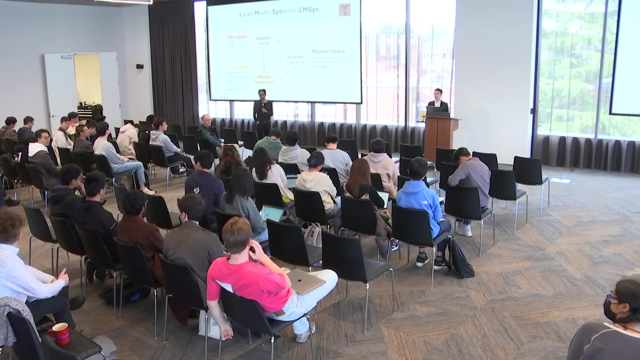 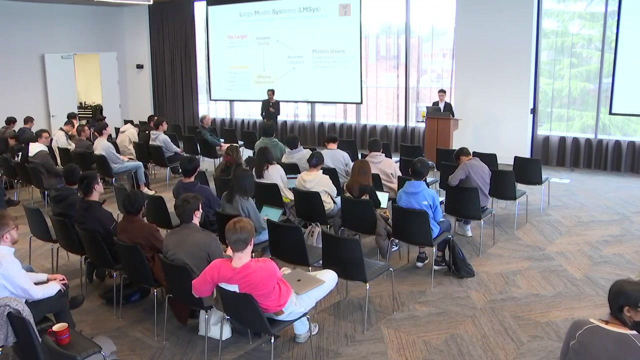 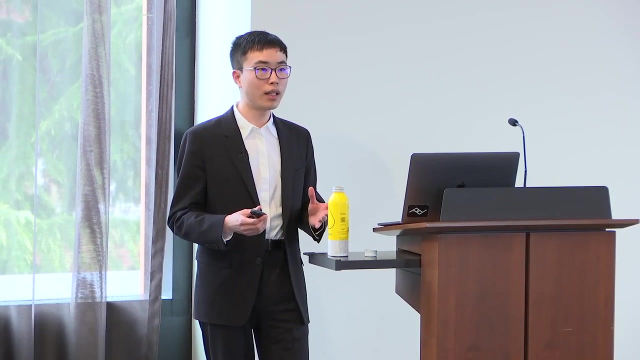 at me, just trying to understand the accurate evaluation piece. I think the general pipeline you are applying you know search companies have been using for a while, like Microsoft, Google and Baidu. is there something different about this? yeah, but then, like for large models, probably the different part is: 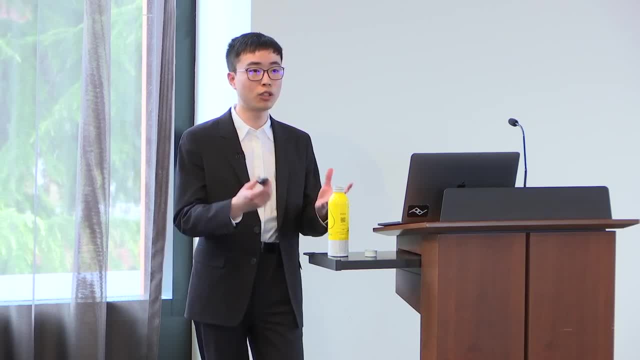 the model can now, I think, handle more tasks. yeah, they are more intelligent. for example, for search engine. you probably cannot ask a model to code or to like: do some like complicated reasoning? yeah, but I think models here are just more smart. so, when to better think of, 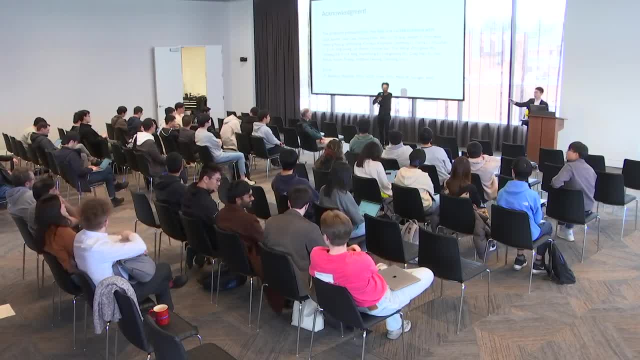 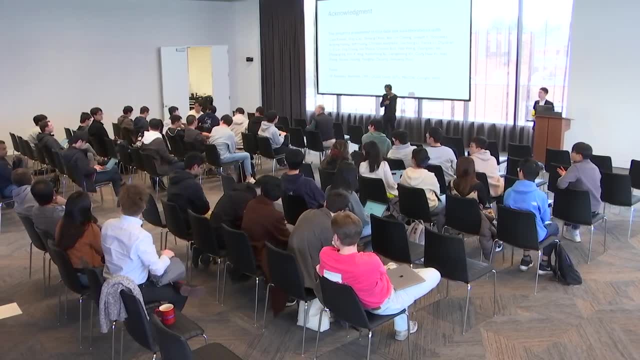 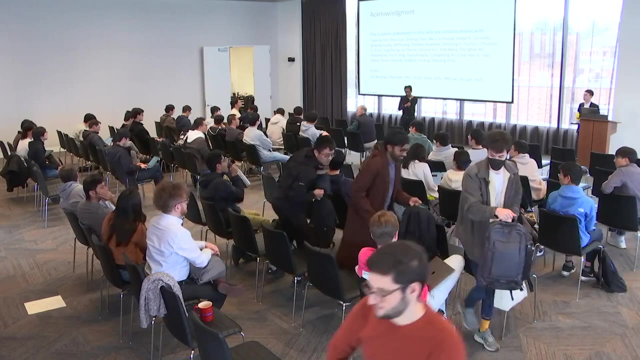 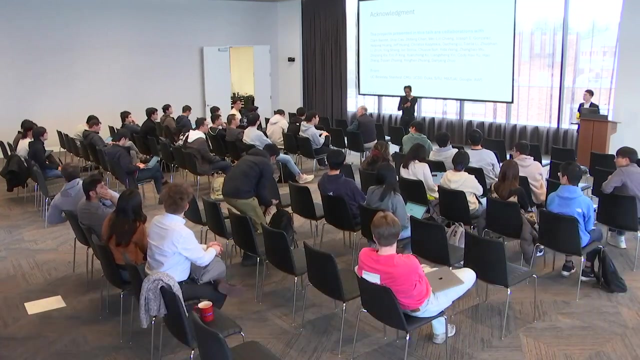 I'll probably he's earlier, so I wasn't sure what your model for when you were talking about the training systems with sort of public use of public software, whether you encountered any sort of privacy questions about the people who were using having the expectation that their conversations. 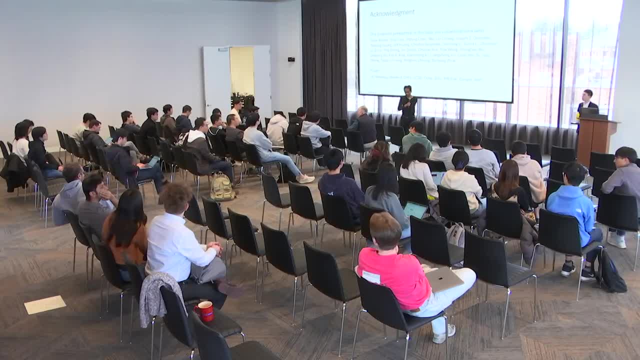 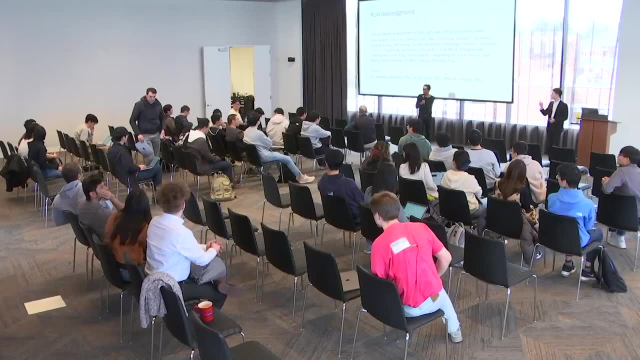 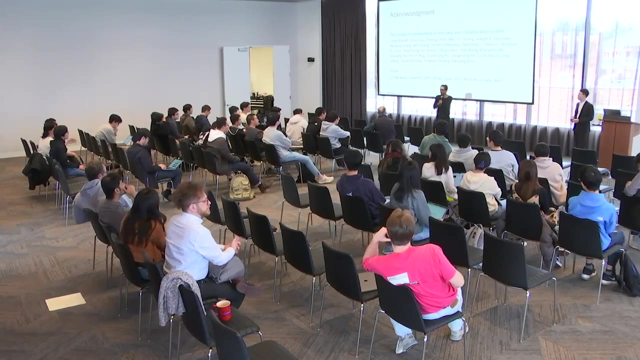 were not sort of widely shared, so I don't know if you can comment on that. okay, so sorry, I didn't hear it very clearly, could you? yeah, I don't know. yeah, I think Tom wanted to comment on privacy issues of users who are kind of using LMS. 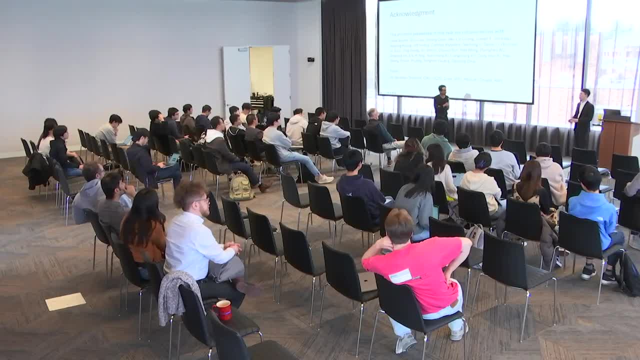 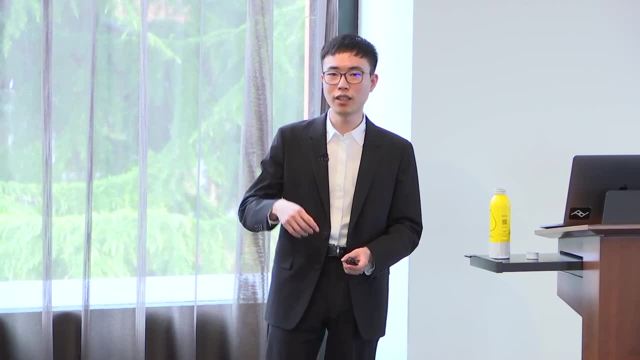 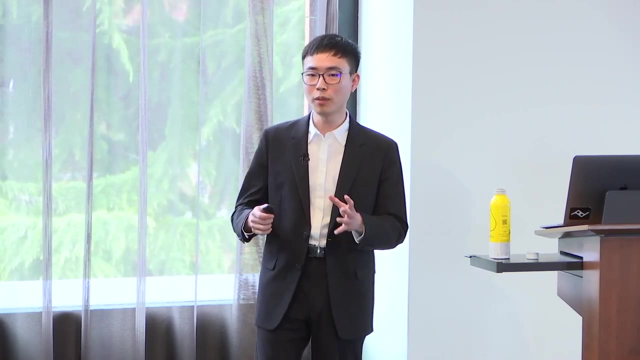 with or okay, yeah, we have an agreement in the very beginning, so they have to agree that their training data will be used for training and the only ones they click the agree button they can go to our platform, and a lot of people they, because they are interested. 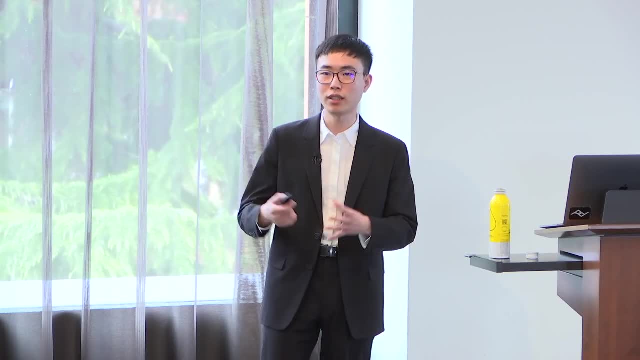 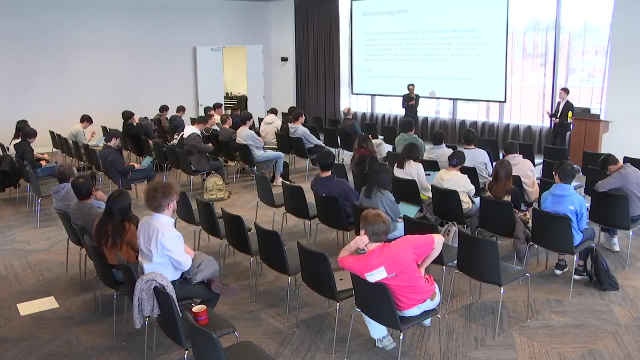 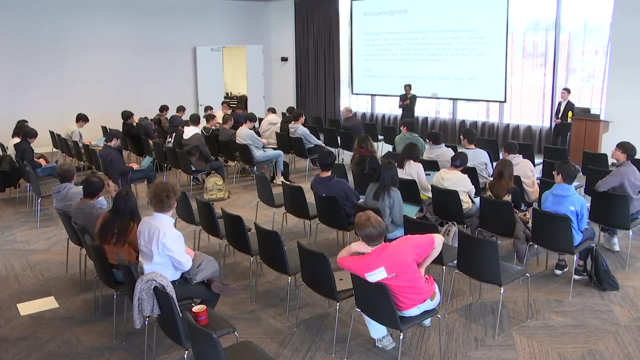 in contributing to this kind of effort and they are happy to share their data. yeah, so when they use this platform, they are aware that their data will be used for training? yeah, and we get the user consent. I think, Wei, you had a question. I guess one observation. 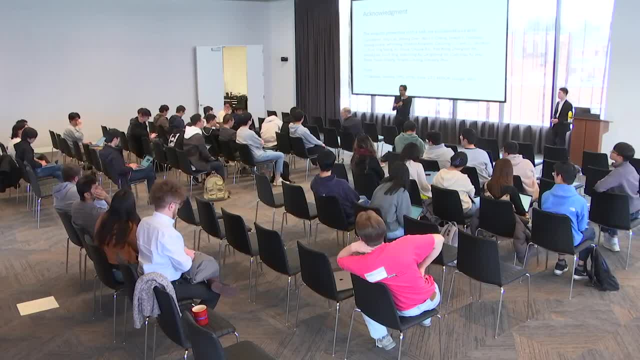 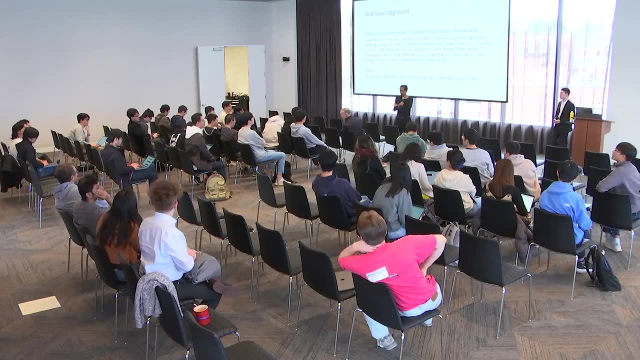 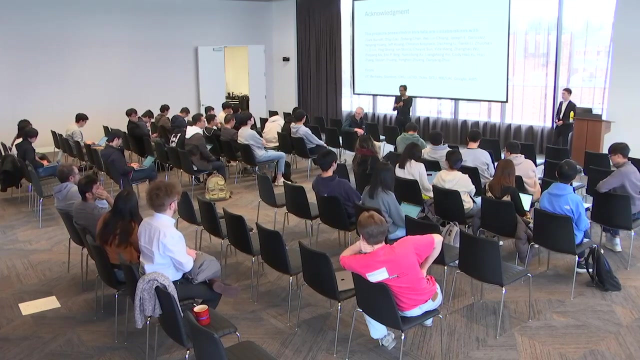 you had is inter-digit Xbox like connection is like slower than the MVLink, right yeah, but now I guess new you know hardware comes along and say they have the MVLink network for the new GPU cards, just, for instance. could you like even generalize this even more? 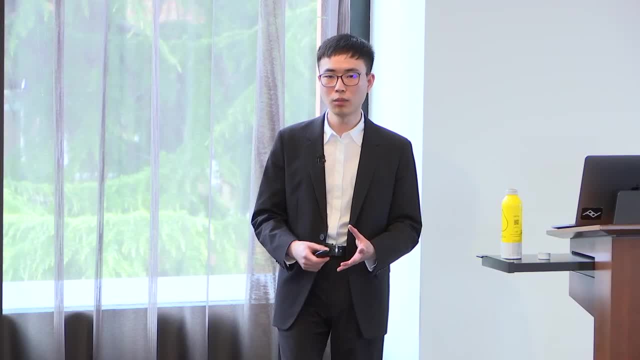 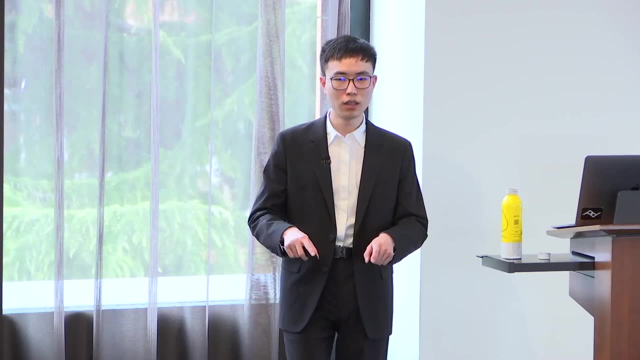 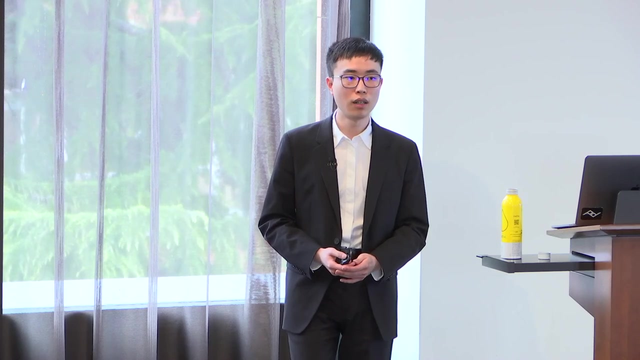 yeah, we can generalize this more, better models of device cluster. then you can generalize our model of the like the 2D dimensional mesh. you can generalize it to other network models and then, yeah, I think definitely like we only consider a simple, like two dimensional device mesh case. 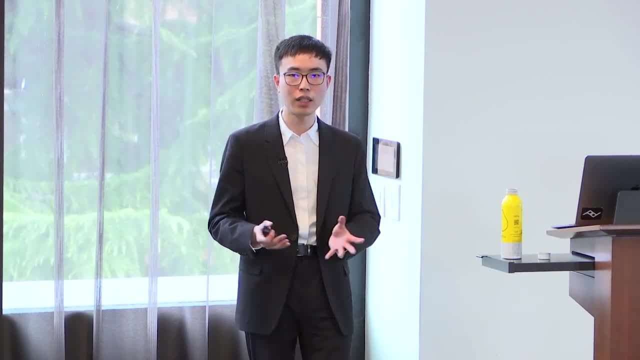 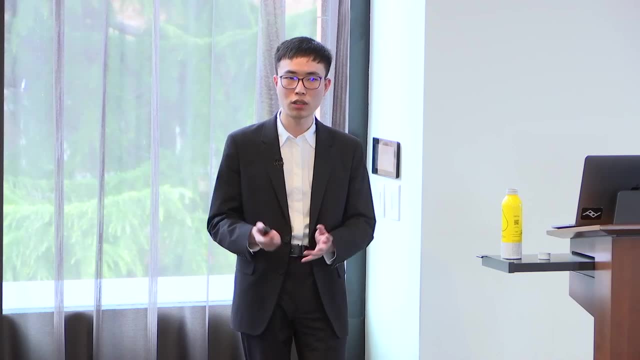 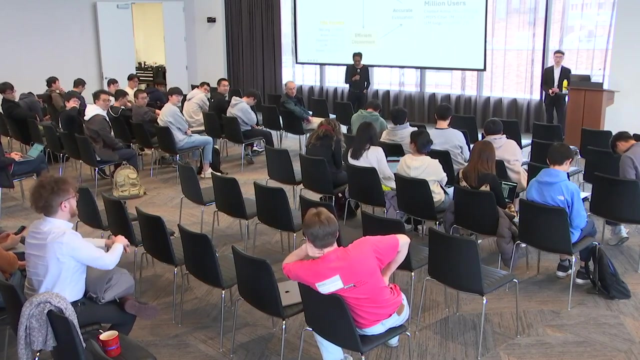 but then you can generalize it and I think our overall the architecture can still apply. probably you need to do some extension to handle newer or different like network topology. yeah, go ahead. thanks, the talk is really great. I heard a lot of parts of it in the the first. 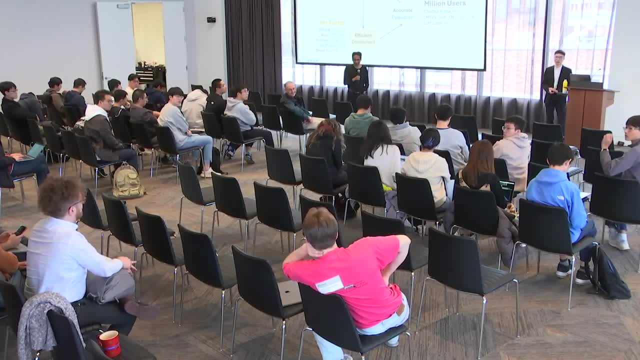 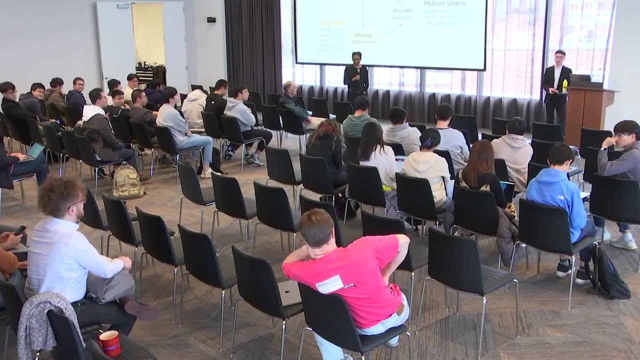 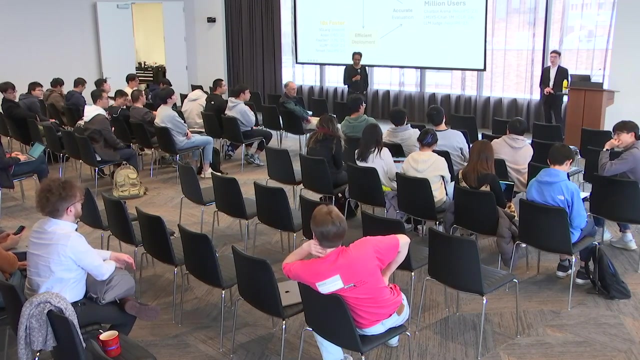 part of the talk. I'm wondering if I can needle you a bit on using linear programming to try to optimize within the GPU. or are you still using sort of a library of heavily tuned kernels running on the GPU, or are you trying to create those kernels? my sense is 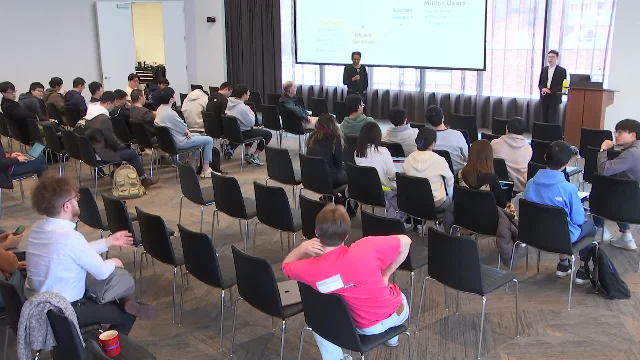 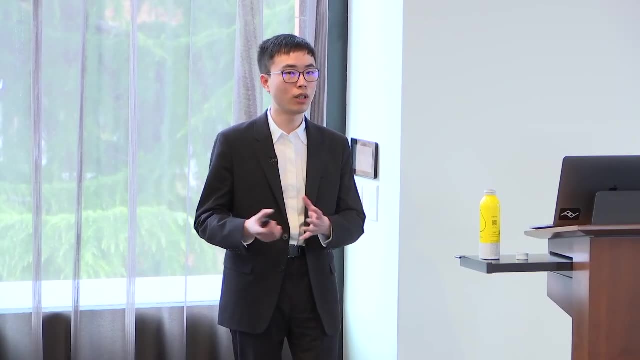 you're going to take some significant performance hit, even if it's only a small constant factor, on trying to use an auto tuned assembled kernel rather than something out of 3DN or Cutlass or whatever. okay, yeah, we directly call Cutlass these libraries. yeah, and we. 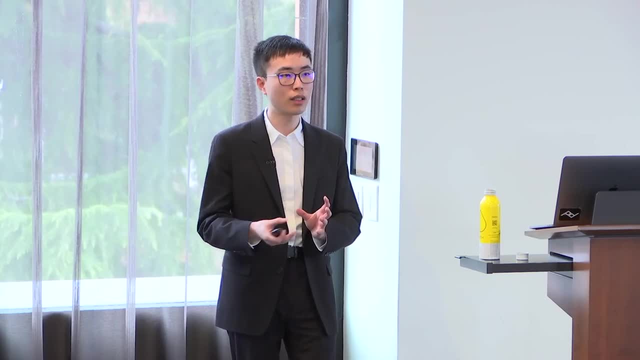 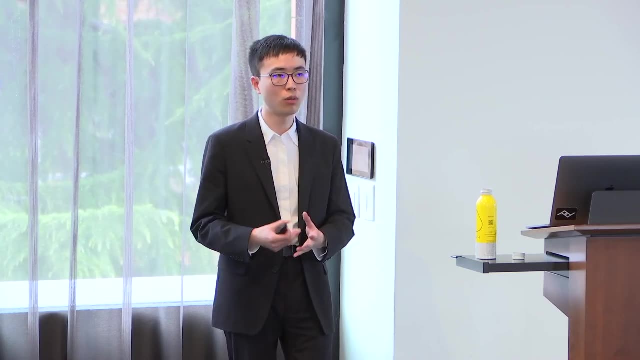 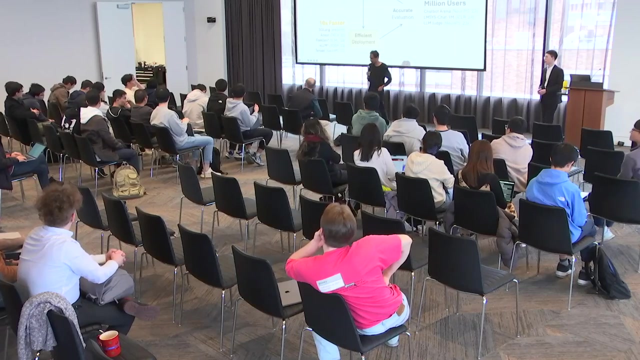 because this project is done in the XLA compiler, so we only inject our parts into a compiler and then the later parts. XLA compiler will mostly call Cutlass for doing matrix verification and then it will try to generate some fused kernel for like for element and that's.